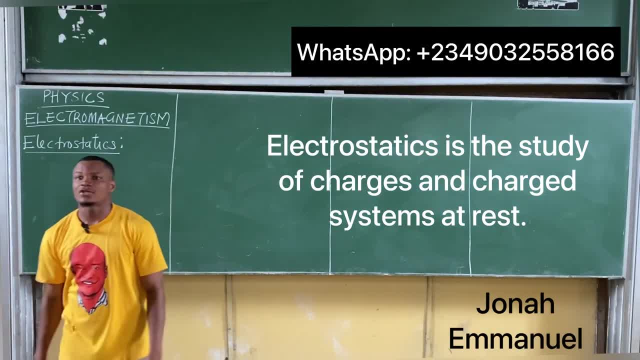 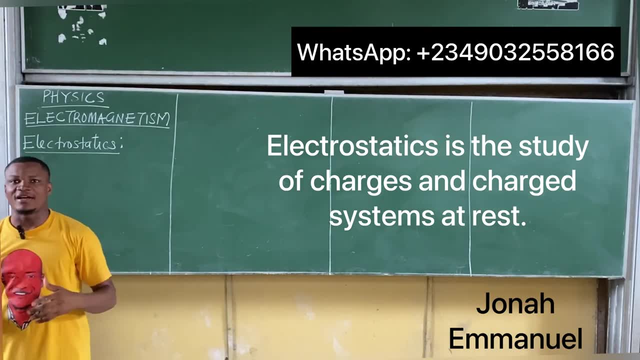 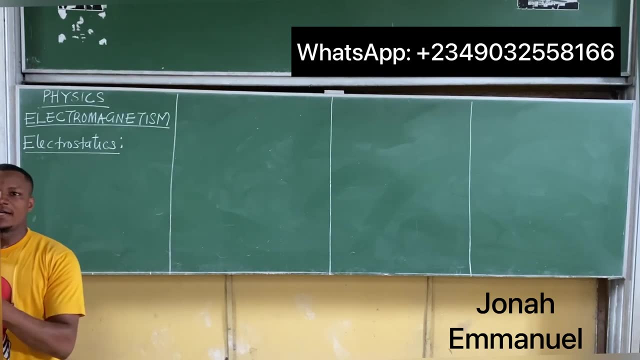 Electrostatics is the study of charges and charge systems at rest. Study of charges and charge systems at rest, Of course electro talks about electrons, or perhaps charges, and then statics talks about no movement at rest. If you combine them, it becomes electro, that's charges, and statics, that's rest. 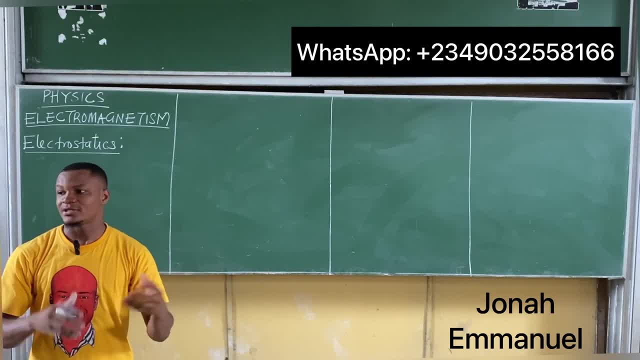 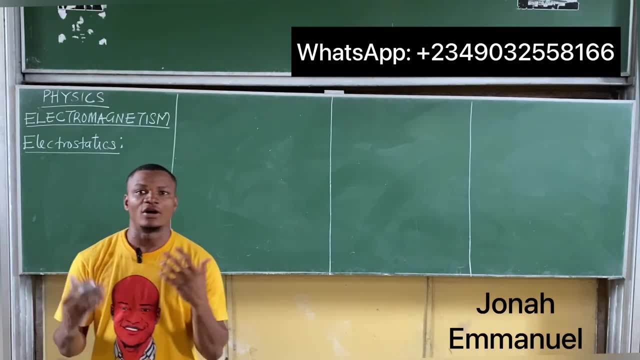 So combine them, because what they're? The study of what Charges and what Charge systems at rest, That's all. Take a paragraph. There are two laws of electrostatics. Take a paragraph, please. There are two laws of. 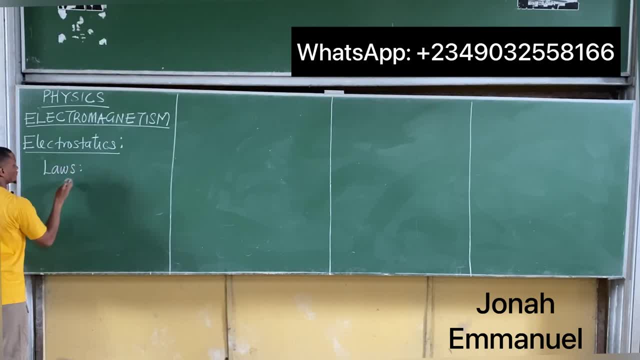 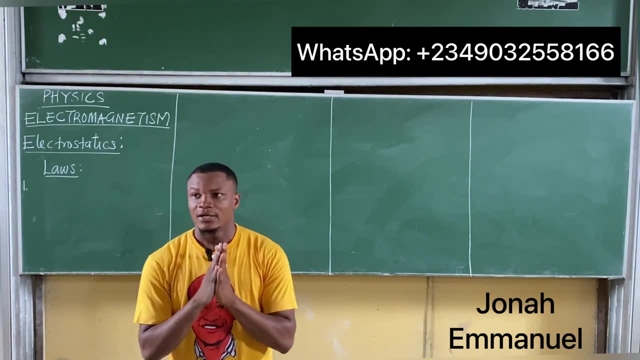 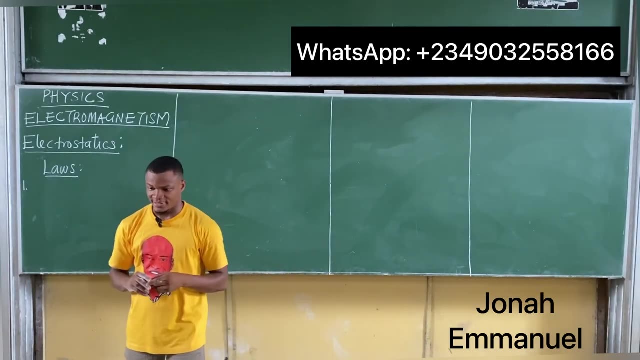 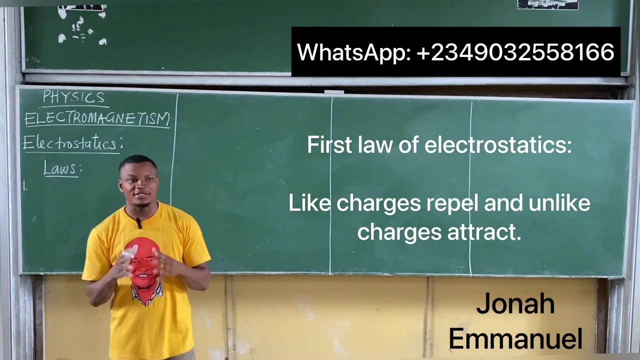 There are two laws of electrostatics. There are two laws of electrostatics, Law one: there are two laws of electrostatics, Law one: light charges repel and light charges attract. Of course you should know this one before now. 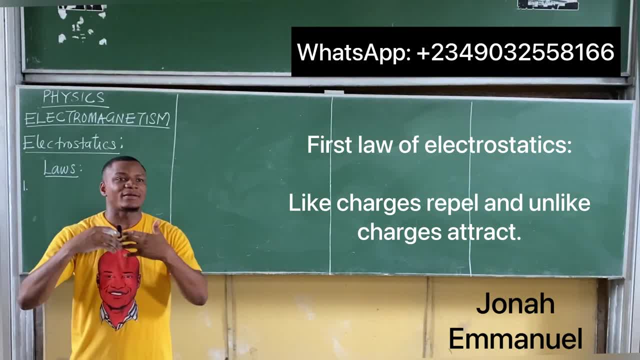 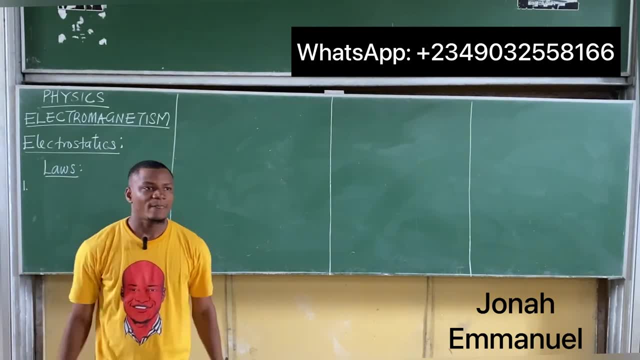 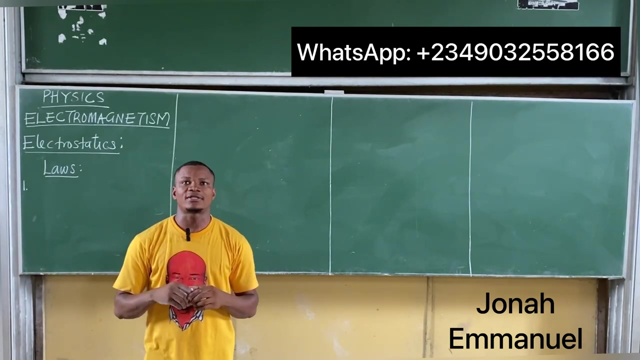 Two laws of electrostatics. number one: Light charges repel and unlike charges attract. That's it. That's the first law, And unlike charges attract, That's your first law. Law two: hold on. Law two is what we'll be dealing extensively on. 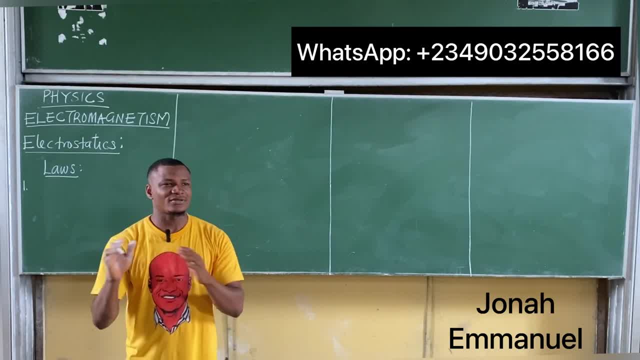 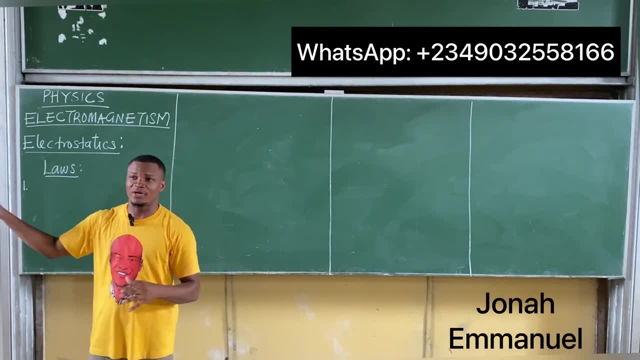 So keep law two pending. Let's look at something else. Keep law two pending. We'll treat law two much more later. Keep it pending, Take down please. I'll give you the second law much more later. Just keep it pending. 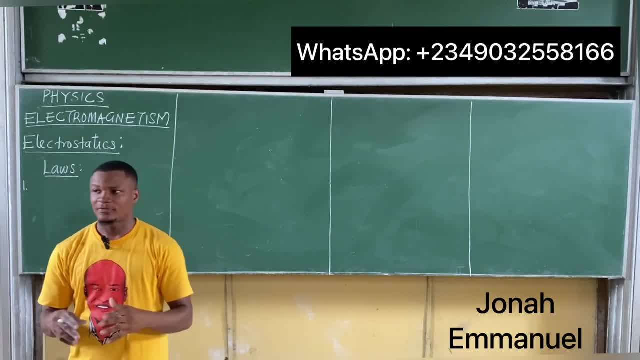 Take down, please, Methods of charging a body. Take down, please, Methods of charging a body. I said we'll do law two much more later. It's kind of complex. It involves calculation, So let's save the calculation for later. 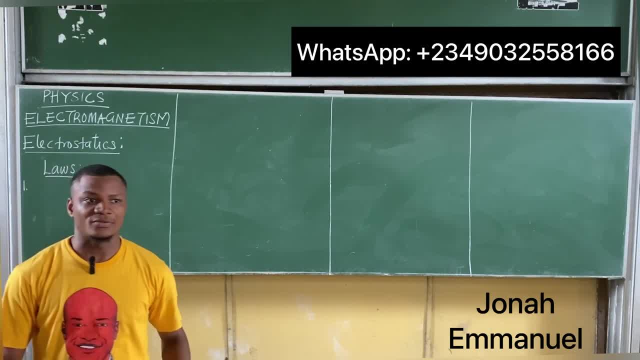 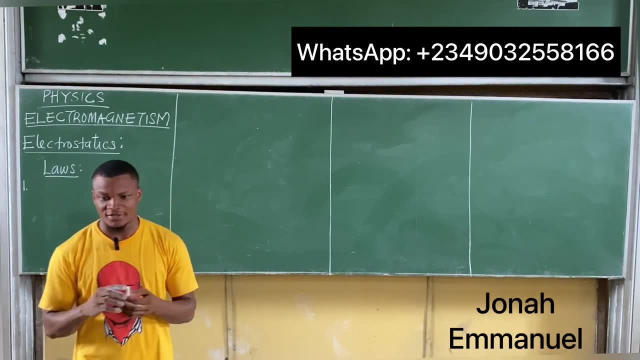 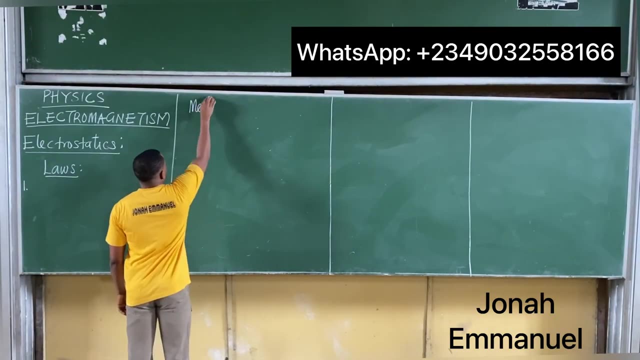 Let's take down as many definitions as we can before we do calculation. All right, Methods of charging the body, please. The different. The different methods of charging a body includes The different methods of charging a body. The different methods of charging a body includes number one. 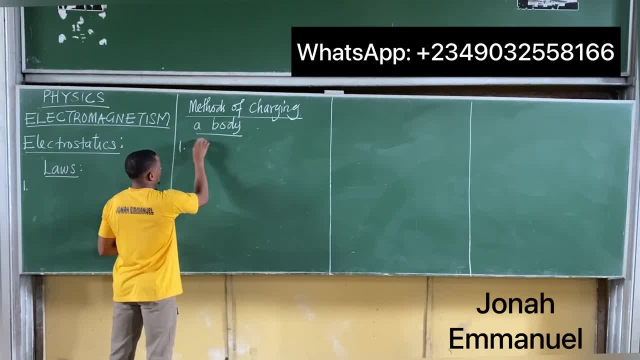 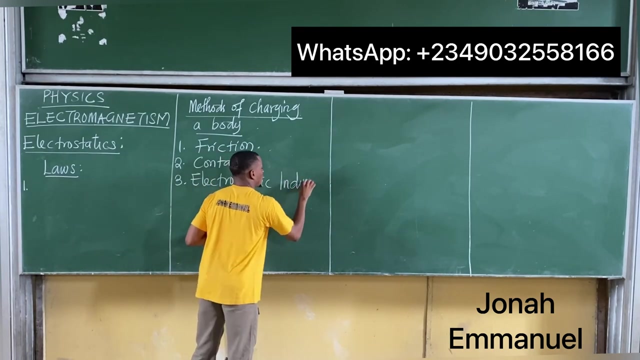 charging by Number one: Number one: Number one One. charging by friction. Number two: charging by contact: Number three: charging by what is called electrostatic induction. Right, You have this please. This was also a past question. 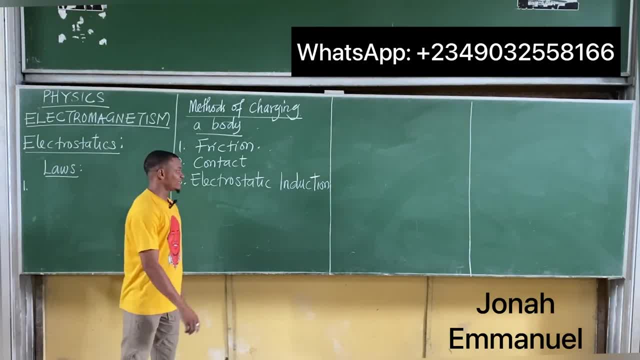 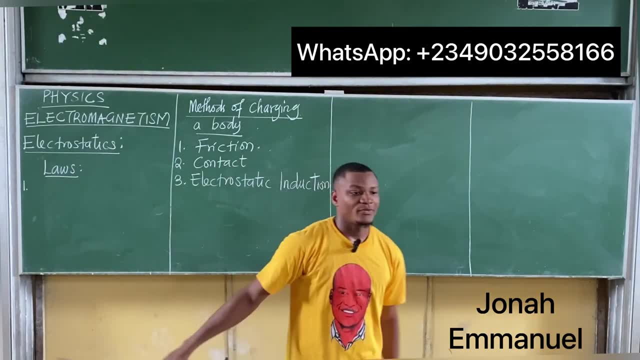 They said: explain electrostatic induction. That was college question. What is electrostatics? That was science's question. We'll see them shortly. All right, Different methods of charging a body includes: number one by friction, number two by contact. 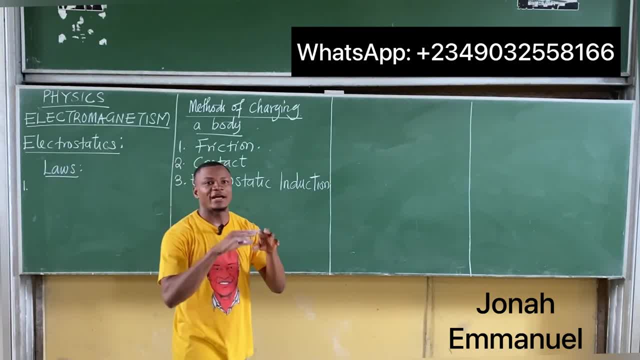 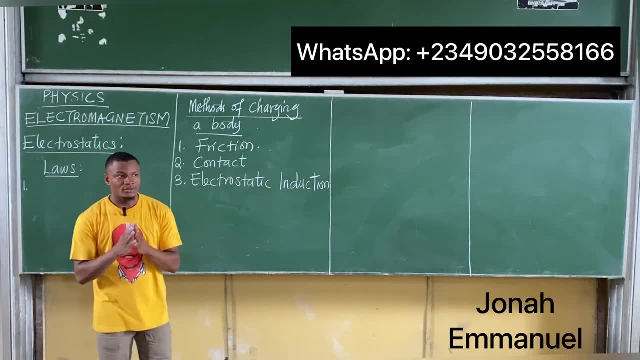 number three, by electrostatic induction. So let's just briefly highlight what they mean, and then we'll proceed. Number one, please: Charging by friction. Number one, please, Let's see what it means. Number one, please. 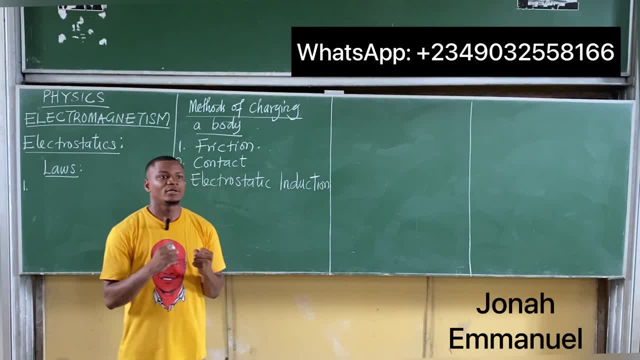 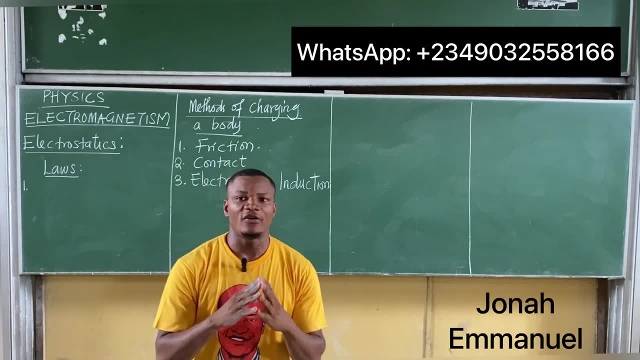 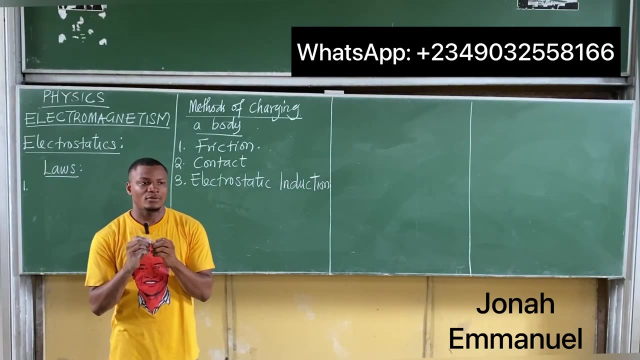 Charging by friction. Number one, please. This involves charging a body by rubbing it against another body. This involves charging a body by rubbing it against another body. Number two: charging a body by rubbing it against another body. Number three: charging a body by rubbing it against another body. Number four: charging a body by rubbing it against another body. Number five: charging a body by rubbing it against another body. Number six: charging a body by rubbing it against another body. Number seven: charging a body by rubbing it against another body. 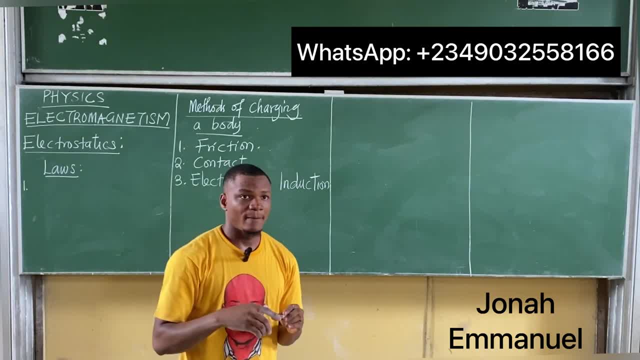 Number eight: charging a body by rubbing it against another body. Number nine: charging a body by rubbing it against another body. Number ten: charging a body by rubbing it against another body. Number ten: charging a body by rubbing it against another body. 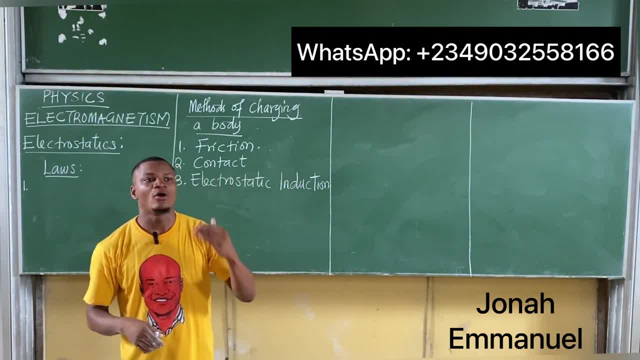 Number eleven: charging a body by rubbing it against another body. Number twelve: charging a body by rubbing it against another body. Number twelve: charging a body by rubbing it against another body Such that electrons are transferred from one body to another. Such that electrons are transferred from one body to another. 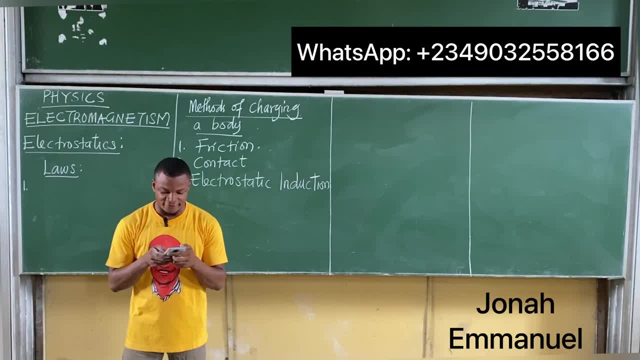 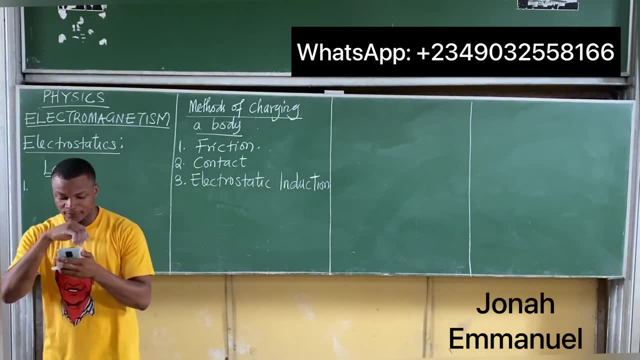 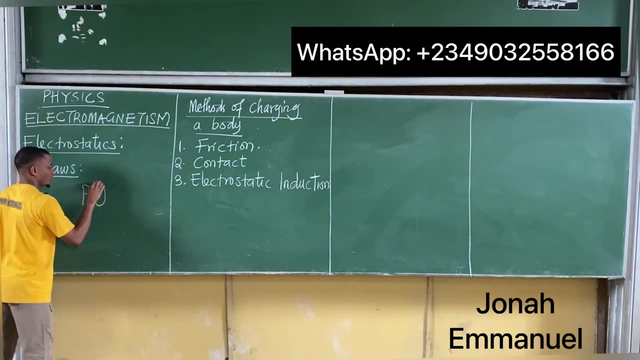 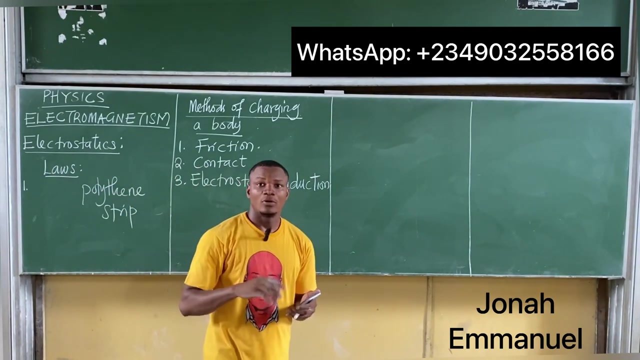 Such that electrons are transferred from one body to another. Example: Example Rubbing a polythene. Example Rubbing here a polythene strip S-R-I-P. Example: Rubbing a polythene strip with biro. 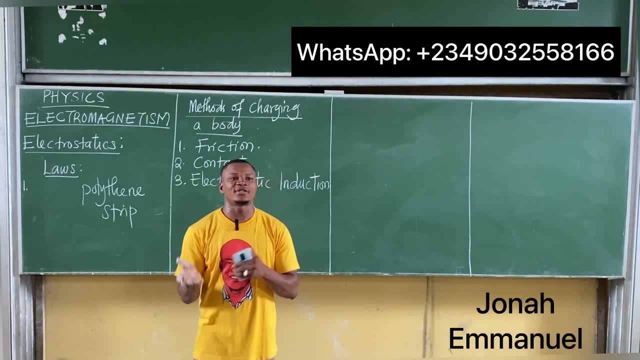 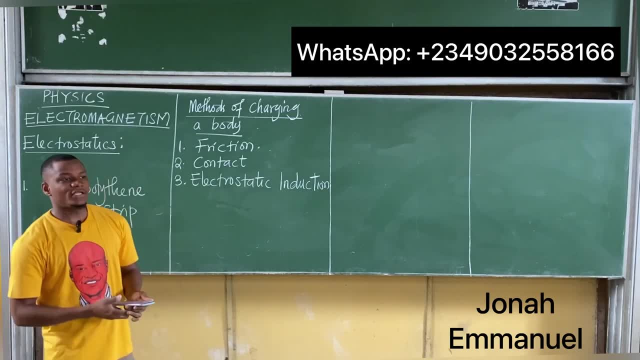 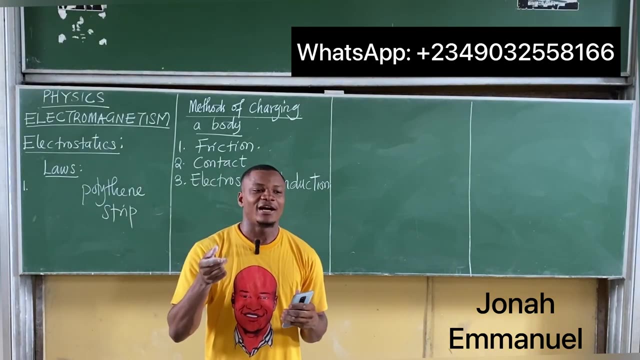 Example: Rubbing a polythene strip with biro. Full stop. This stuff, this concept here explains the- in quotes- magic that we did when we were smaller Guys. if you actually did that there, that this magic we do. what's the magic there? 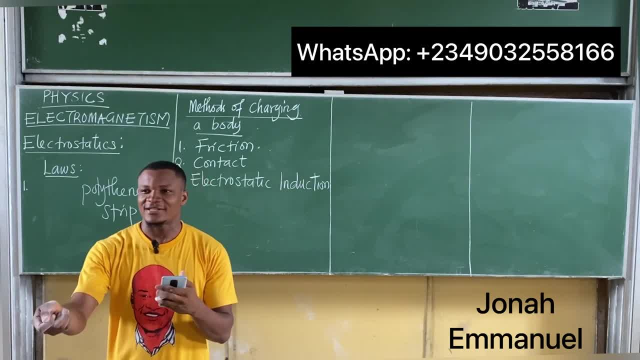 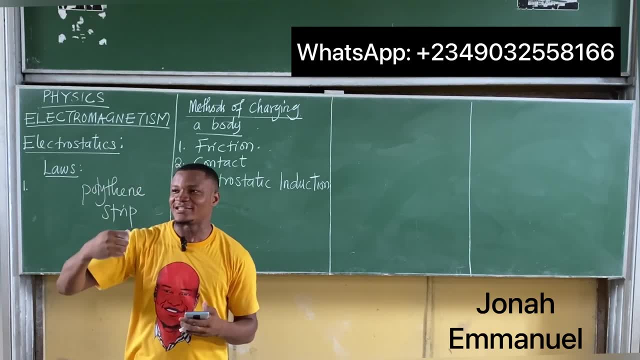 You tear a piece of paper and keep it on a desk. You carry your pen and touch it. Nothing happens. What do you do next? You cut and do what there. Rub it on your head, Is it not? But when you touch it, what happens to the paper there? 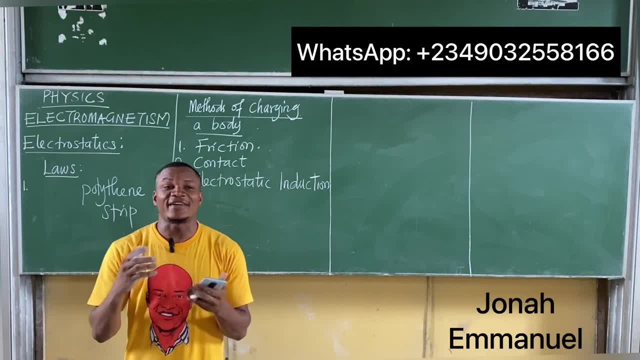 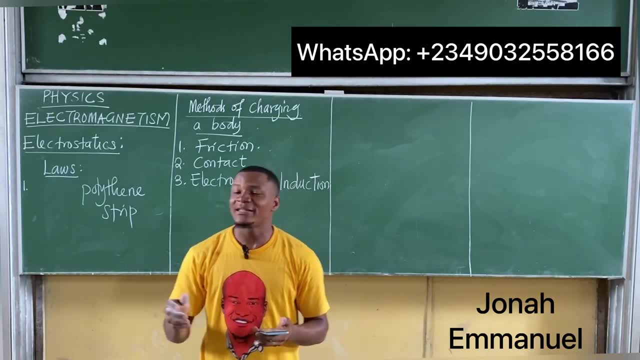 It starts moving and they say it's magic. It's not actually magic. Now here's the idea: when you had that pen and that paper, at that point the pen was not charged. By the time you used that pen to rub against your head, you've charged the pen by what? 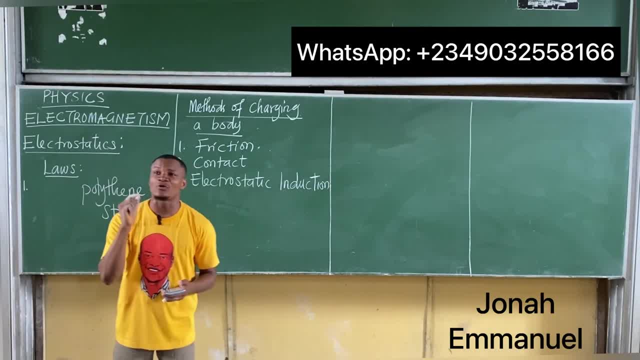 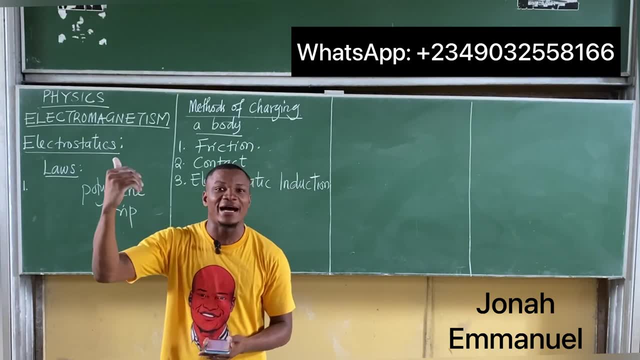 there Friction. So there's a friction between that biro pen, that biro cover and your head. That stuff now creates charges such that the charge on the biro pen and the paper becomes what there Opposite charges. And then, when you bring it closer, what happens there now? 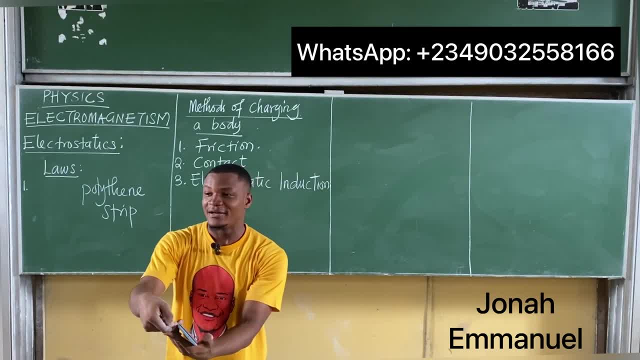 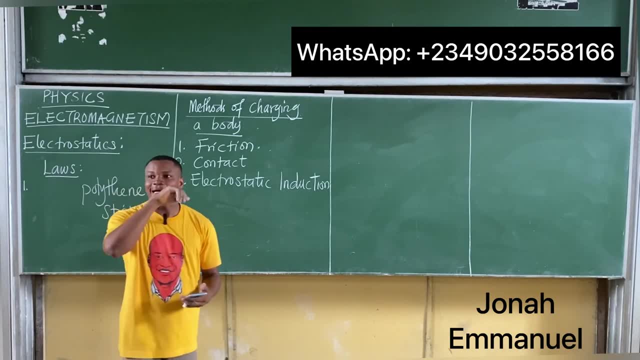 It starts doing what there Attracting, And you call it what there Magic. So this explains it. Okay, Number 2.. So that's the first one there. Charging by friction: Number 2.. Charging by contact: Number 2.. 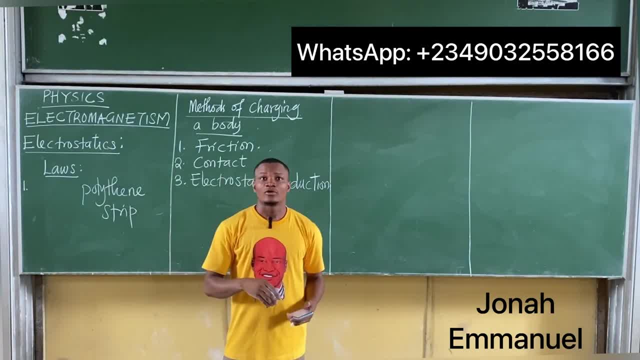 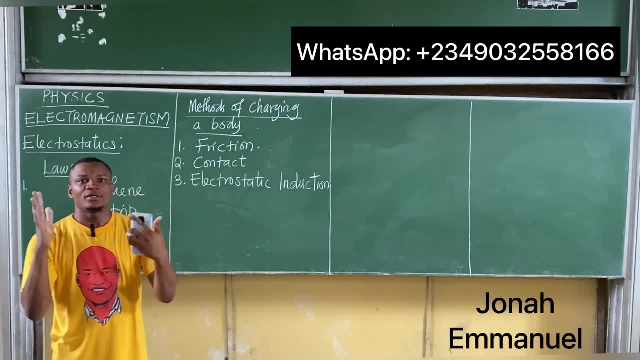 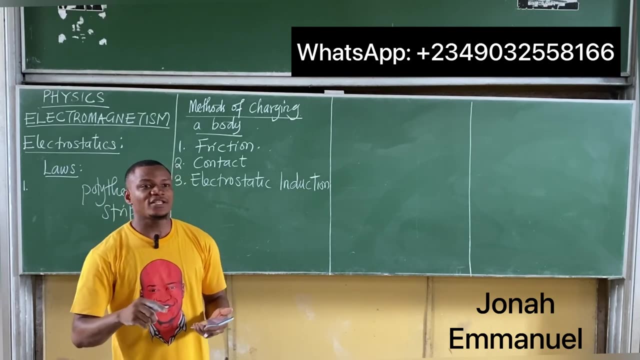 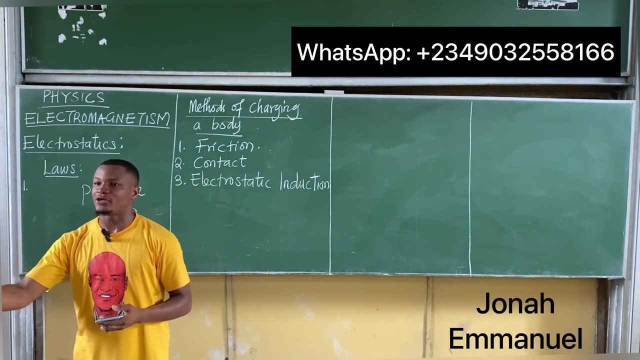 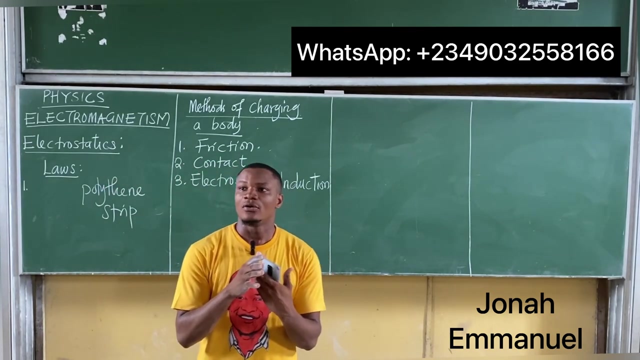 Charging by contact Number 2. Charging by contact: What does it mean? This involves charging a body. Okay, Use neutral body. This involves charging a body. Charging a neutral body: this involves charging a neutral body by bringing it in contact with a charged body. 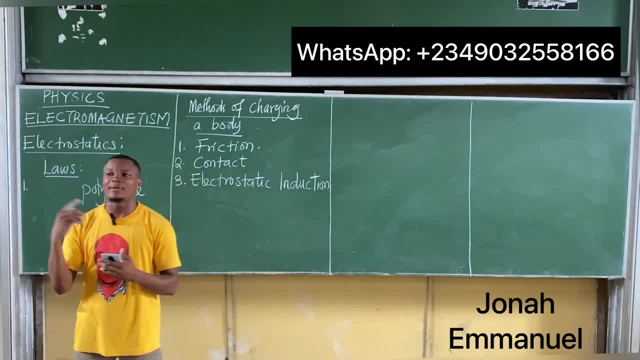 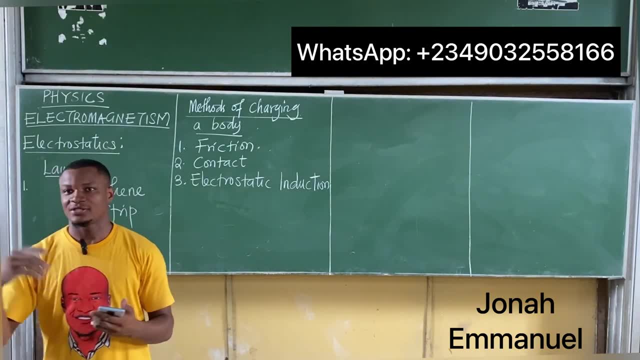 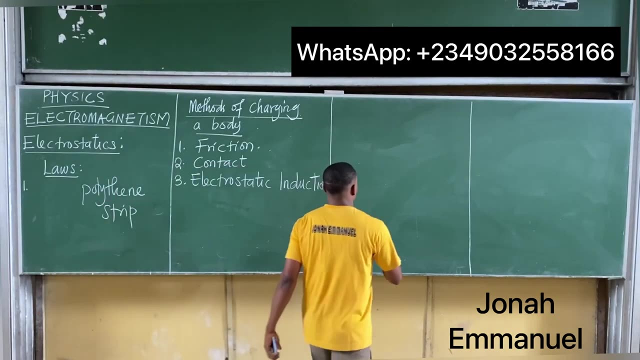 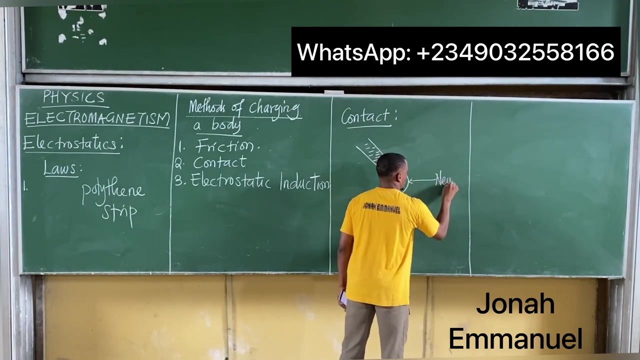 Charging by contact involves charging a neutral body by bringing it in contact with a charged body. Charging by contact involves charging a neutral body by bringing it in contact with a charged body. by bringing it in contact with a charged body: Asin Bilu, Asin Bilu. 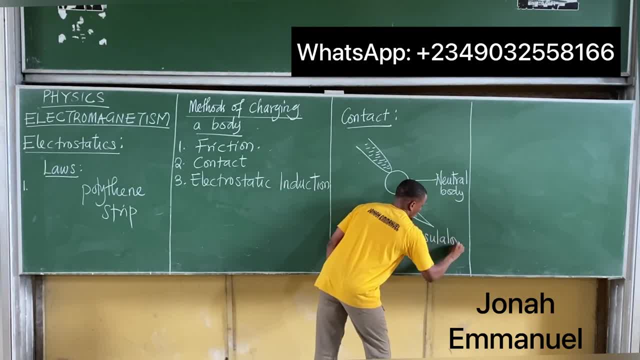 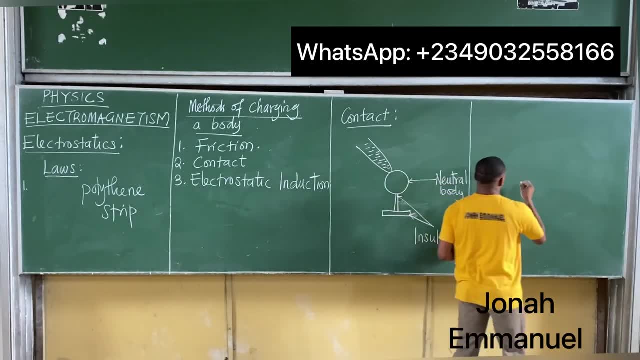 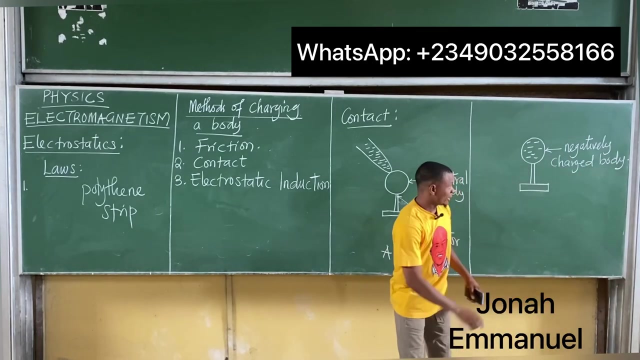 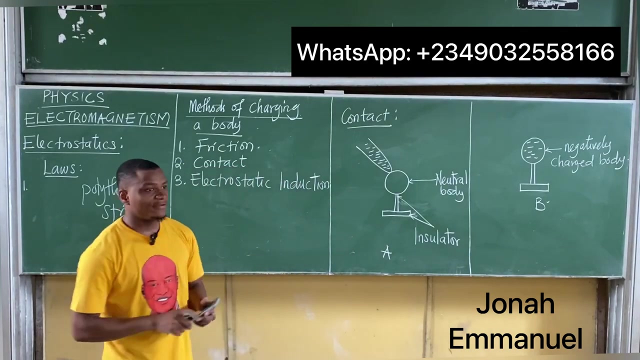 Asin Bilu, please. Thank you All right, So here's a diagram for charging by contact, please. Here's a diagram for charging by contact. You have diagram A, diagram B. Here's a diagram for charging by contact. You have diagram A and diagram B. 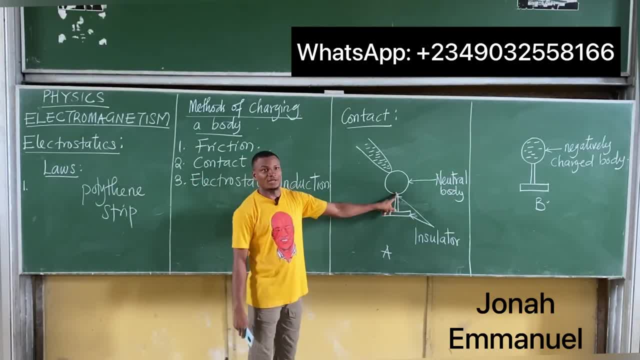 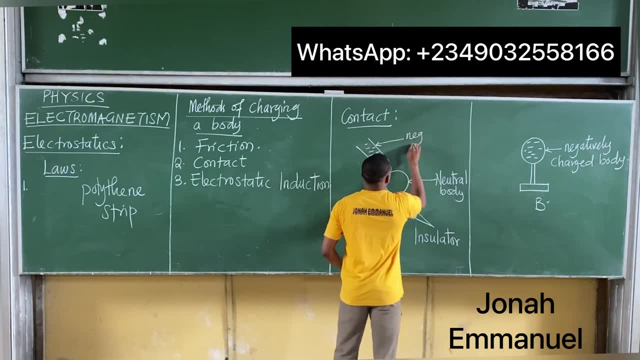 For A. what do you observe? I have a neutral body. What next? I bring a negative. Okay, so put here. You can add here Here, negatively charged rod, Negatively charged rod. So you bring a negatively charged rod in contact with the neutral body. 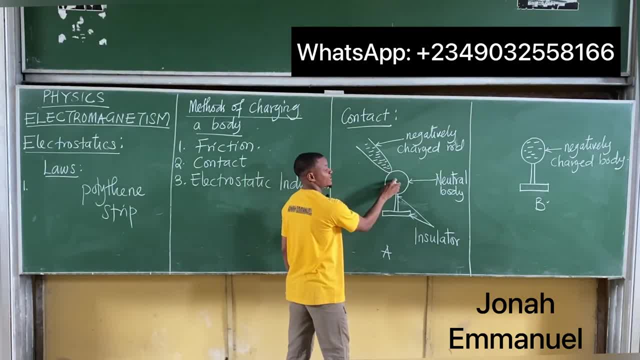 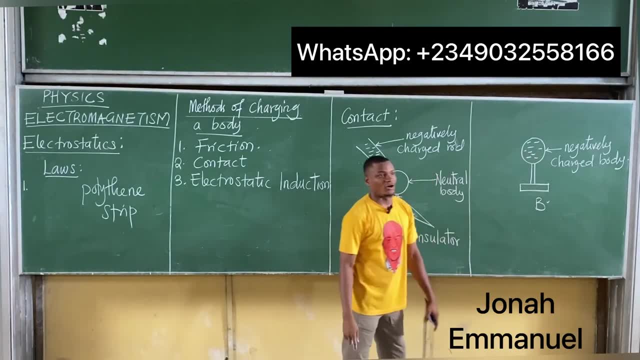 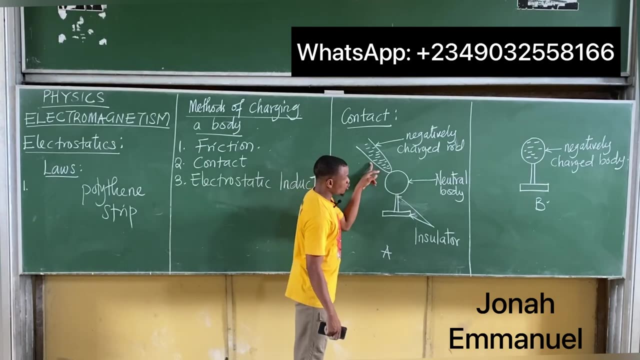 What happens here now? The electrons flow into this, So electrons move into this, And then when you take off the rod there, I'll be having electrons here, So it becomes negatively charged. That's all You see. why there Bring a negatively charged rod close to a neutral body. 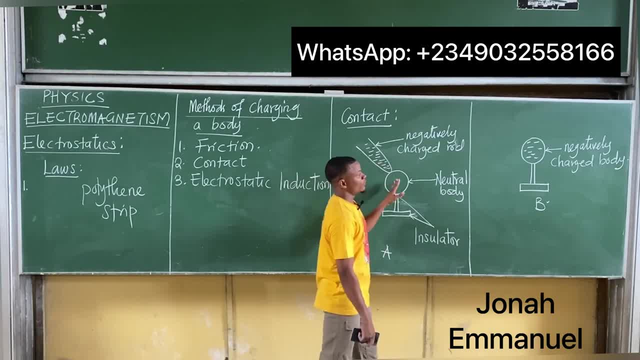 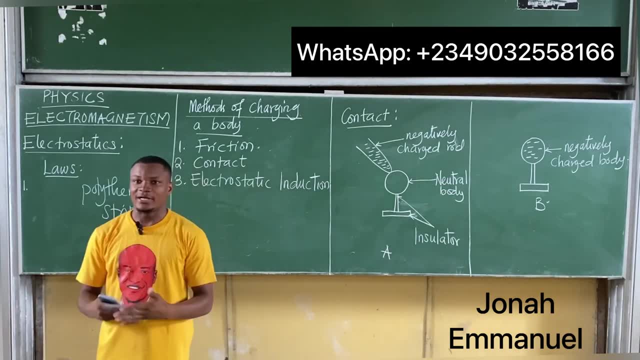 Take off the rod there, You observe that the electrons from here will flow into this. And then I have this one here. So that's as simple as it gets. So that's charging by contact. This stuff explains if you did. these days, birthday parties are different from how it was during my time. 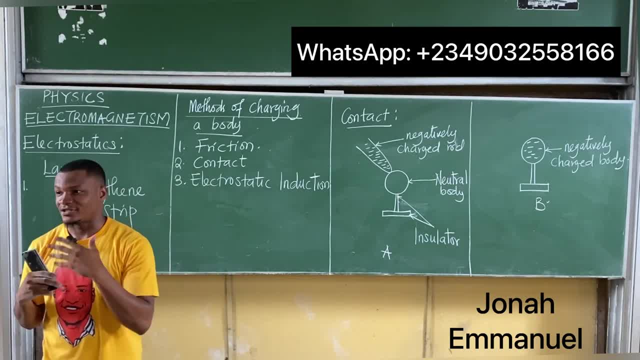 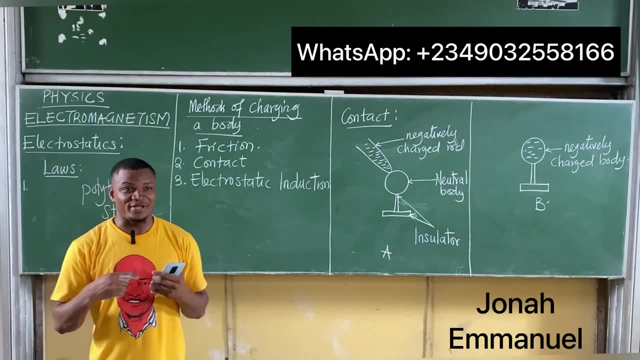 This December is two years old And the birthday present Is three plots of land and the G-Wagon. in this age, my turn, my time, what we're doing, birthday party. how was it You call all the children in the neighborhood, is it not? 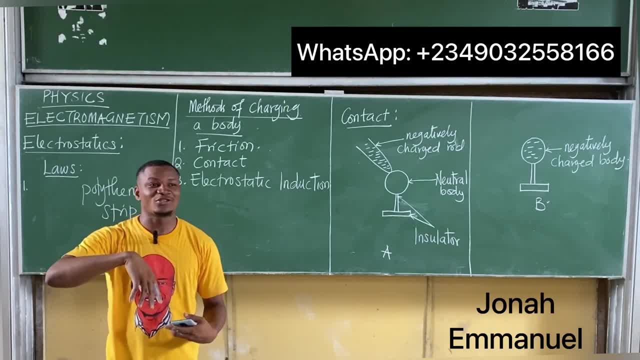 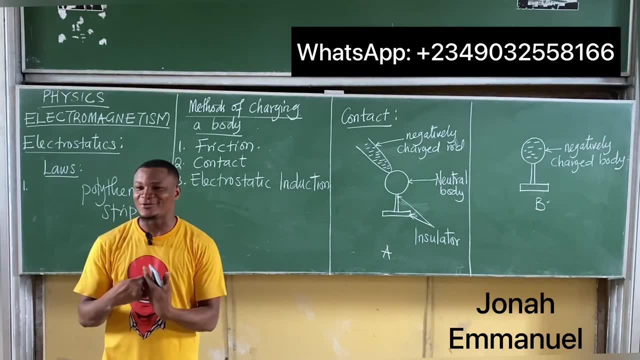 You keep plastic all around. What does he do? You cook rice inside that big stainless tray, is it not? Yes, If you know Gen Z will not, will not relate, right? You put rice inside that big tray and then have to go around the day. 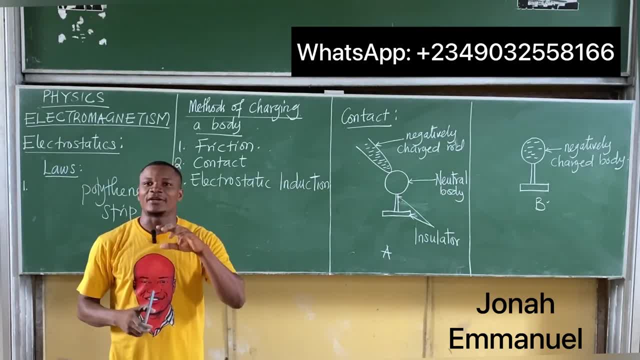 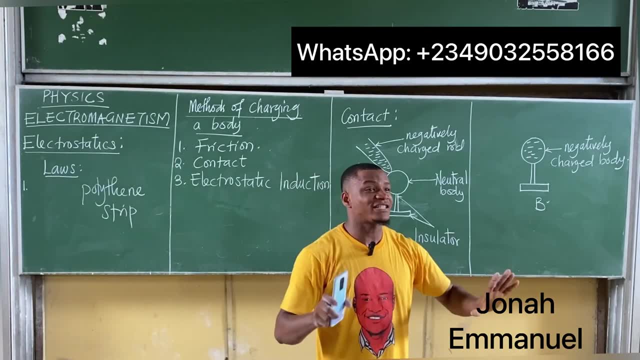 But here's the thing. here's the thing. there is something about those events. How do you not go to this kind of events where you sit down there on a plastic chair, you're seated and then all of a sudden you start feeling ant-like movement on your hand? 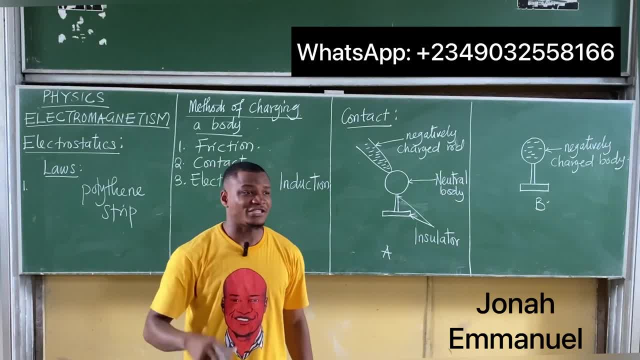 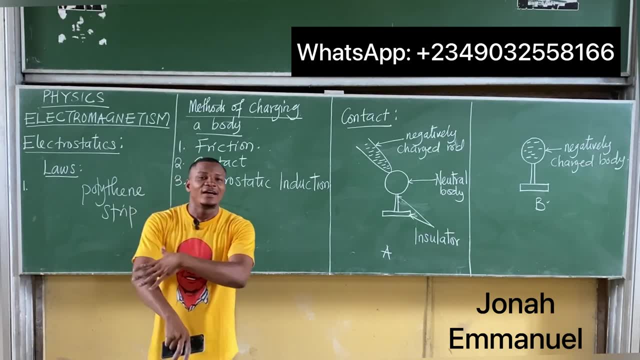 Do you feel it there? Yes, Um, plastic chairs. really, When you sit on a plastic chair, observe, do you feel some kind of sensation as if ants is there, And then when you check, there's no ants, But you're feeling a kind of. 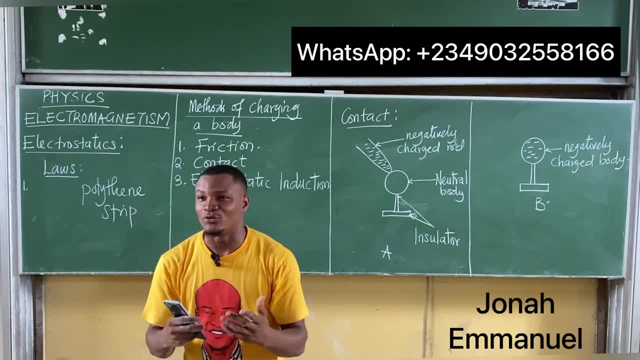 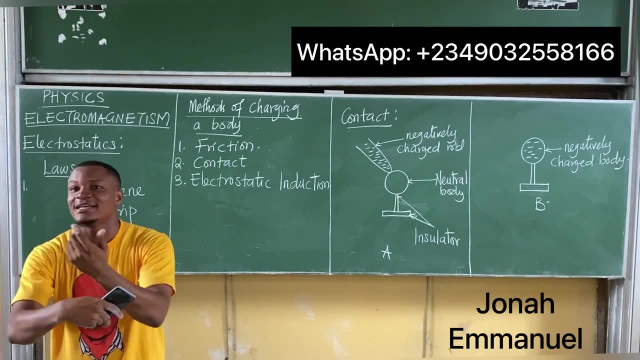 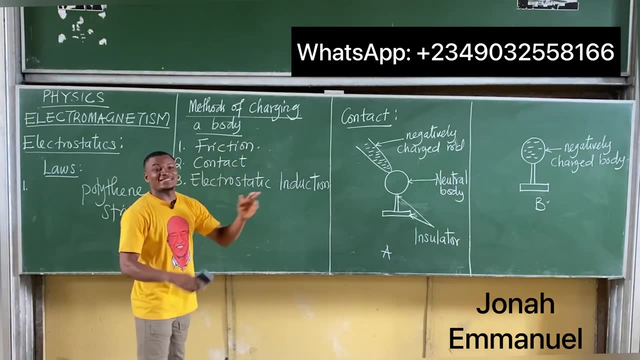 What's happening? The idea is simple: As your skin is having contact with that plastic chair, you are having contact, So hence your, your input. your skin is being input charged, You're actually charging yourself. So that sensation you feel is actually what they're: electrons. 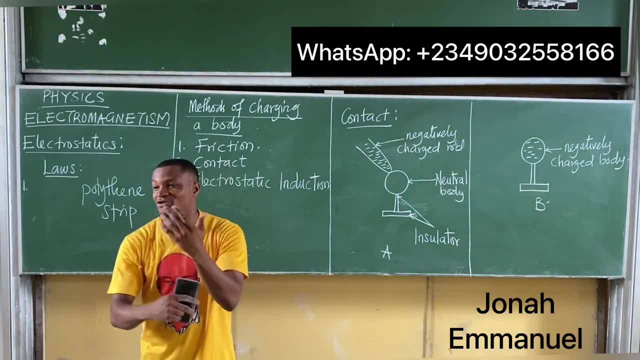 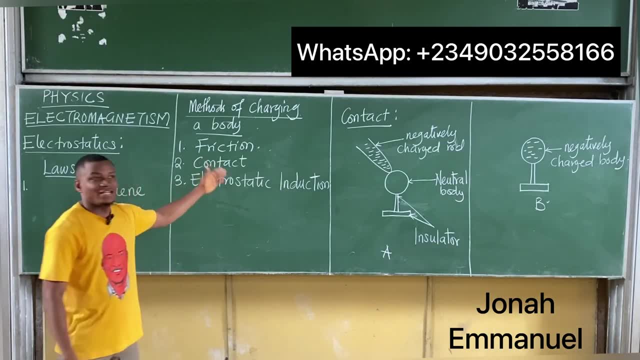 That's it, So that ant-like movement is not ants, It's electrons that actually will be what they're flowing. So this explains um that stuff. So this is charging by contact. Let's look at the last one, please. 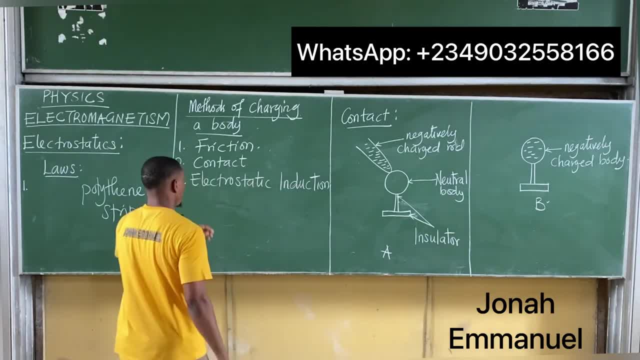 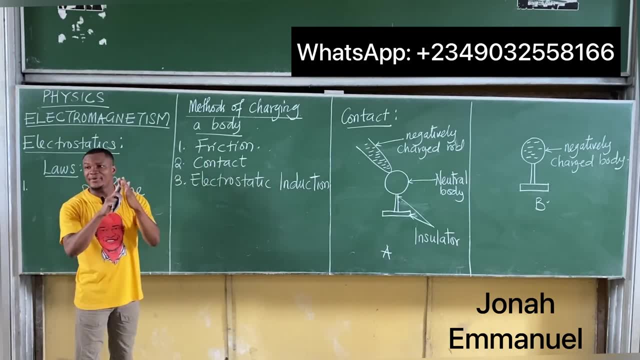 Charging by electrostatic induction. These two are similar. These two are similar. What's the difference? For this one, it involves what they're rubbing of the surfaces. For this one, here there is contact, but there's what they're no rubbing of the surface. 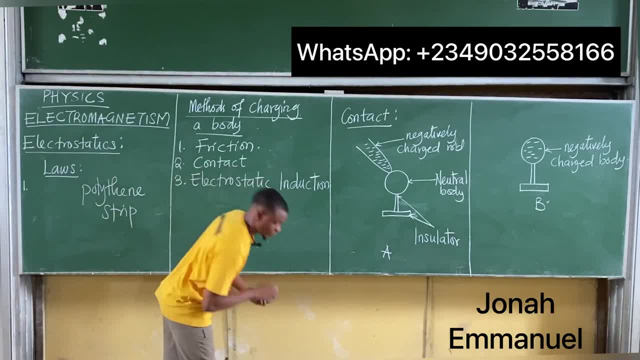 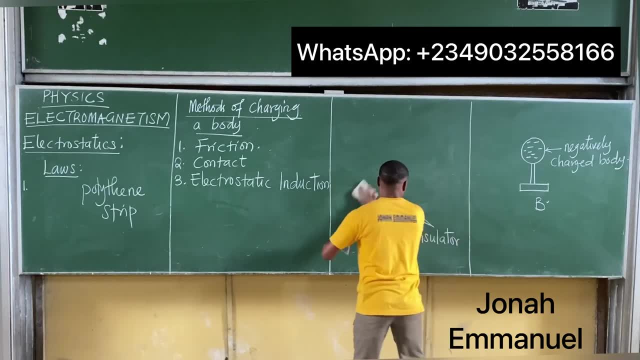 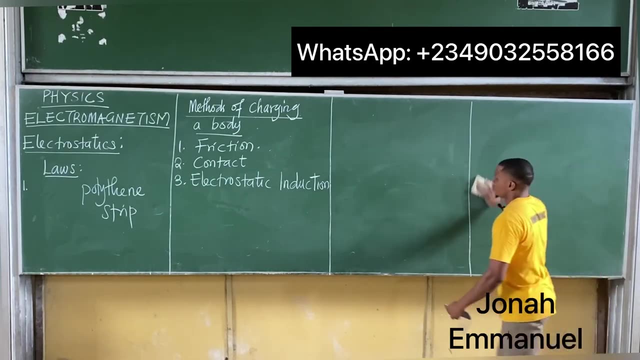 That is the difference. All right, Last one, please: Electrostatic induction. Electrostatic induction. So here's the difference. Here's the difference, please. These two somehow involve contact of the two bodies. For this one here, um, for these two processes I charge a body by bringing them in contact. 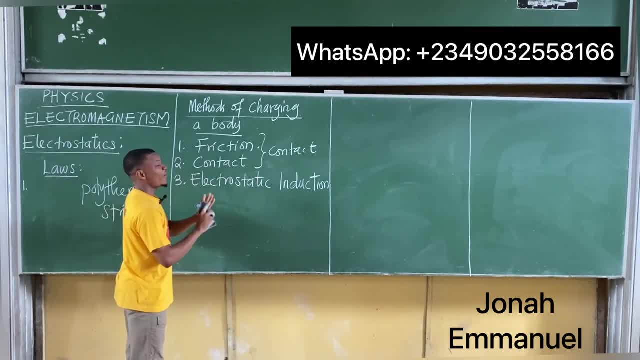 Whether I choose to rub it though, in case of friction, or I choose not to rub it in case of contact, both of them involve a contact. For this one here, I'll be charging a body without any contact. That's it. 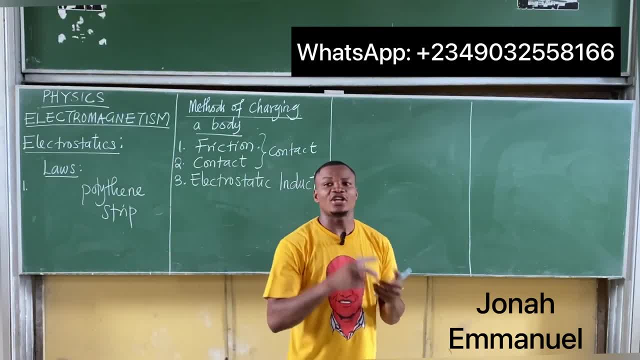 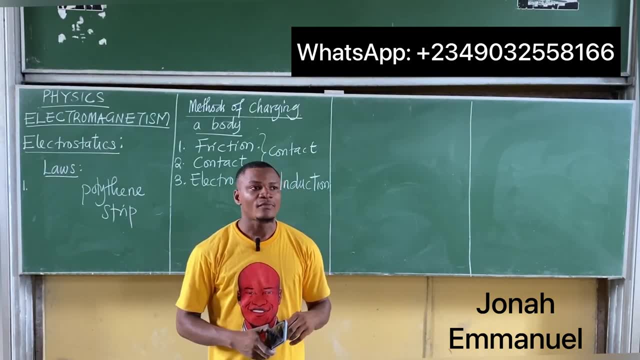 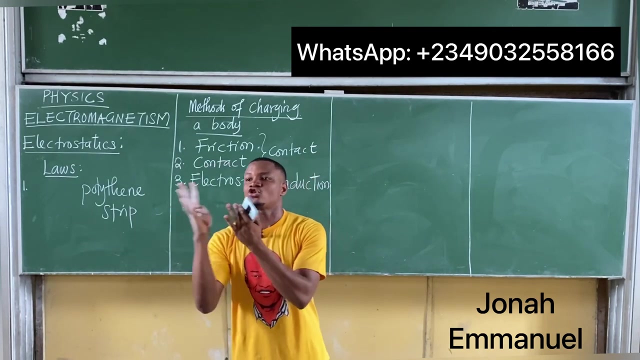 So take that please. Electrostatic induction involves charging a body. Use the word neutral body. Electrostatic induction involves charging a neutral body by placing it close to electrostatic induction. involves charging a neutral body by placing it close to electrostatic induction. 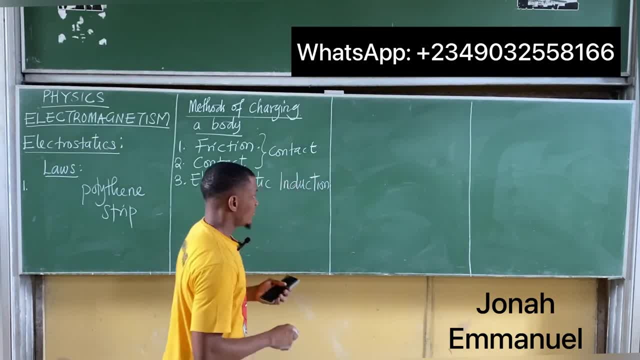 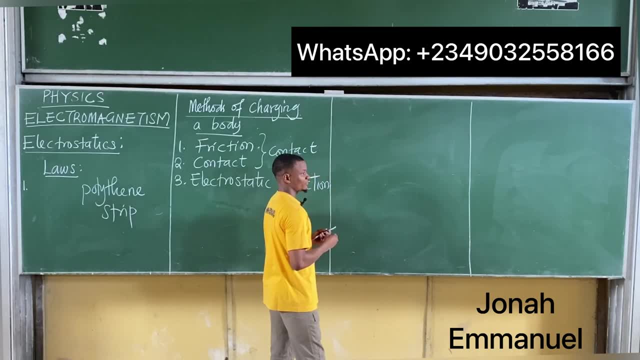 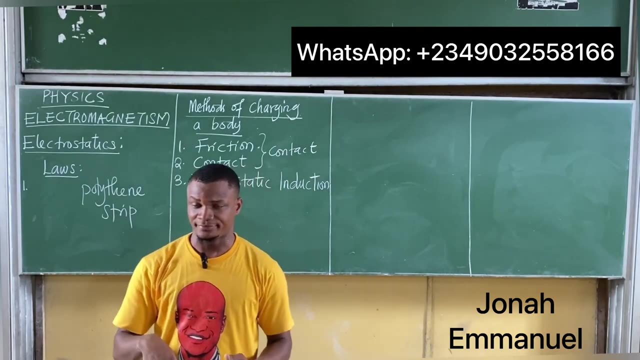 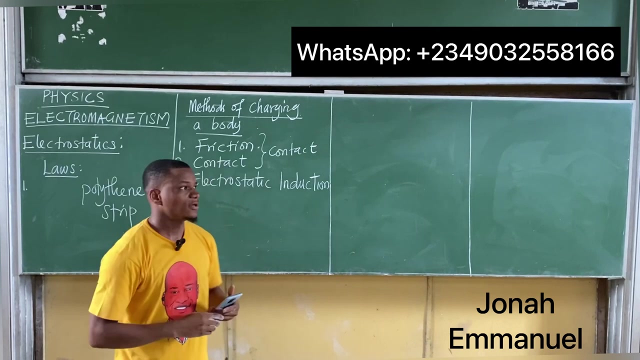 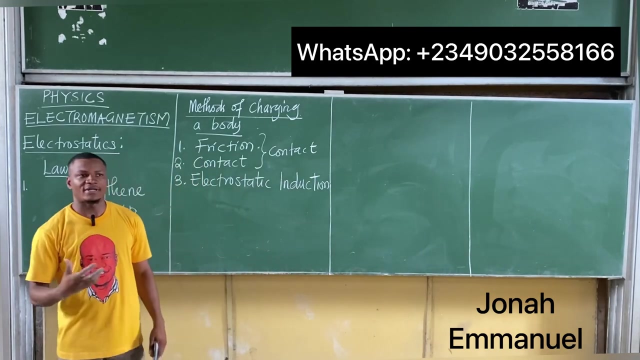 A charged body by placing it close to a charged body without any necessary kind of contact between the two bodies, Without any necessary kind of contact between the two bodies, Without Any necessary kind of contact between the two bodies. So please look up, please. 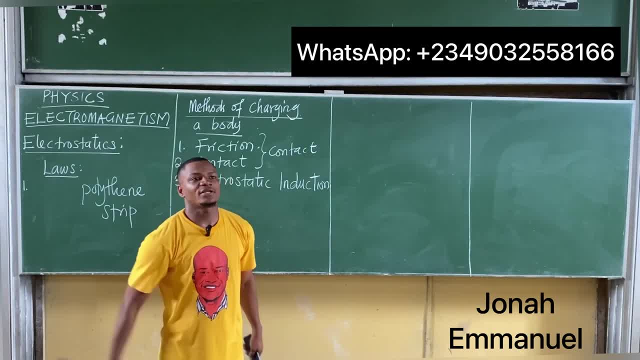 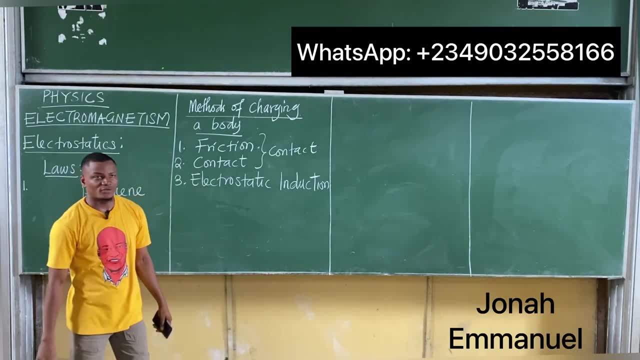 Look up please. I'll give you a note. Just look up please. Let me explain EI electrostatic induction briefly and I'll give you a note. So look up please. So here's how I do electrostatic induction. 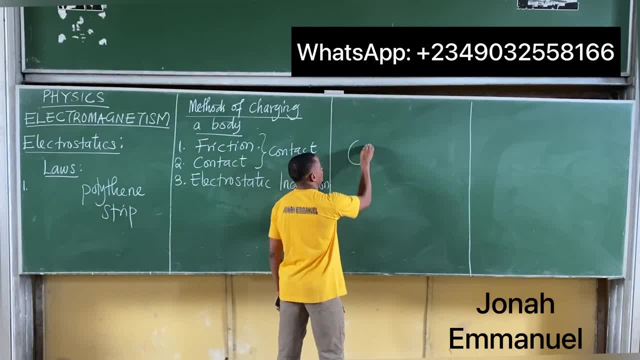 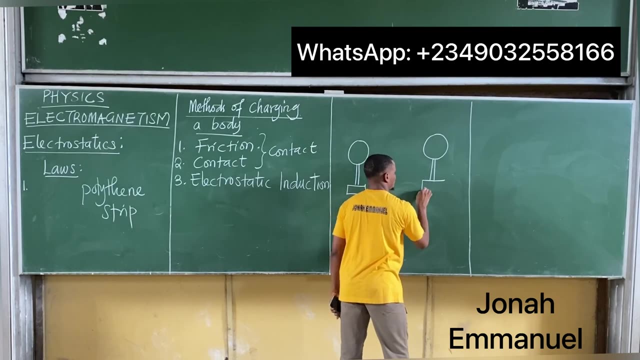 Case one, diagram A: I'm having a neutral body. So here's a neutral body. So this diagram A. I have a neutral body. For diagram B, I'm having the same neutral body. this We said for this one here I'm bringing a charged body in contact with this without any necessary form of contact. 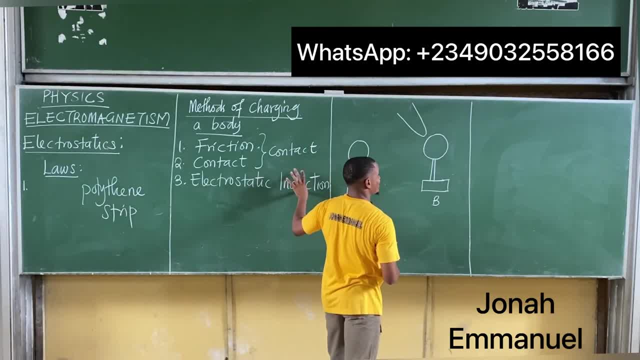 So observe: there's no contact here. That's why I said this one here. there's no contact in this. But I'm bringing this close to this. here, Let's say: here's a negatively charged rod. Let's say: here's a negatively charged rod. 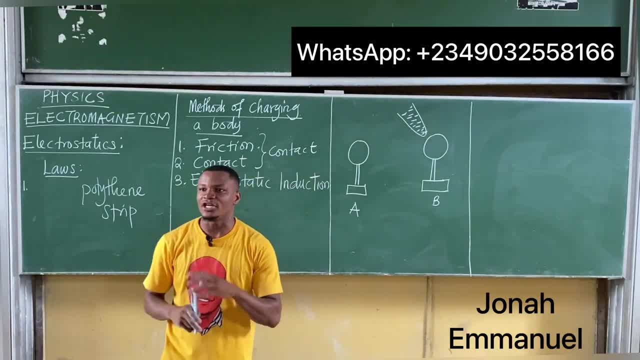 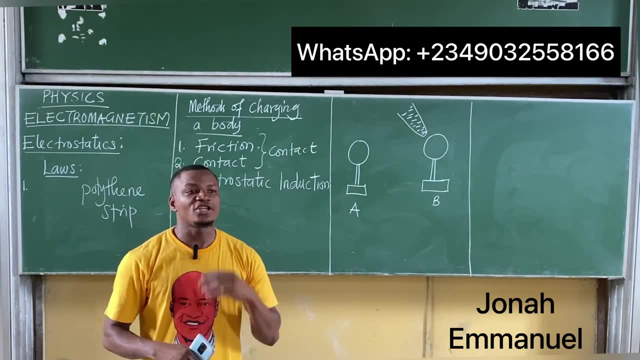 So what happens? And first things first, when a body is neutral, it means that body does not have protons and electrons, true or false. When a body is neutral, it means the body does not have electrons or protons, true or false. 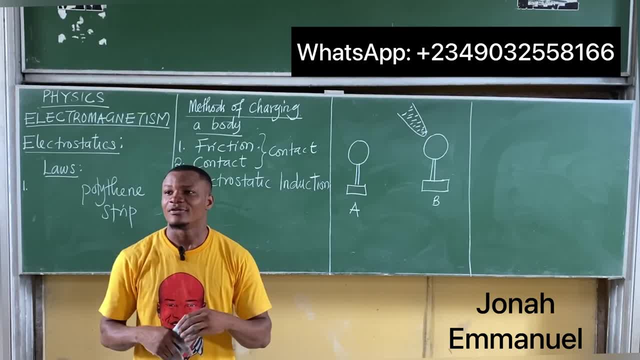 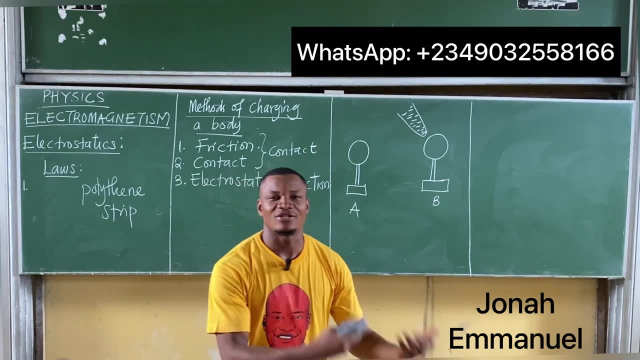 True or false. Talk to me now, feel free. When a body- listen. If a body is negatively charged, it means that it has no electrons or protons. If a body is positively charged, it has electrons. If it's positively charged, it has what there. 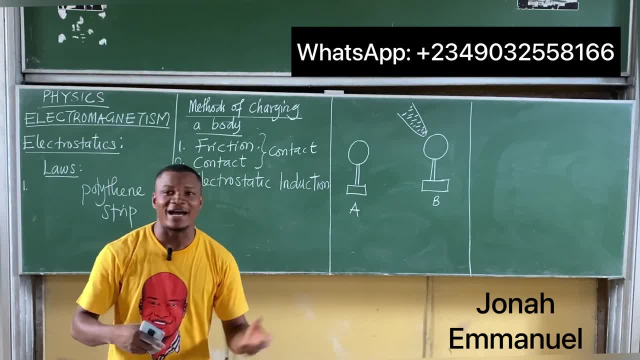 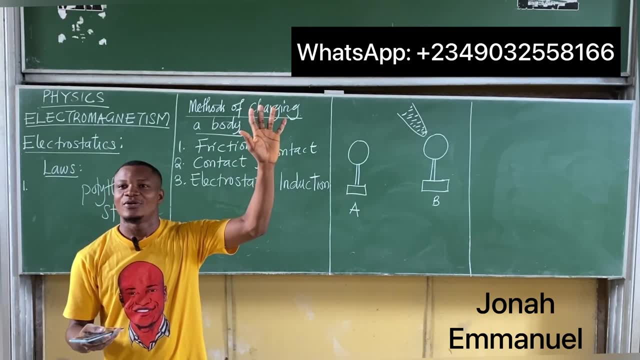 Protons. So if it is neutral, it means it has no electrons and no protons. true or false? True, Let me say that. true Okay. False, Let me say that I think I have more truths than false. 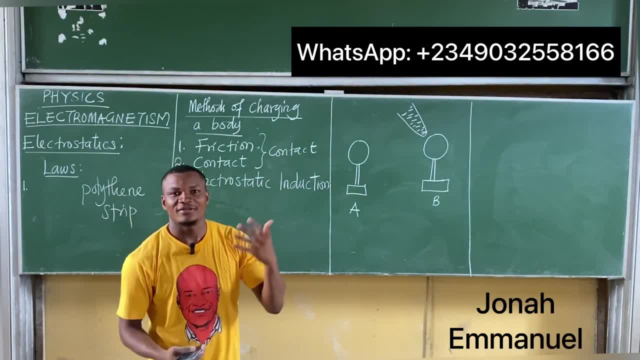 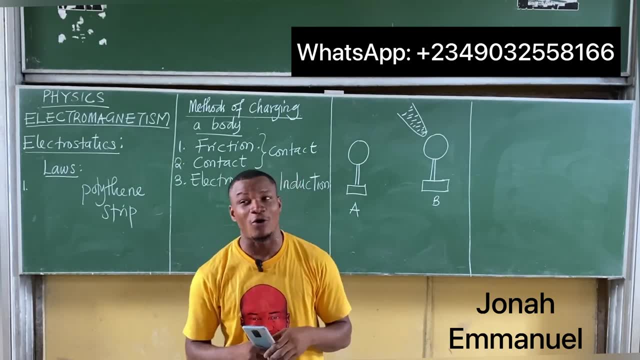 Listen, There's a correlation between physics and chemistry. When a body is neutral, does it mean it does not have protons? True. When a body is neutral, does it mean it does not have electrons and protons? That's false. 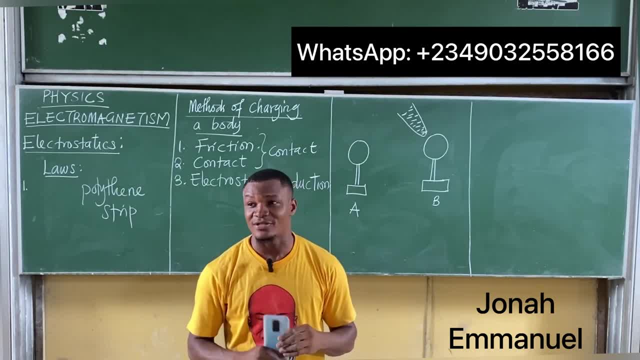 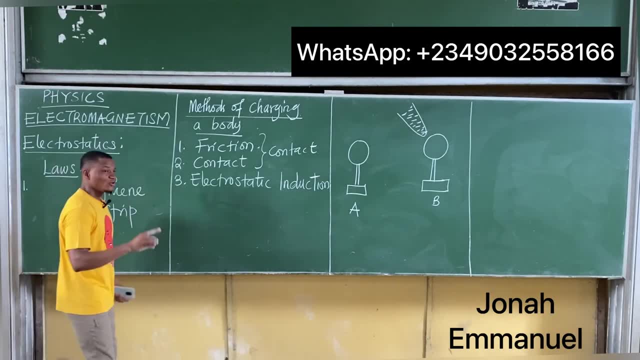 That's false. A neutral body can have electrons and protons and still be neutral. It's possible. How Look at this, please? I don't want to explain this. last semester- I don't know if you've gotten- I said: look at these three scenarios. 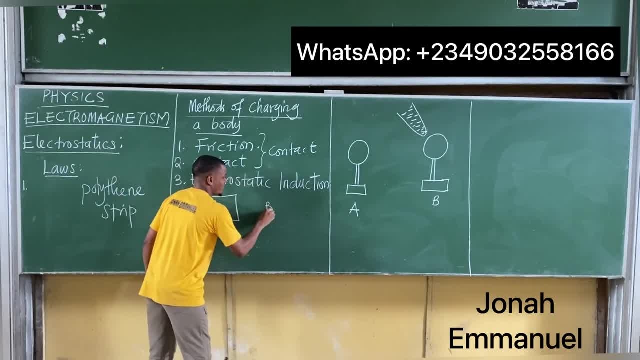 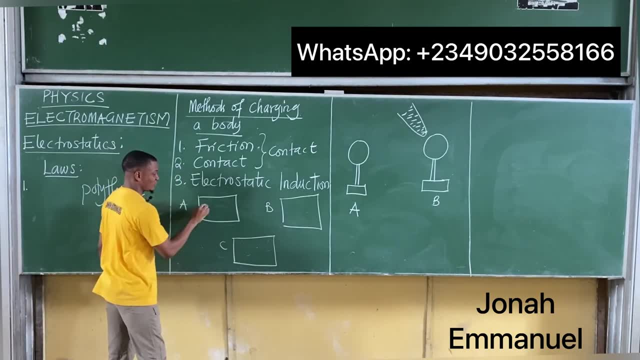 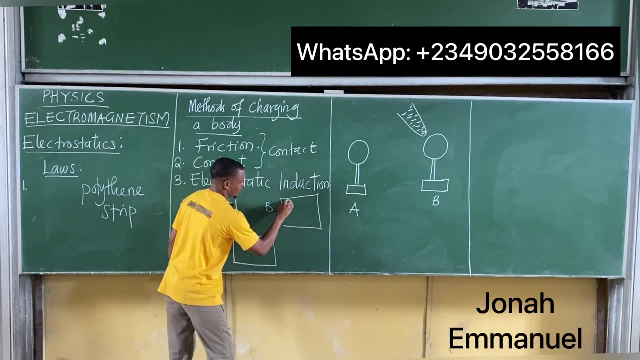 This is diagram A, This is diagram B, This is diagram C. For diagram A, I have more positive than negative, So positive, positive, positive, negative, negative. For B, I have more negative than positive, So let's say positive, positive and I have negative, negative, negative. 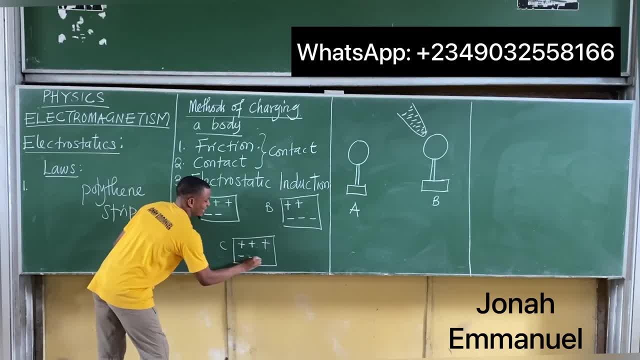 For diagram C, I have equal number of positives and negatives. The positive are my proton, negative are my electron. For this one here, what do you observe? This will cancel this. This will cancel this. Observe that diagram A is positively charged. 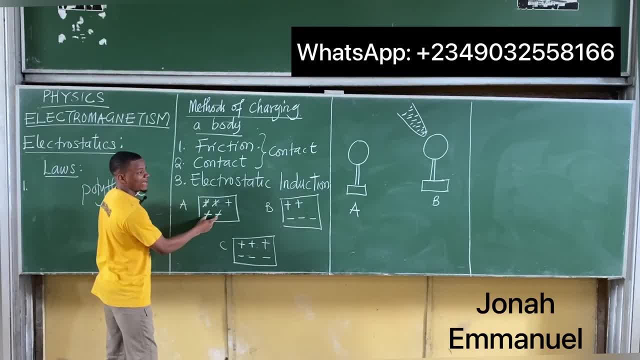 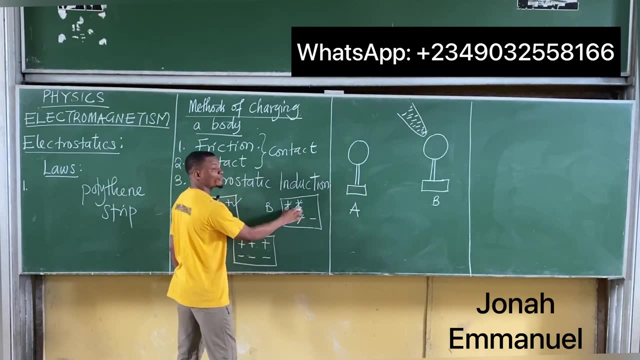 It being positively charged does not mean it does not have electrons. For a positively charged body, I have more protons than what they're electrons. That's the idea. Same thing here. This cancels this. This cancels this. It is negatively charged does not mean it does not have protons. 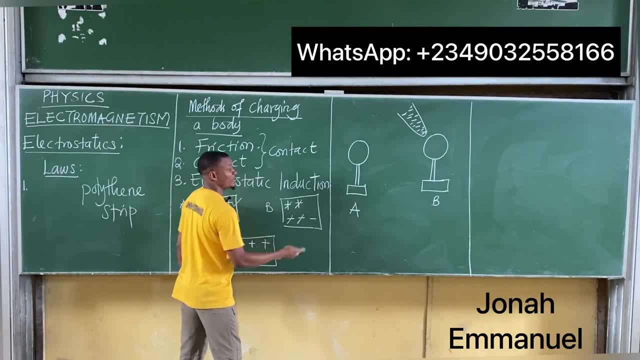 It does. But a body being negatively charged means it has what they're More electrons than what they're Protons For C. this cancels this. This cancels this. This cancels this. It is neutral. It being neutral does not mean it does not have protons and electrons. 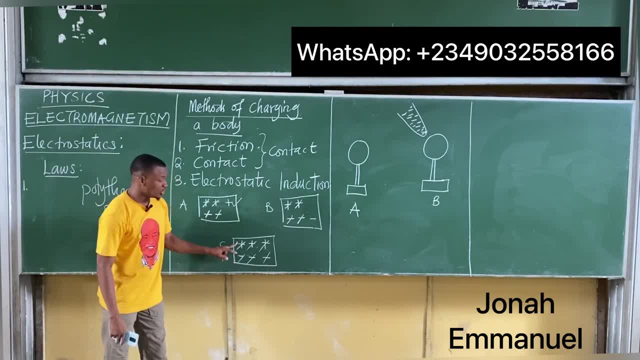 It does. What's the idea here For a neutral body? number of what Protons equal to what there? Number of what Electrons? That's the idea. How does this help us here? Look up please. So if this body here is neutral, it means it has protons and electrons here. 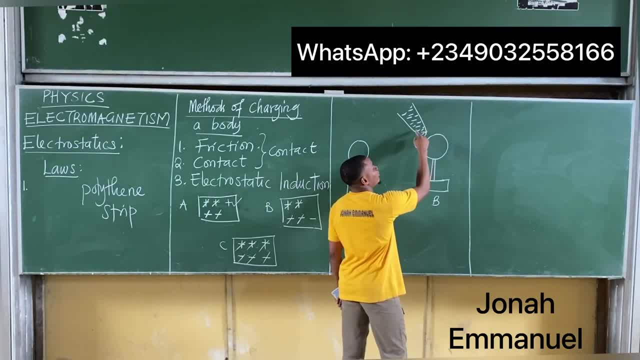 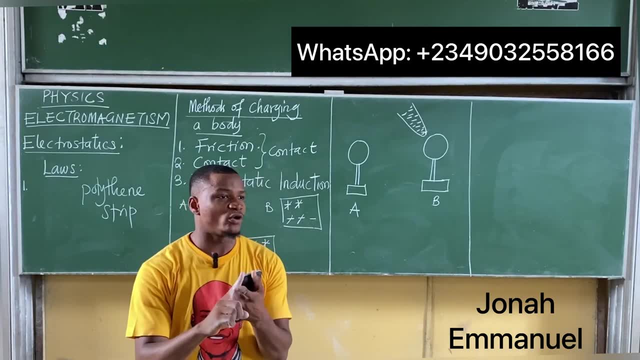 So what? So if I bring a negatively charged body to this one here, from our first law of electrostatics, we see what will happen there. now, Unlike charges- we were there- attract. So that means this point here will be attracted by the unlike charge. 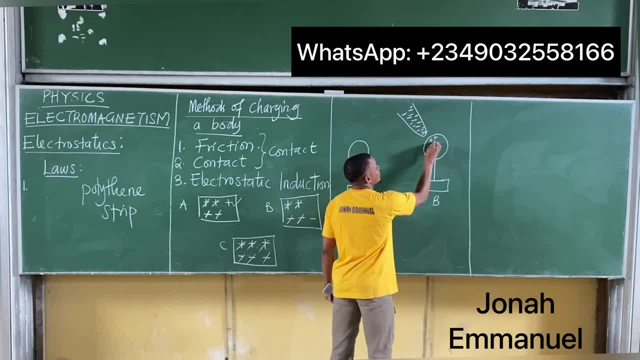 If here is negative, that means positive charges will be here. Why Attraction? So the positive charges that were in this neutral body will be attracted towards the negative part there Also. unlike charges will do what there Repair. That means the negative that were here. 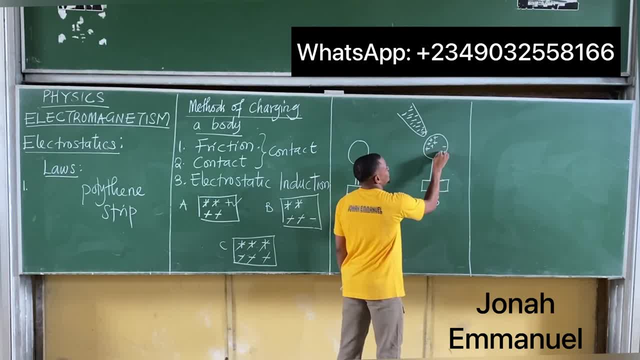 1,, 2,, 3,, 4,, 5,, 6.. So 6 negative: 2. 1,, 2,, 3,, 4,, 5, 6.. Notice that this one here is at the opposite end. 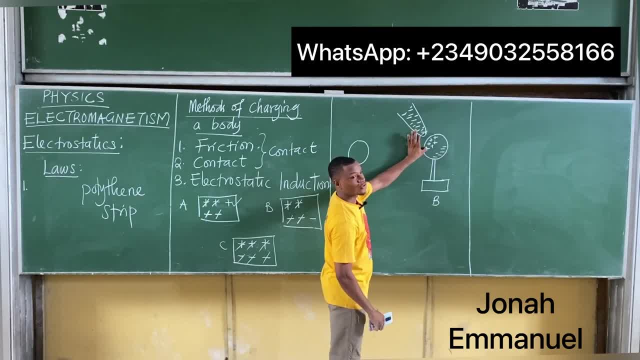 Show you what there Repulsion. These ones here are closed. Show you what there- Attraction. That's the idea, All right. So if I bring a negatively charged rod close to this one here, the positive will go in this direction. 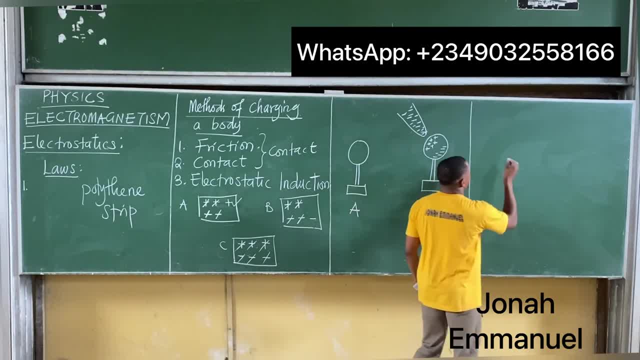 Negative will repair. So what next? At this point here from my diagram C, I will do something called etching. I will do something called etching. So here's what etching means. So this one here, negatively charged rod. 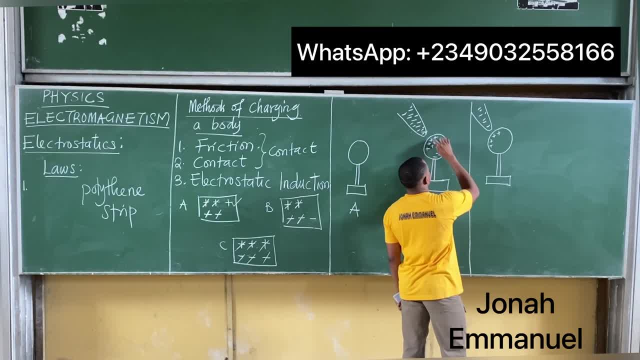 positive here: 1,, 2,, 3,, 1,, 2,, 3,, 4,, 5,, 6,. 1,, 2,, 3,, 4,, 5,, 6, and then 1,, 2,, 3,, 4,, 5,, 6.. 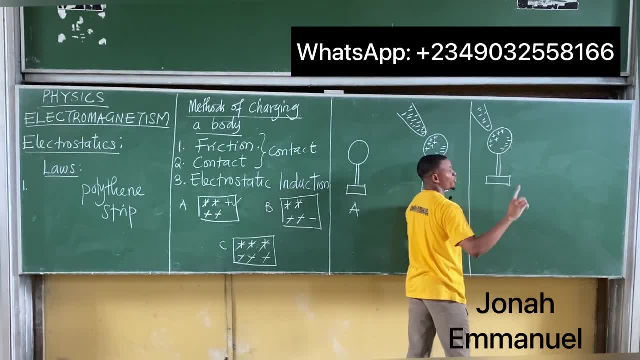 I will etch this. What does it mean to etch? To etch means I will use for. look for a conductor and bring this to etch, Please. this is the symbol for etching What you see. this means etching. 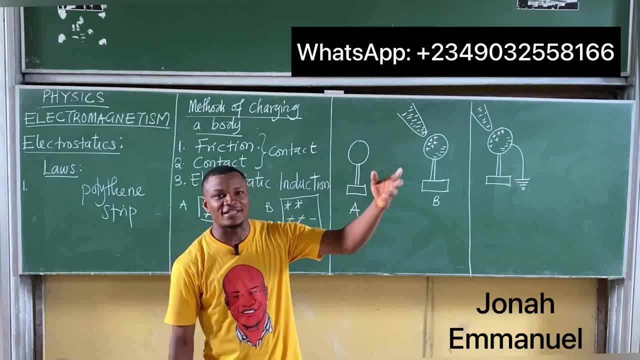 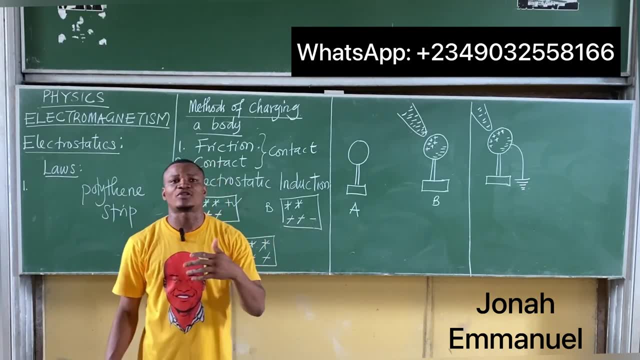 What does etching means? Etching means I'm transferring the charges from a body to the etch. That's what's called etching. This stuff is what you observe If you go through, if you do a lot of travels through the highways. 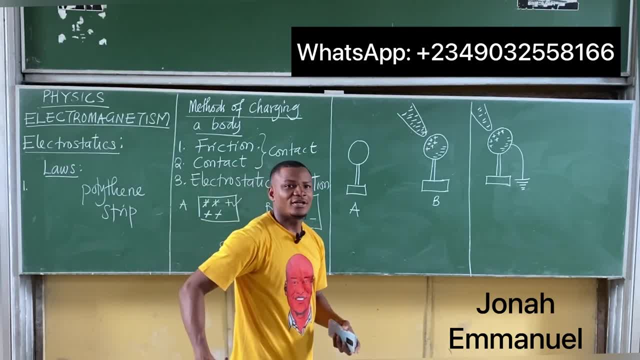 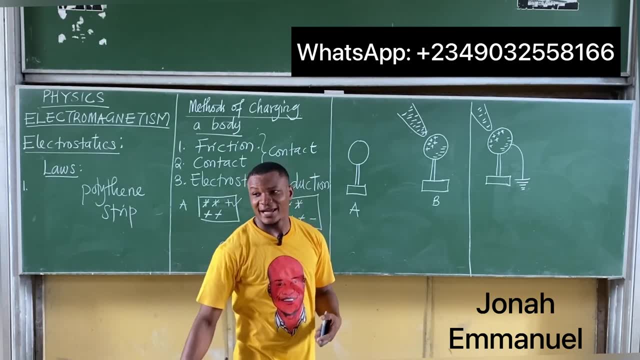 you observe that tankers do have chain, is it not? Tankers have chain connected to them, is it not? And to the ground. Why do tankers have chain connected from their back to the ground? That's what they're etching. 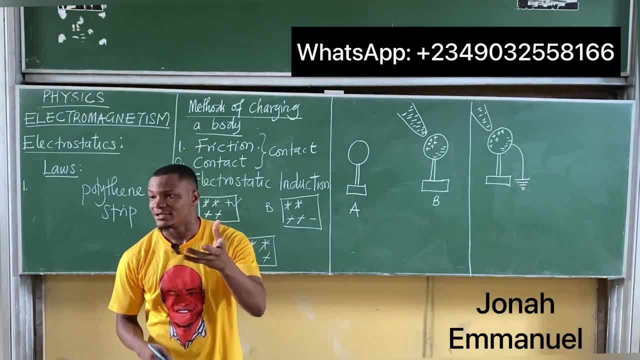 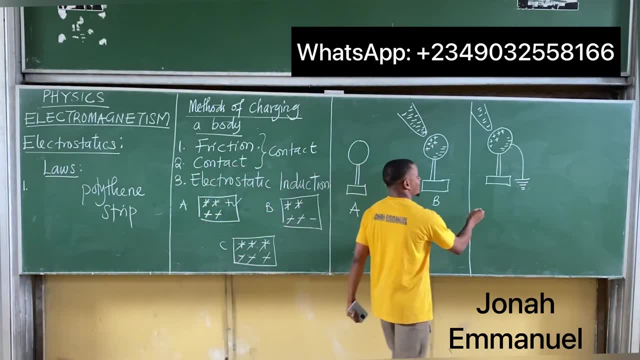 The idea is that this petrol has what they're- a lot of charges. So they now connect the chain to the ground. What's happening there now? They're etching it. If I etch this, this diagram C, if I etch this, what happens here? 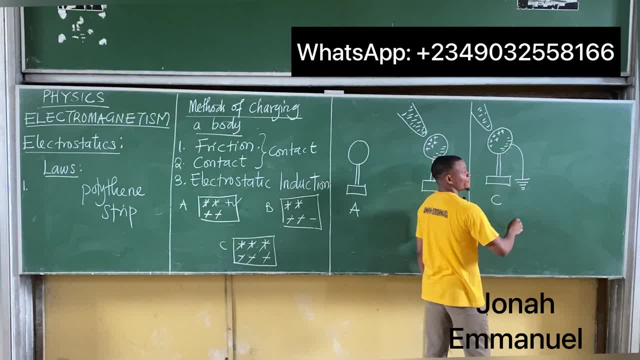 These electrons will now flow out. Electrons now flow out. Electrons now flow out. Electrons now flow out from here. Flows into the etch. If electrons flow into the etch, what happens there? now? I'm left with what there. 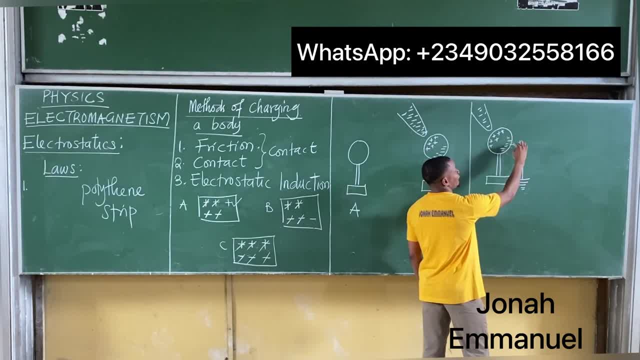 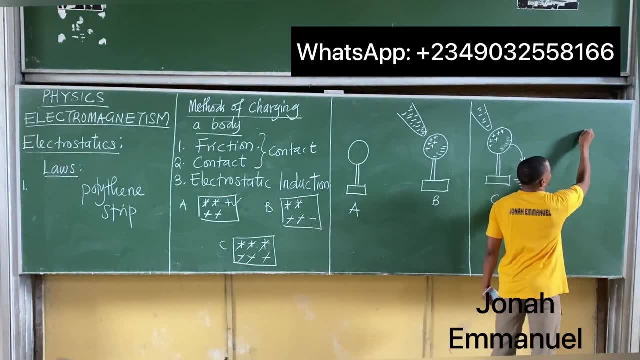 Protons. Please observe, If the charges flows into the etch here, they will leave this point here. I'm left with just protons. Take off this one here. You now observe that I'm having this body here. Of course, by the time I take off this one here, there's no attraction. 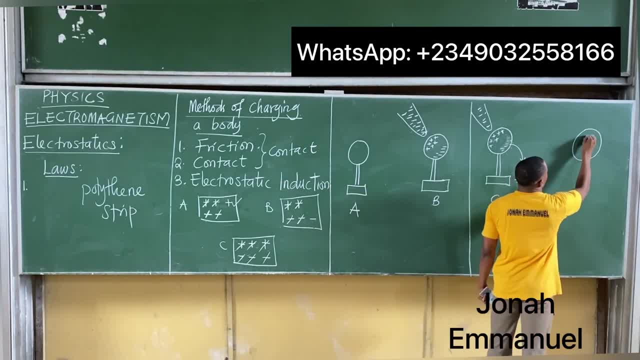 So these ones now will fall back here. Hence I'll be having only one, two, three, four, five, six Positively charged bodies, And I'm having this. So observe that I have converted this body from a neutral body to a positively charged. 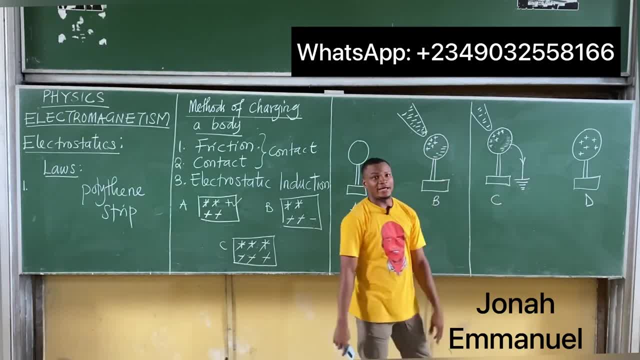 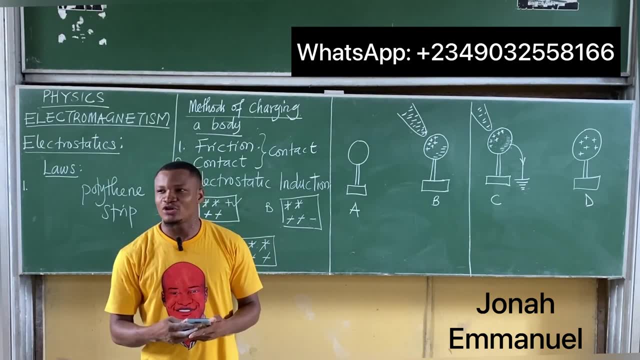 body without any contact. This is called electrostatic induction. That's it. Should I give you a note? Can you form the note? Which of them? All right, Can you give me a note please? Okay, So I'm having this. 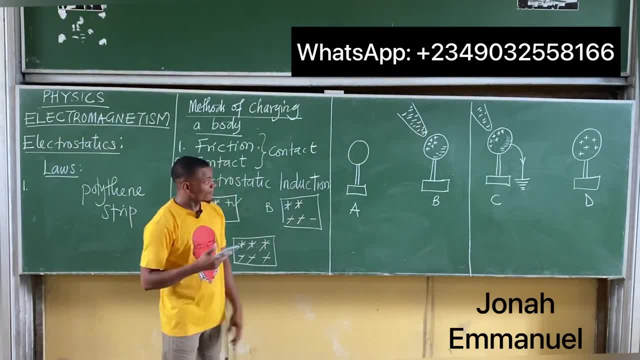 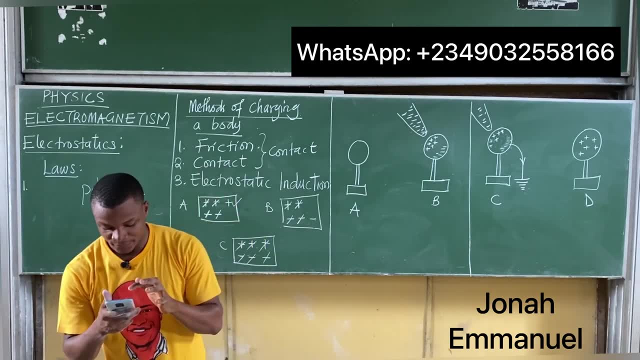 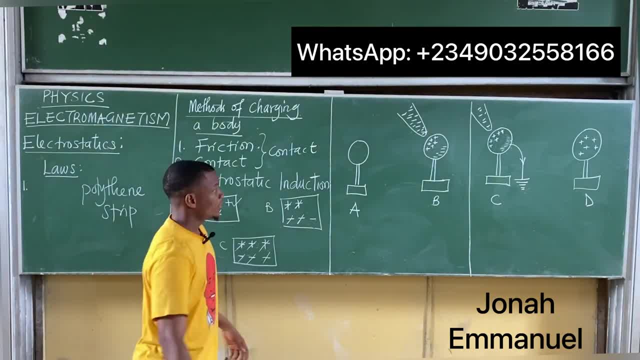 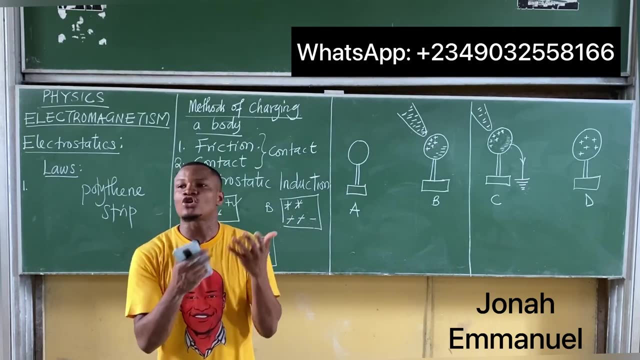 Electrostatic induction. Please Take down This. Have I given a definition already? Yeah, Yeah, You're great. Okay, Take down. Sure, Just add that As shown below. Just add that As shown below. I said this involves charging a neutral body by bringing it close to a charged body without. 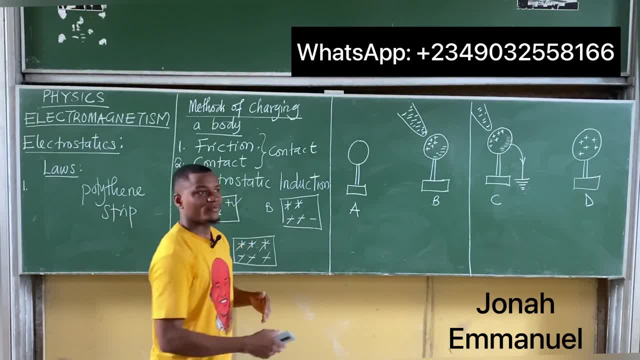 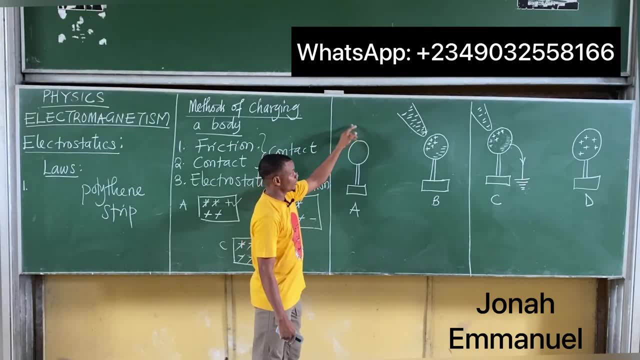 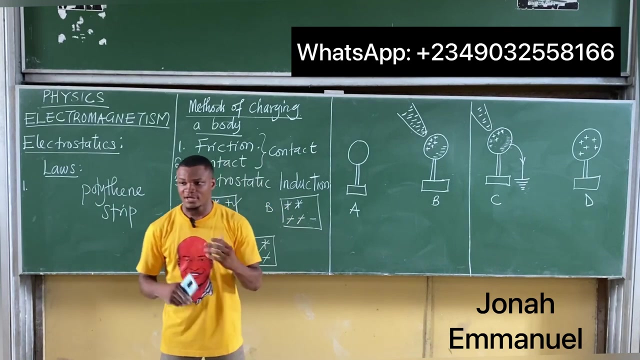 any contact. Now add that there are shown below: are shown below step one: step one: the neutral body. step one: the neutral body is given in a below sketch. this step one, the neutral body, is given in a below sketch. this, please, let's proceed. please, let's proceed. 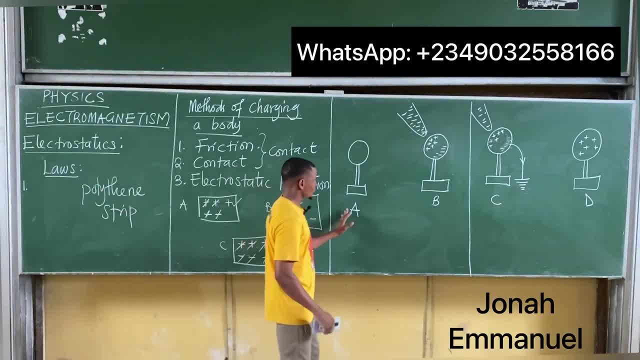 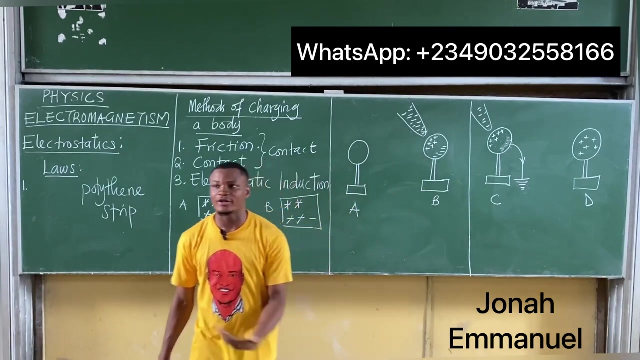 if you're done. step two: step two: a negatively charged rod. a negatively charged rod is brought close to the neutral body. step two: a negatively charged rod is brought close to the neutral body. step two: a negatively charged rod is brought close to the is brought close to the neutral body without any contact. 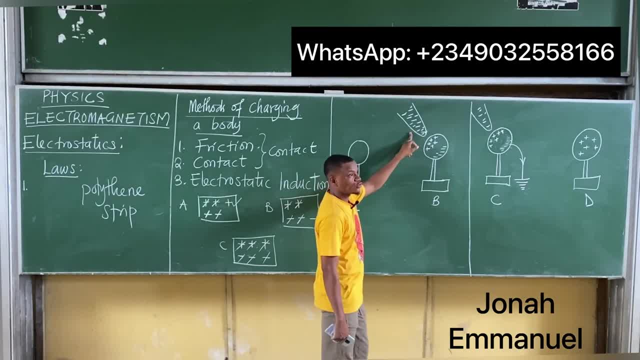 a negatively charged rod is brought close to the neutral body without any contact, such that the positive charges move close to. okay, move the wall. use your two words. use your two words such that such that the positive charges move towards the, the positive charges move towards the, the positive charges move towards the negatively charged rod. i experienced 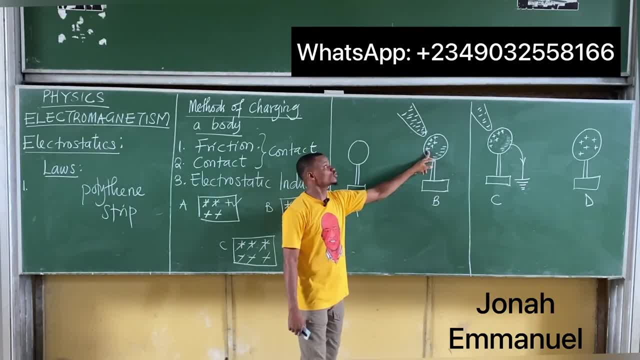 negatively charged rod. i experienced negatively charged rod, i experienced already, already, already, such that the positive charges moves, such that the positive charges moves, such that the positive charges moves towards the negatively charged rod, towards negatively charged rod and the towards negatively charged rod and the towards negatively charged rod and the negative charges moves. 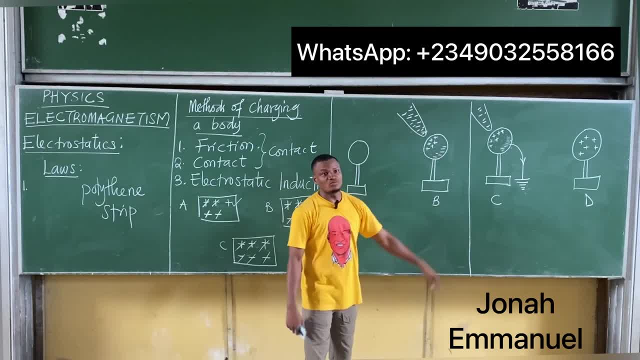 negative charges moves. negative charges moves against and the negative charges moves against and the negative charges moves against and the negative charges moves against, against and the negative charges moves against, against and the negative charges moves against the negatively charged rod, the negatively charged rod, the negatively charged rod and the negative charges moves against. 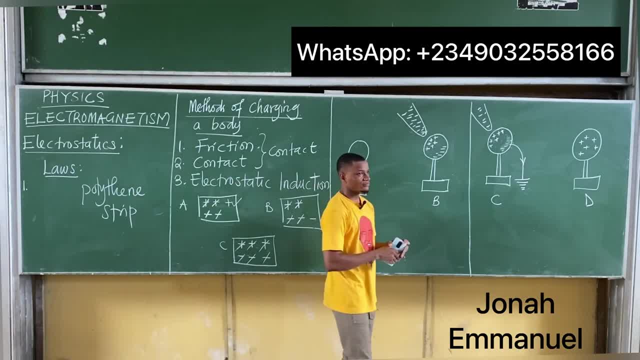 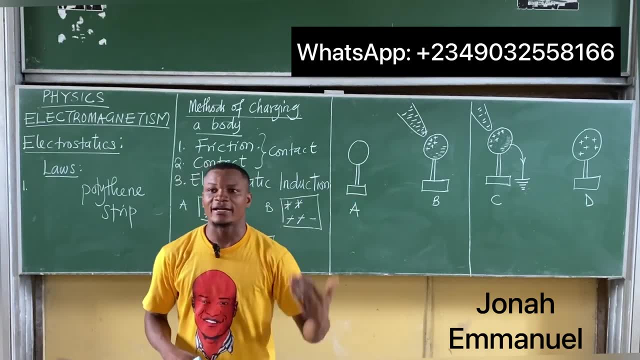 and the negative charges moves against. and the negative charges moves against the negatively charged rod. according to which law? in brackets? according to the first law of in brackets. according to the first law of in brackets. according to the first law of electrostatics: close the brackets. electrostatics: close the brackets. 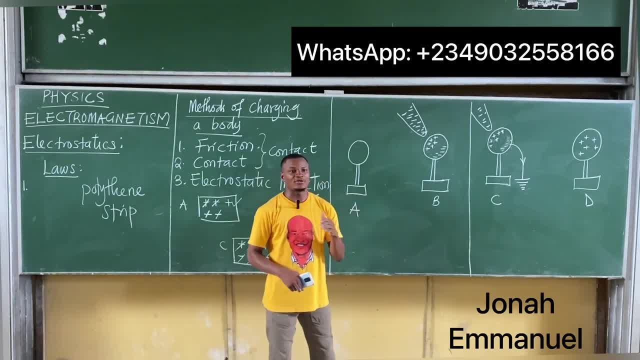 electrostatics. close the brackets according to the first law of. according to the first law of. according to the first law of: electrostatics. close the bracket. electrostatics. close the bracket. electrostatics. close the bracket as shown in b below. you can now sketch. 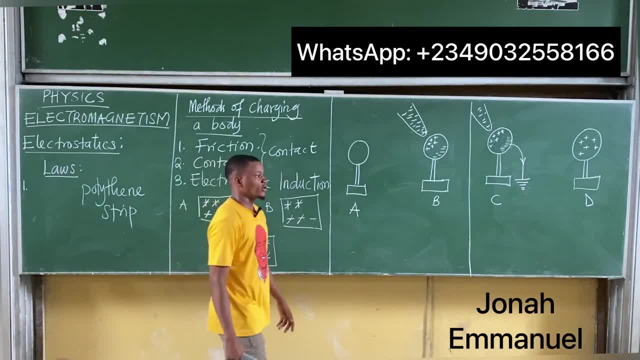 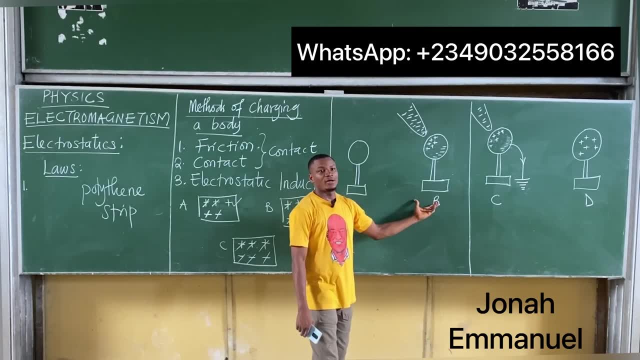 as shown in b below. you can now sketch. as shown in b below. you can now sketch this: this: this according to: according to: according to the second law, the second law, the second law, according to what the first law of. according to what the first law of, according to what the first law of electrostatics are shown in b. 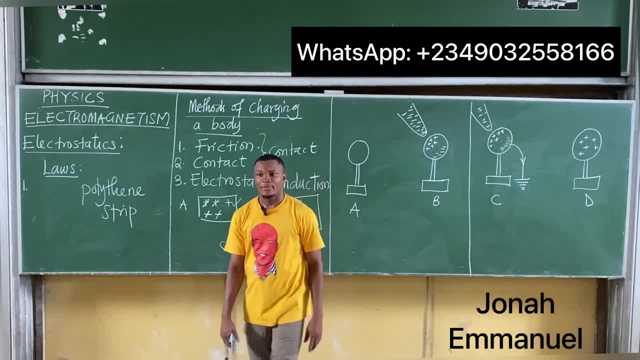 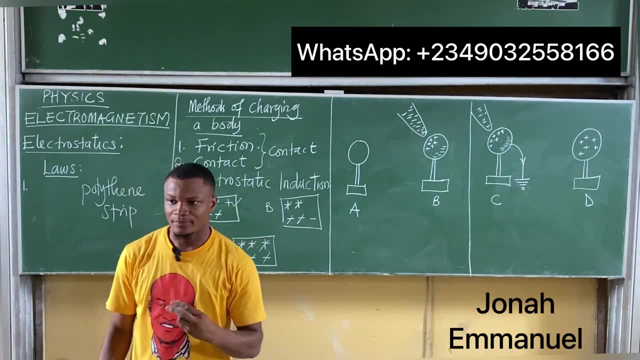 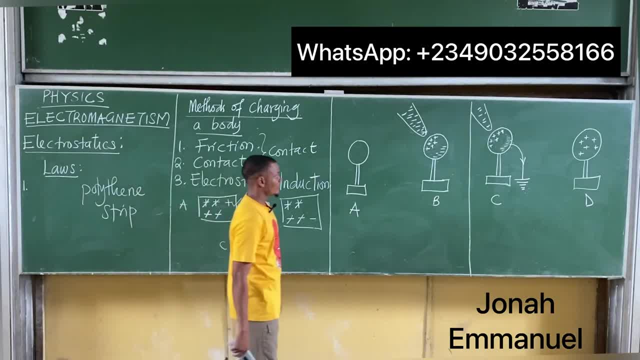 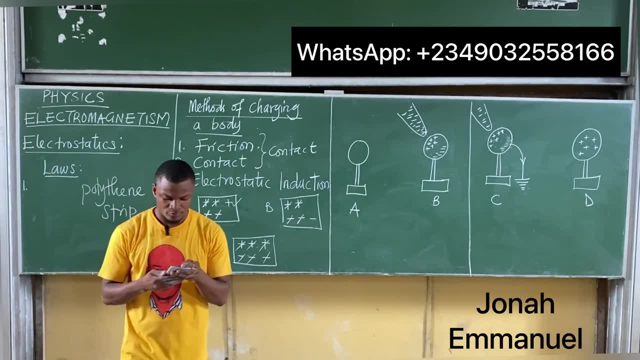 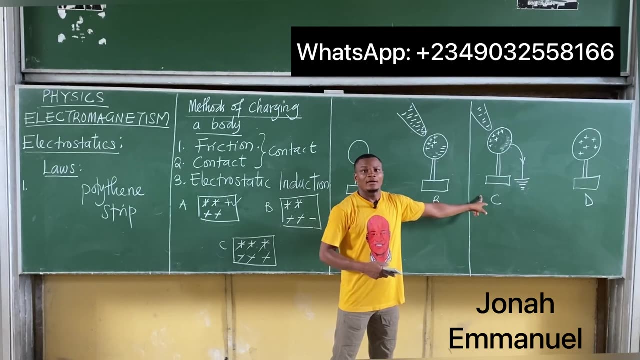 please catch bill, let's move on, please. please catch bill, let's move on, please. step three: please catch bill, let's proceed, please step. please. step three, step three. add the path. step three: x e a r 2 h. how add the path step three: x e a r 2 h. how. 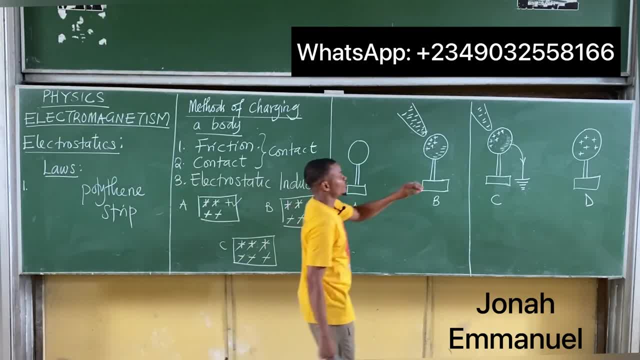 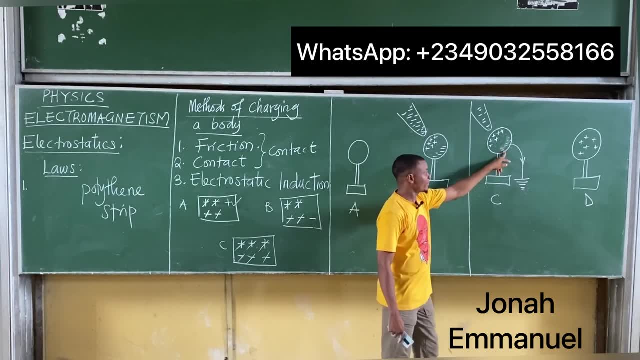 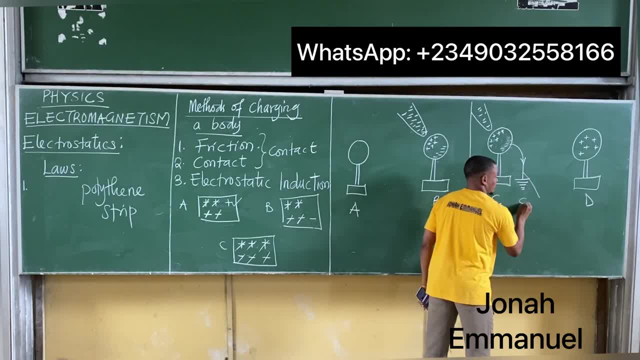 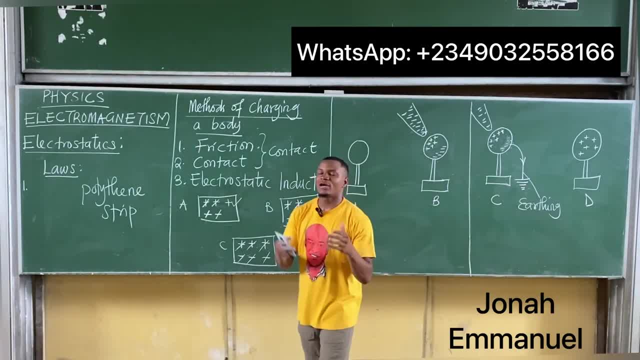 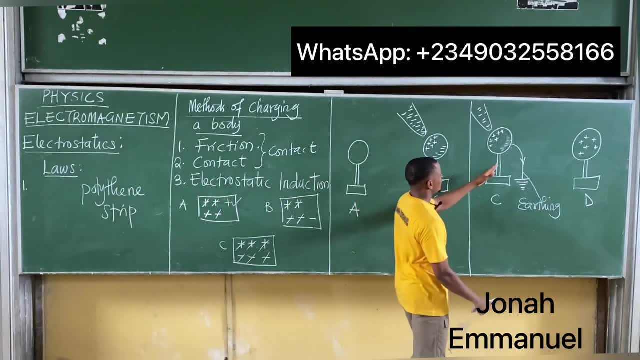 that's the path of the neutral body. that's the path of the neutral body. that's the path of the neutral body, of the neutral body, having the negative of the neutral body, having the negative of the neutral body. having the negative charges, charges, charges. having the negative charges. 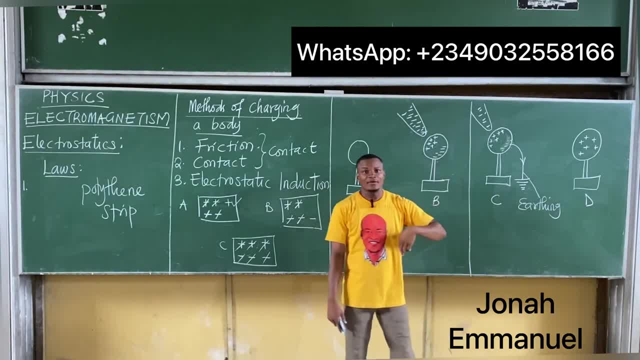 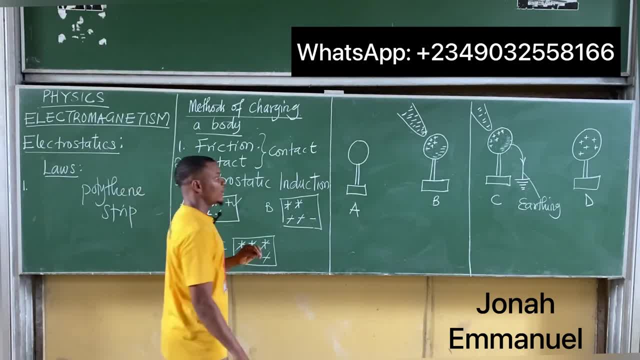 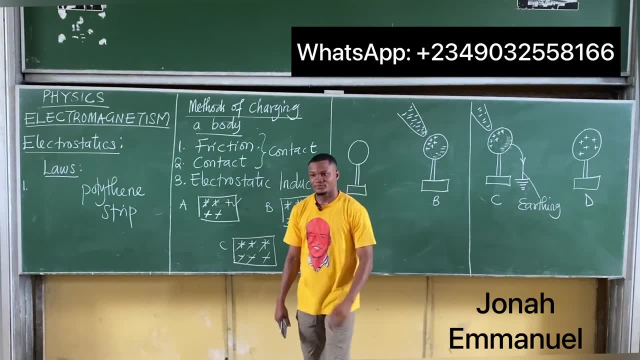 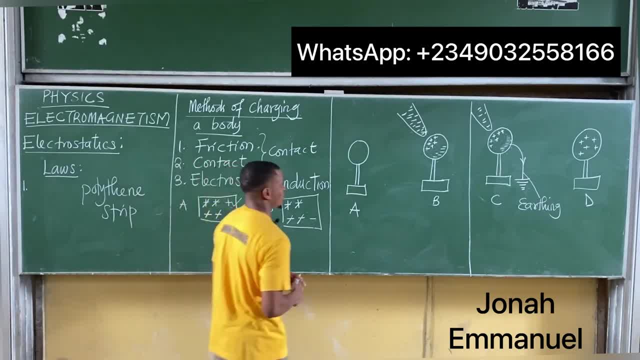 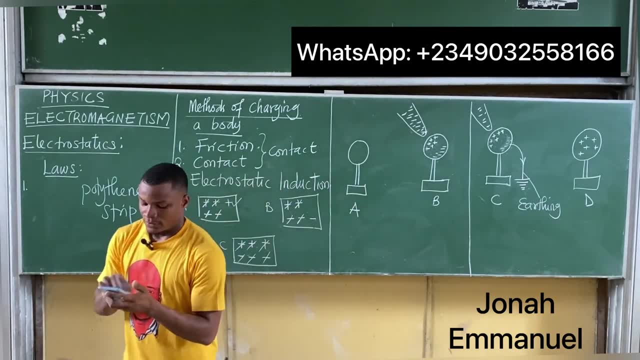 you can now sketch this one, such that you can now sketch this one, such that they flow into the earth. they flow into the earth. they flow into the earth. are shown in c. you can now sketch. are shown in c. you can now sketch. are shown in c. you can now sketch this one. 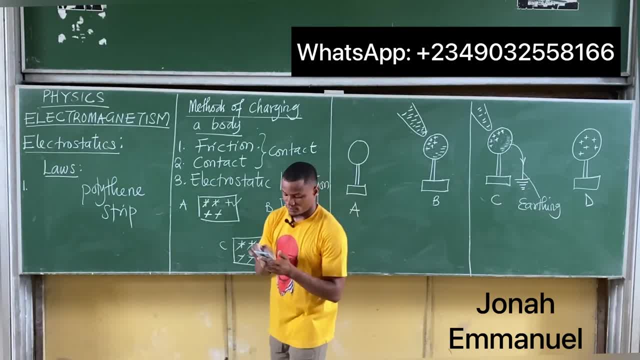 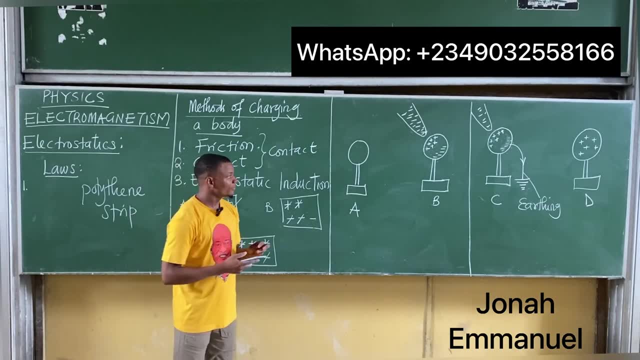 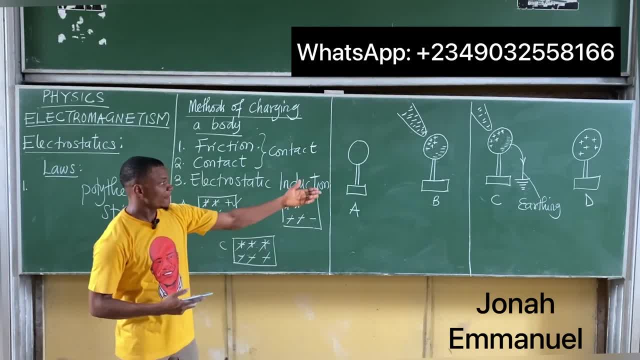 so please understand the process of. so please understand the process of electrostatic induction. know how it electrostatic induction. know how it electrostatic induction. know how it works right, works right, works right. know how it works. know how it works. know how it works. if you're done, please step four. finally, 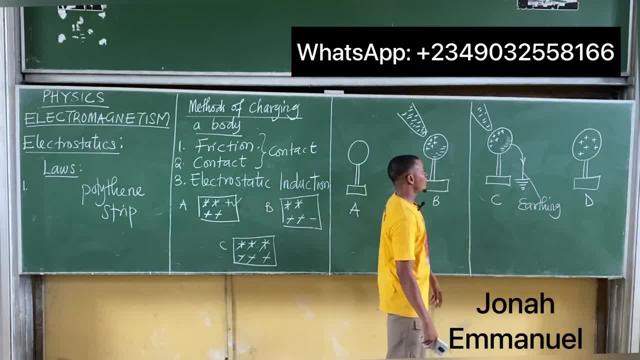 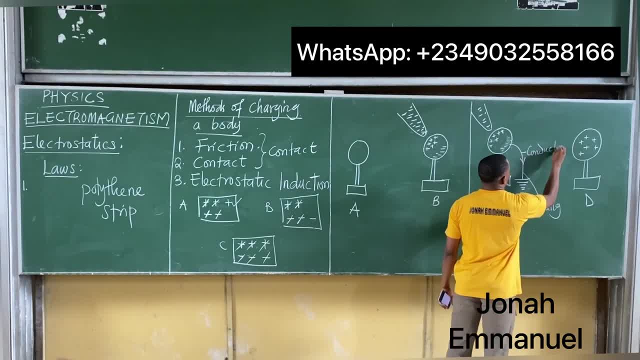 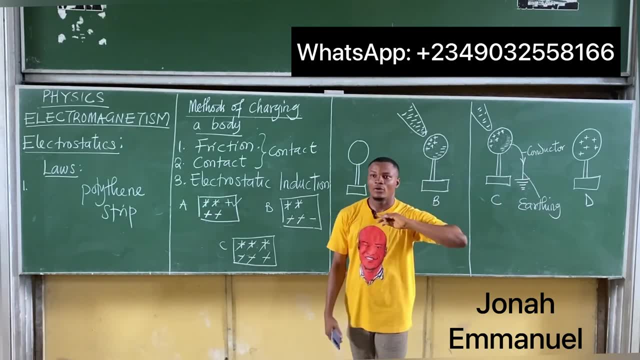 take off the negatively charged rod, because here has to be a conductor, here has to be a conductor, here has to be a conductor, it has to be a conductor. take off the negatively charged rod. and take off the negatively charged rod. and take off the negatively charged rod and the conductor. 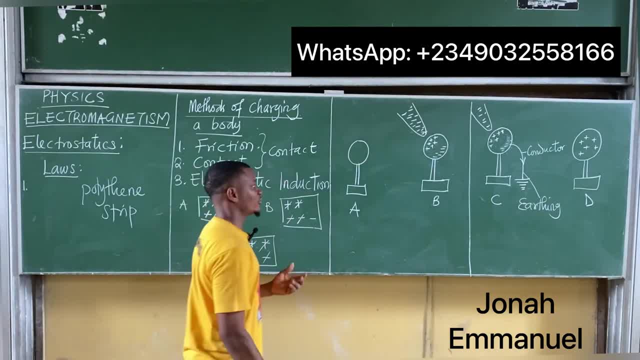 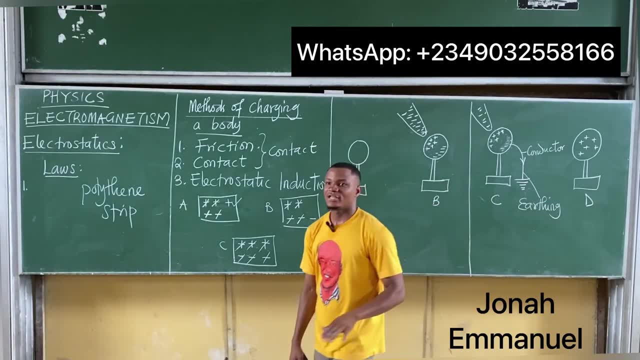 the conductor, the conductor, take off the negatively charged rod and take off the negatively charged rod and take off the negatively charged rod and the conductor, the conductor, the conductor, such that the neutral body becomes such that the neutral body becomes such that the neutral body becomes positively charged, as shown. 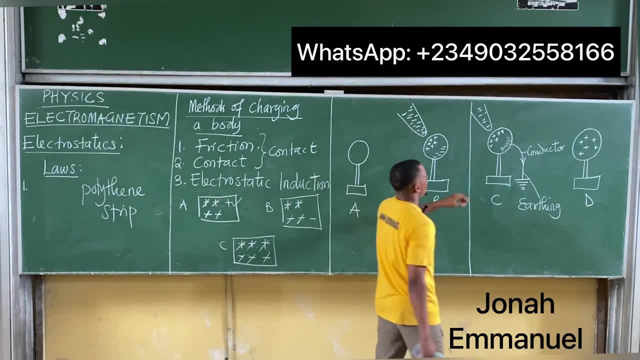 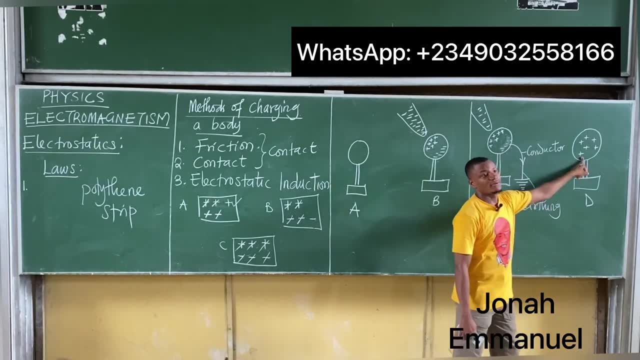 positively charged as shown. positively charged as shown below step four. below step four. below step four: take off the negatively charged rod. take off the negatively charged rod. take off the negatively charged rod and the and the and the conductor such that the neutral body. conductor, such that the neutral body. 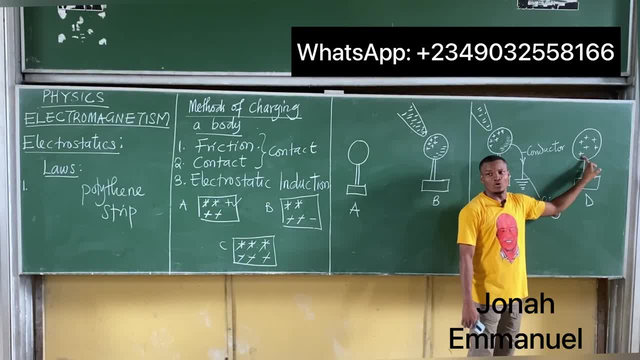 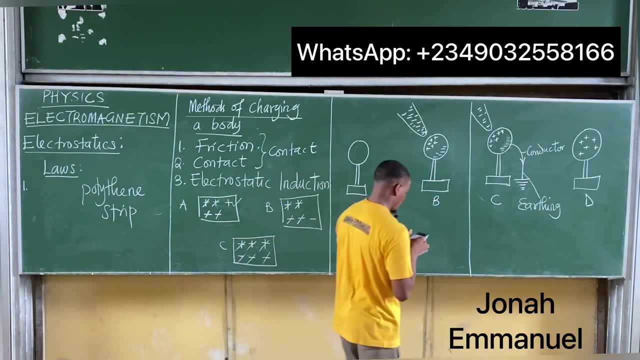 conductor, such that the neutral body becomes positively charged, as shown, becomes positively charged as shown, becomes positively charged as shown below. please catch this and below. please catch this and below. please catch this and we are done, please. all right. so i believe that stuff is all right. so i believe that stuff is. 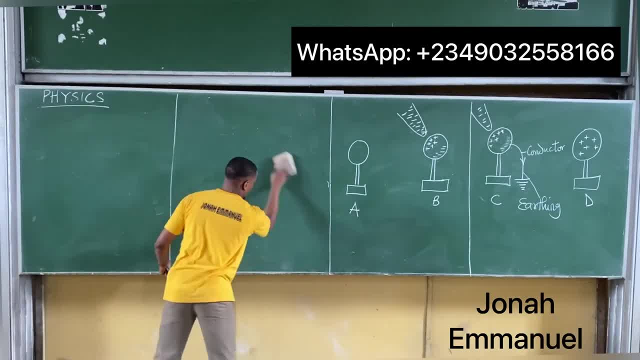 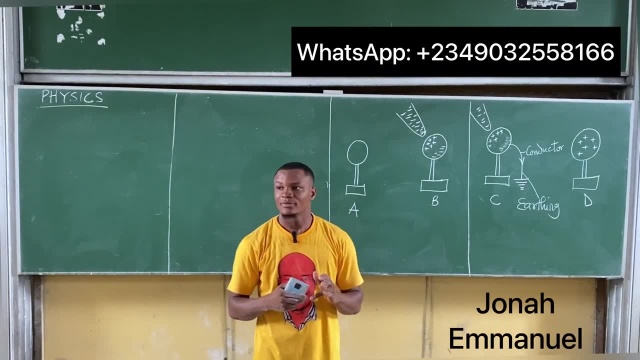 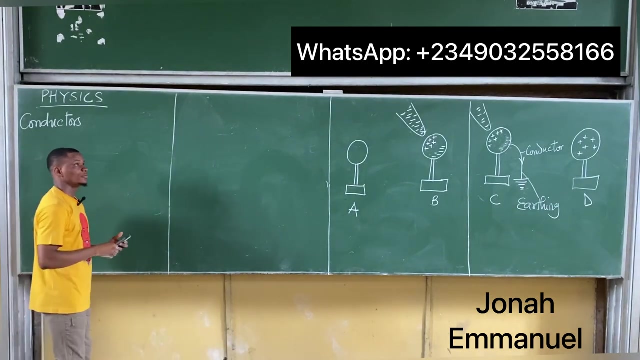 all right. so i believe that stuff is clear: take down, please stop heading. take down, please stop heading, please take down, please stop heading, please take down, please stop heading please. so, so, so all right. so many please: conductors, semiconductors, insulators and superconductors, please. 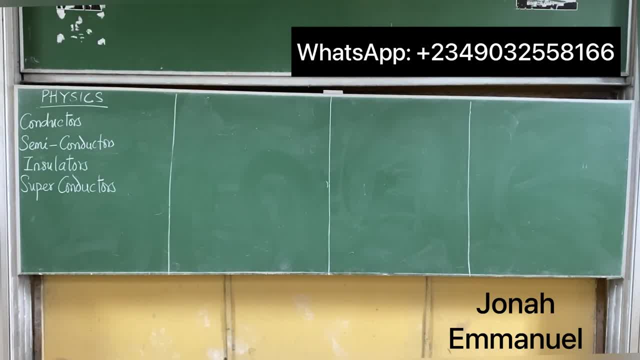 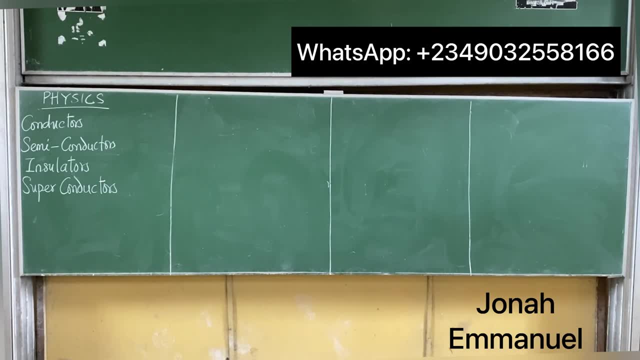 what are conductors? conductors, semiconductors, insulators and superconductors. superconductors, right. conductors are materials that allow the flow of electrical charges. electric charges, that's it. conductors are materials that allow the flow of electrical charges, that's it. conductors are materials that 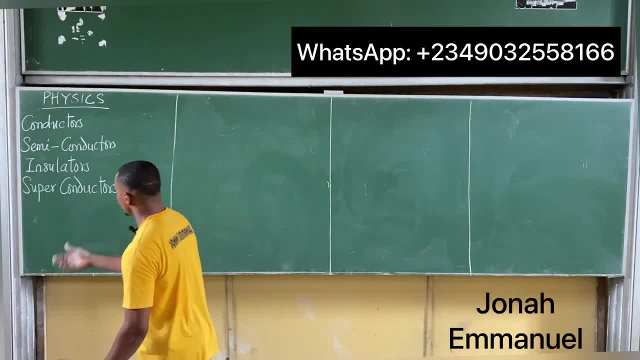 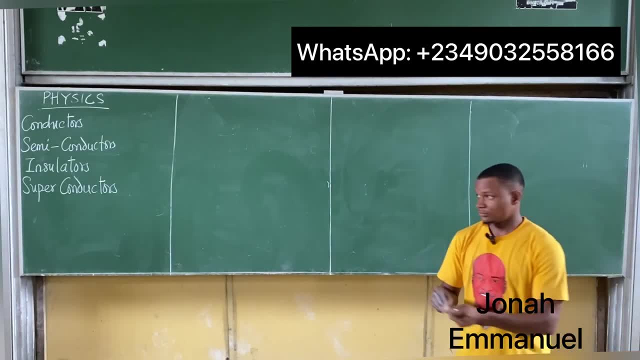 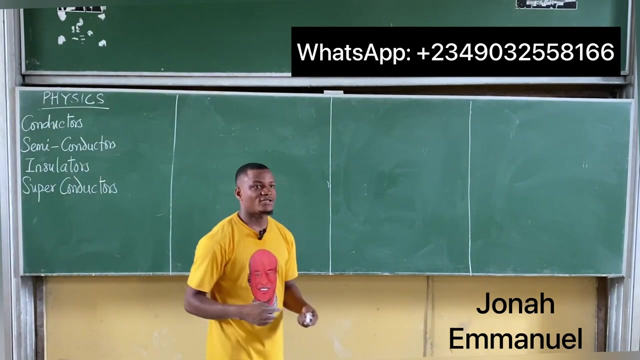 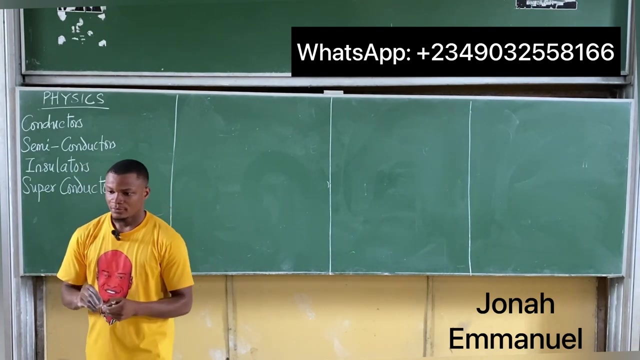 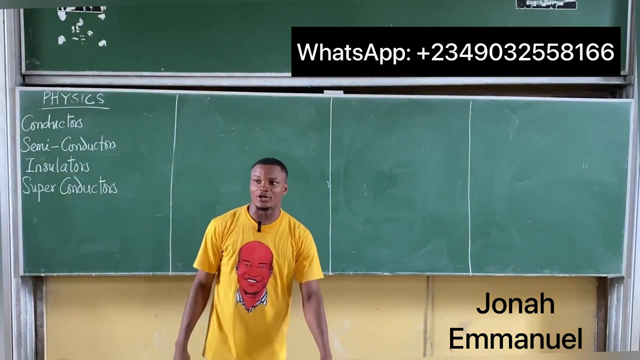 conductors are materials that allow the flow of electrical charges. let's look at insulators. keep semi impending. insulators are materials that do not allow the flow of electrical charges. insulators: insulators are materials that do not allow the flow of electrical charges. next, please, semiconductors. 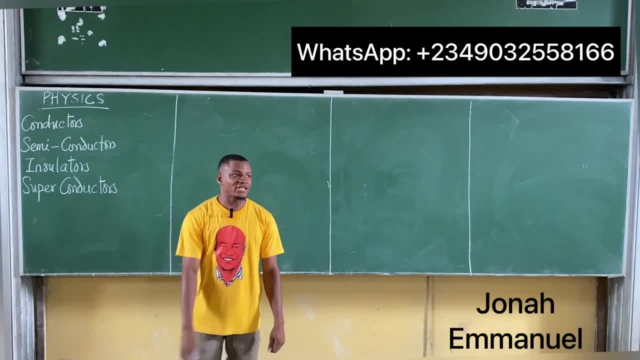 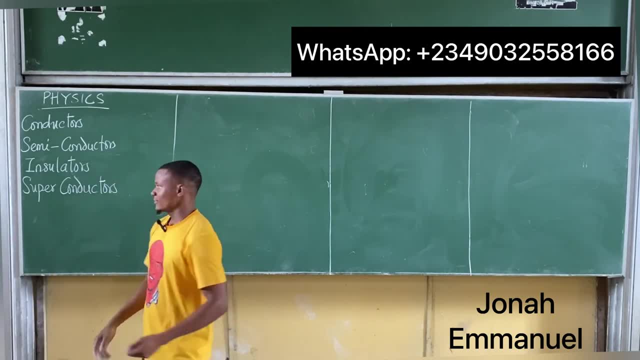 semiconductors. next, please, semiconductors. these are materials which in their pure state do not conduct electricity. right, this is called a semi, not a semi semi semiconductors. these are materials which in their pure state do not conduct electricity, electric charges, but become superconductors. 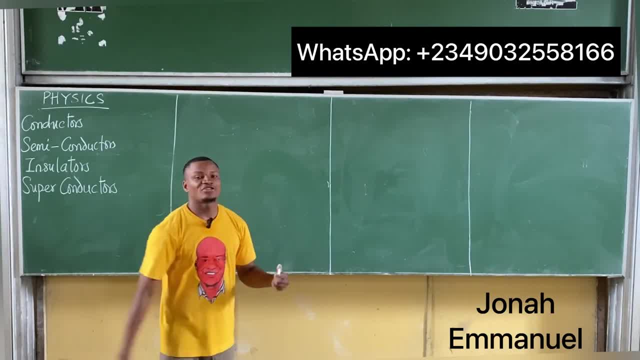 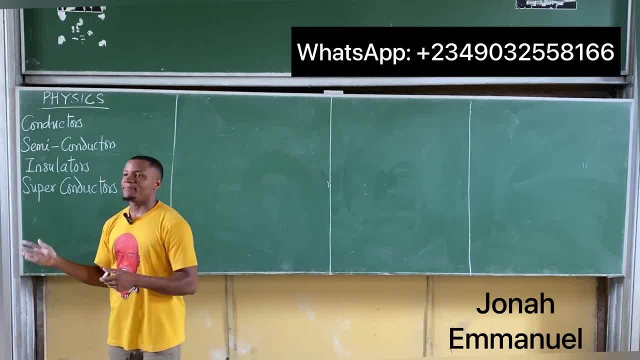 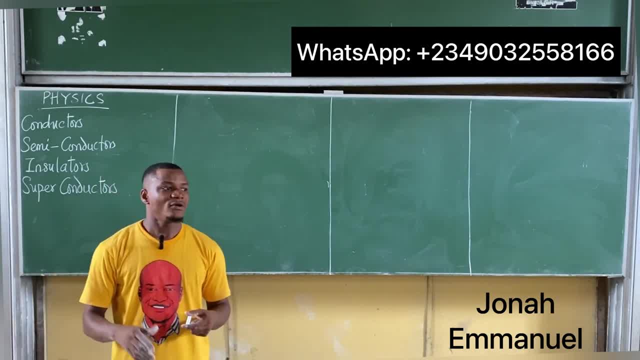 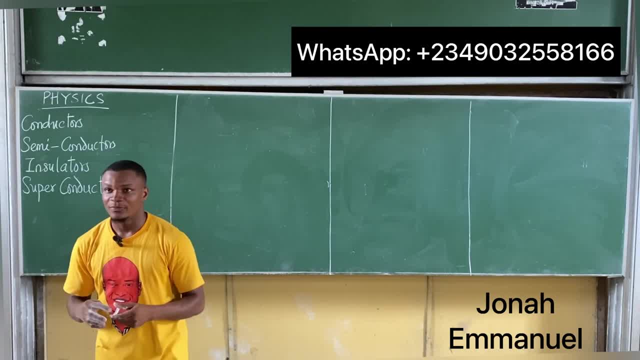 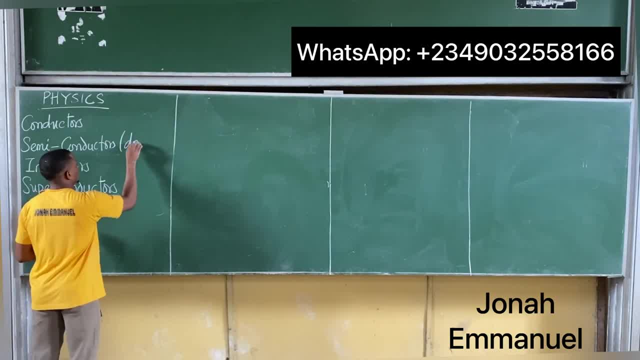 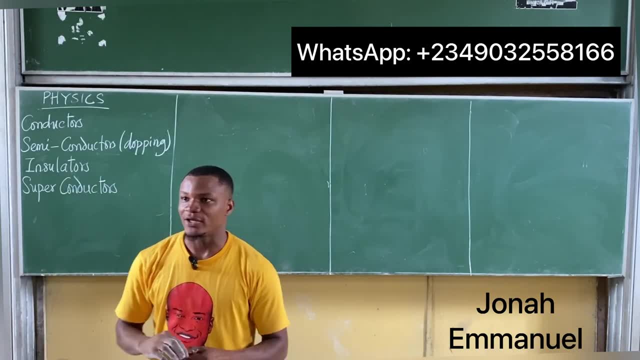 through a process called doping, through a process called doping, through a process called doping, through a process called, through a process called doping, through a process called doping, doping, doping, doping, called doping. what's doping? doping is a called doping. what's doping, what's doping? doping is a. 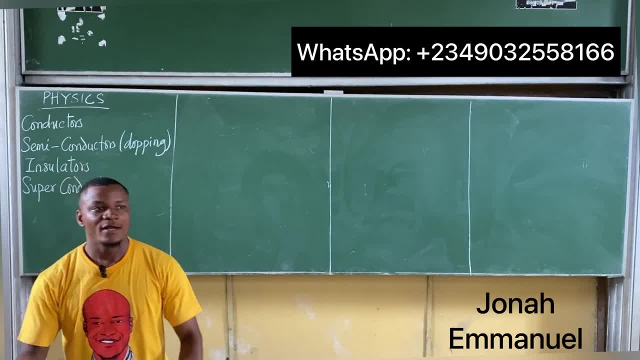 called doping. what's doping? what's doping? doping is a process of adding an impurity to order. process of adding an impurity to order. process of adding an impurity to order to a semi-conductors to move them from. to a semi-conductors to move them from. 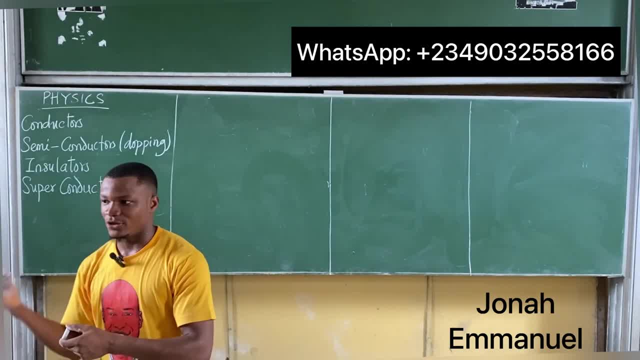 to a semi-conductors to move them from what they're insulators to what? what they're insulators to what? what they're insulators to what conductors? it's called doping. finally, conductors, it's called doping. finally, conductors, it's called doping. finally, please, superconductors. 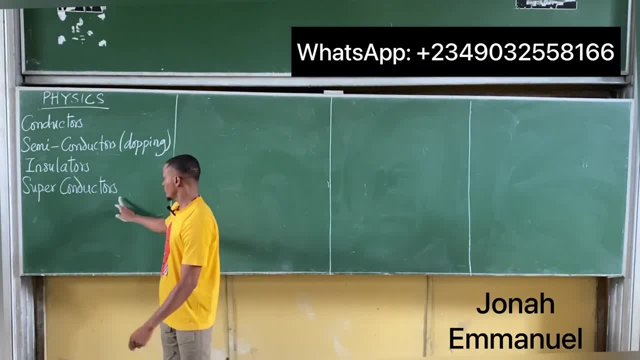 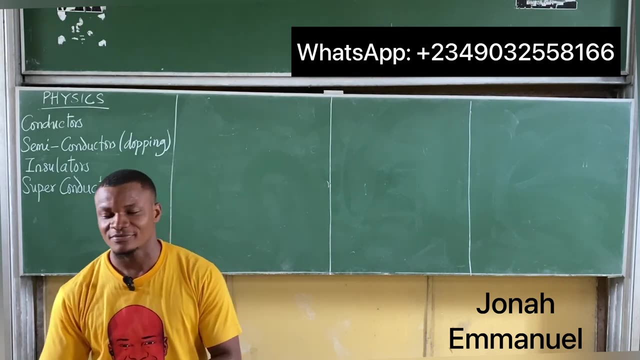 please, superconductors, please superconductors, finally, please, superconductors, finally, please superconductors. these are materials, that these are materials, that these are materials that does not, does not, does not, or material material do not, do not, or material material do not, do not, or material material do not do not. these are materials that do not. 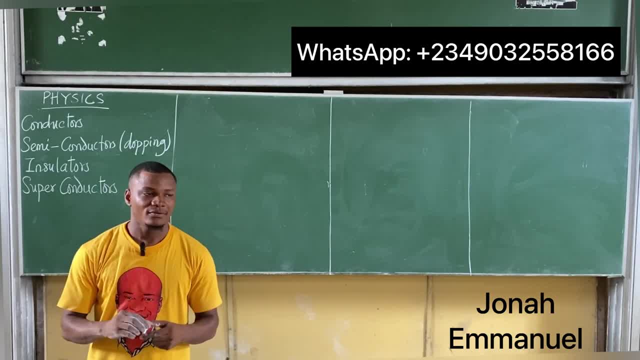 these are materials that do not do not. these are materials that do not have have have any form of resistance, any form of resistance, any form of resistance. these are materials that do not have any. these are materials that do not have any. these are materials that do not have any form of. 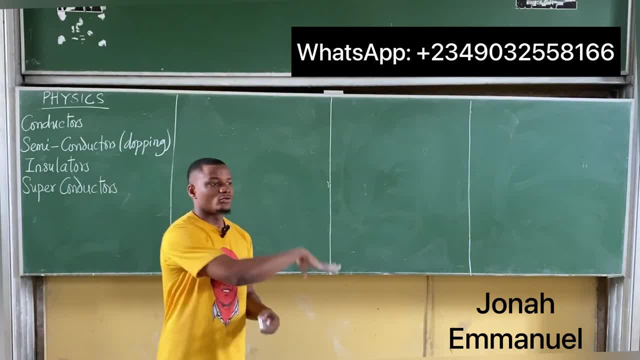 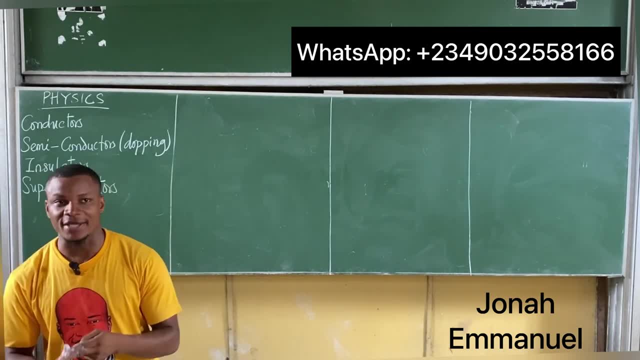 form of form of resistance, any form of resistance, any form of resistance, any form of resistance to the flow, to the flow, to the flow, or or or passage of passage, of passage of electrical charges. electrical charges, electrical charges. these are, these are materials that do. these are, these are materials that do. 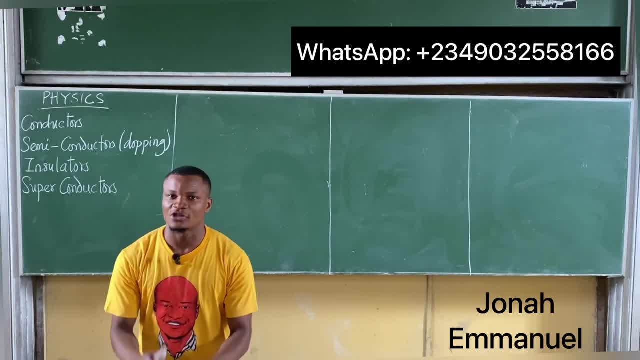 these are? these are materials that do not have any form of not have any form of not have any form of opposition or resistance, opposition or resistance, opposition or resistance to the to the to the flow or passage of electrical charges. to the flow or passage of electrical charges. 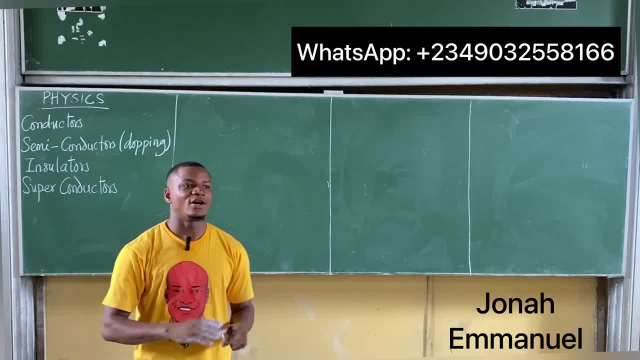 to the flow or passage of electrical charges, the flow or the passage or the movement of the flow or the passage or the movement of the flow or the passage or the movement of electrical charges. few example electrical charges. few example electrical charges. few example conductors. an example: copper. 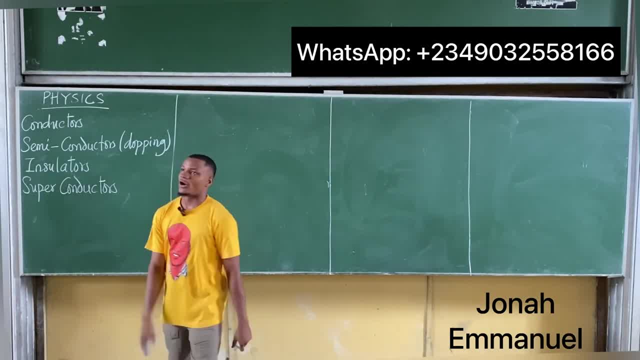 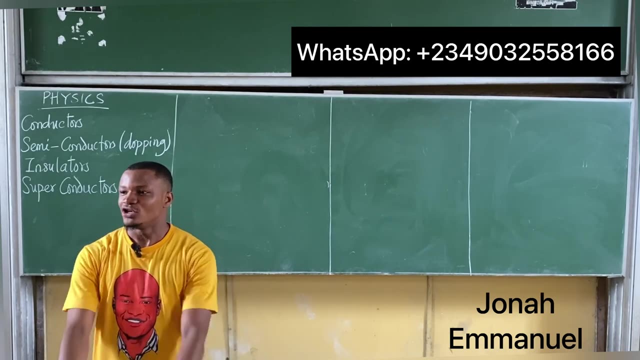 conductors. an example copper conductors. an example: copper ion atc semiconductor- ion atc semiconductor, ion atc semiconductor: um silicon, um silicon, um silicon. right example here. right example here. right example here: silicon insulator- dry wood insulator, dry wood insulator, dry wood, dry wood. you know what i'm using: dry wood. 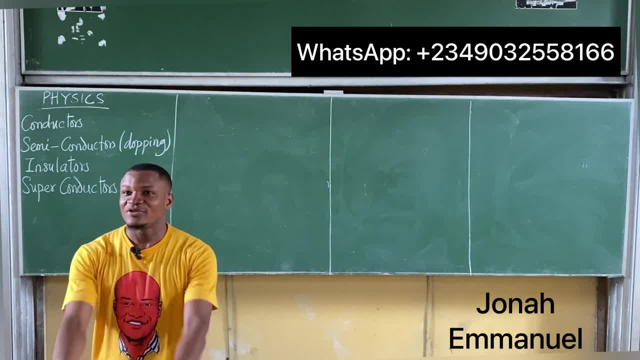 dry wood. you know what i'm using? dry wood, dry wood. you know what i'm using? dry wood, what is dry wood? what is dry wood? what is dry wood? because that is the first that comes to, because that is the first that comes to, because that is the first that comes to mind when somebody's been executed. 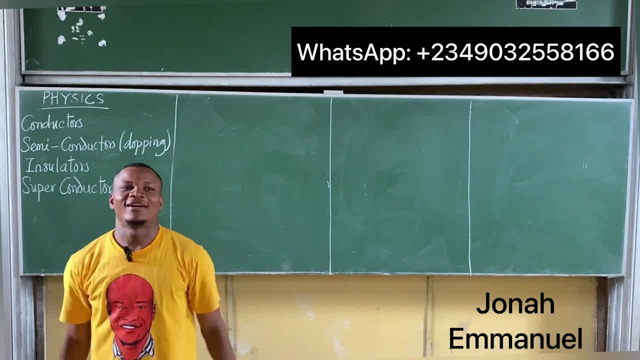 mind when somebody's been executed. mind when somebody's been executed two by two. plug him down, two by two. plug him down, two by two. plug him down. so now i'm using dry wood, please, so it's. so now i'm using dry wood, please, so it's. 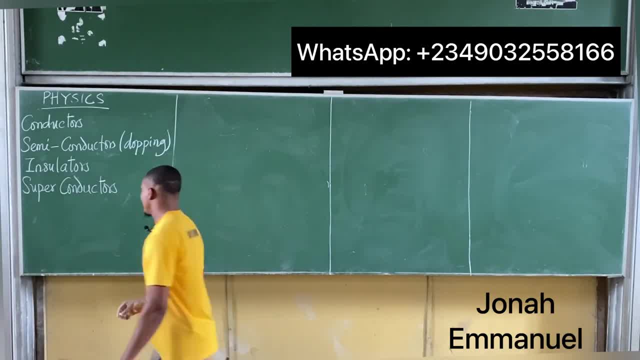 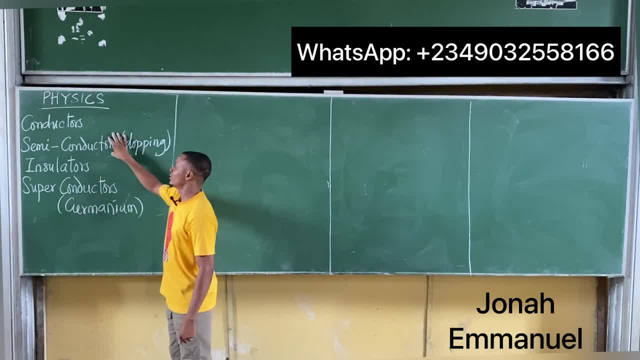 all right. so germanium or superconductors, all right. so germanium or superconductors. it's little isn't dry wood semi. it's little isn't dry wood semi. it's little isn't dry wood semi. conductor using silicon and then conductor using silicon and then. 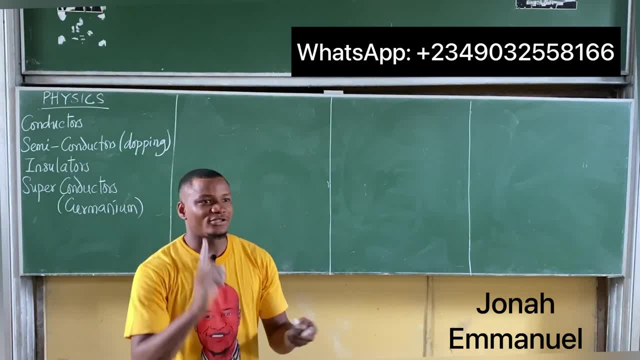 conductor using silicon. and then conductor. we said anything you want to conductor. we said anything you want to conductor. we said anything you want to uh iron copper, etc, etc, etc. so done with uh iron copper, etc, etc, etc. so done with uh iron copper, etc. etc, etc. so done with this. let's move on again. 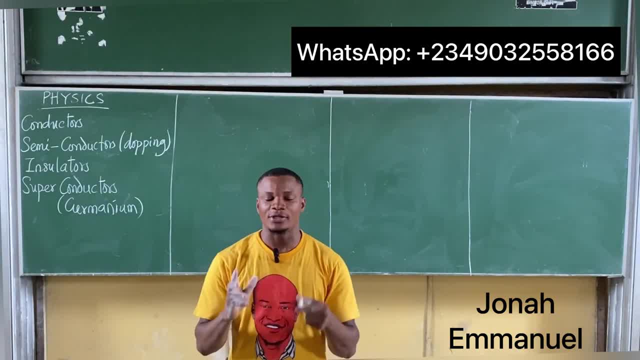 this, let's move on again. this, let's move on again. one more thing. um, we were looking at one more thing, um, we were looking at one more thing. um, we were looking at what's it called the? what's it called the? what's it called the laws of electrostatics. we've done the. 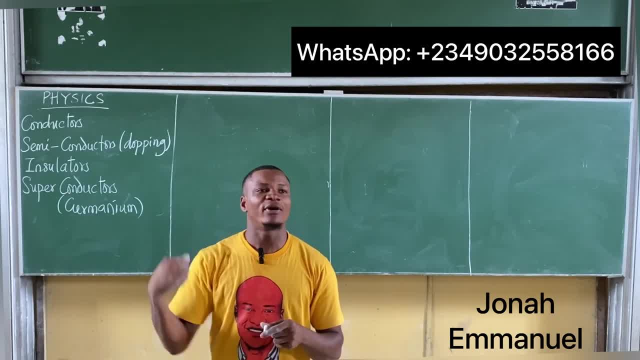 laws of electrostatics. we've done the laws of electrostatics. we've done the first law. we'll do second law, but first law. we'll do second law, but first law. we'll do second law, but before then we'll take one more thing. before then we'll take one more thing. 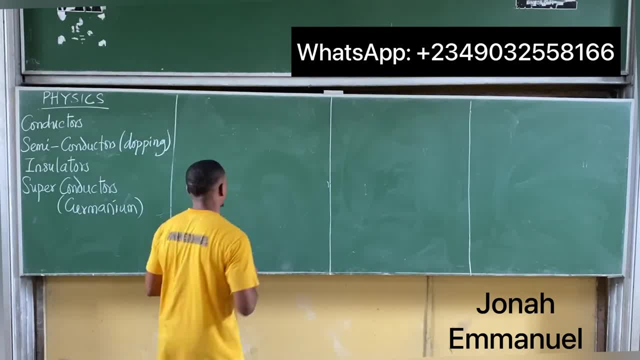 before then we'll take one more thing. we'll take a past question and then we'll we'll take a past question and then we'll we'll take a past question and then we'll proceed. please take that, please proceed. please take that, please proceed. please take that. please charge quantization. 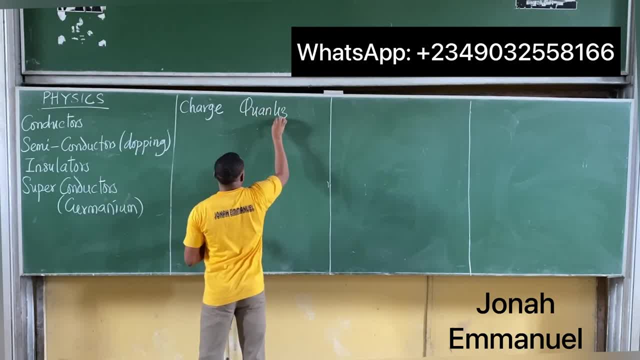 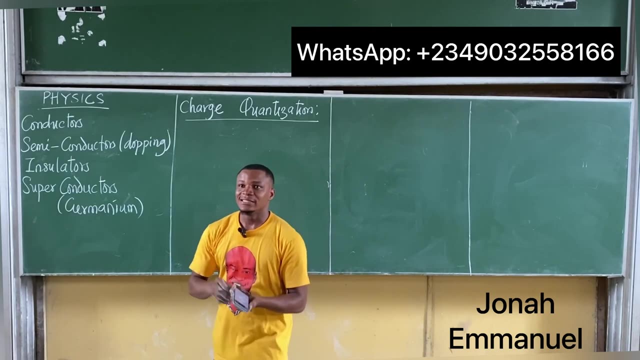 charge, charge, charge, quantization, charge quantization. this is the material charge quantization. this is the material charge quantization. this is the material past question. these are in sciences past question. these are in sciences past question. these are in sciences, um, um, um come out of your past question. 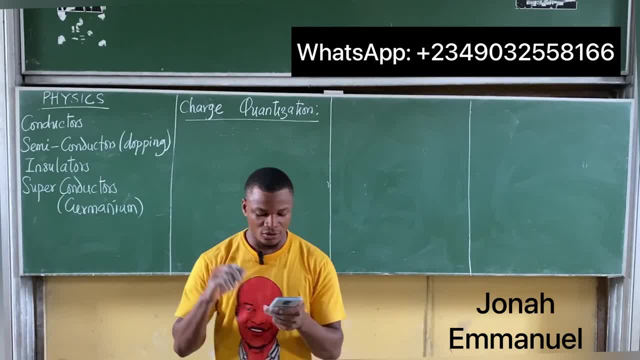 come out of your past question. come out of your past question. they will say: they will say: they will say: set questions on it, but i'll give you set questions on it. but i'll give you set questions on it, but i'll give you just a brief definition. i'll give you. 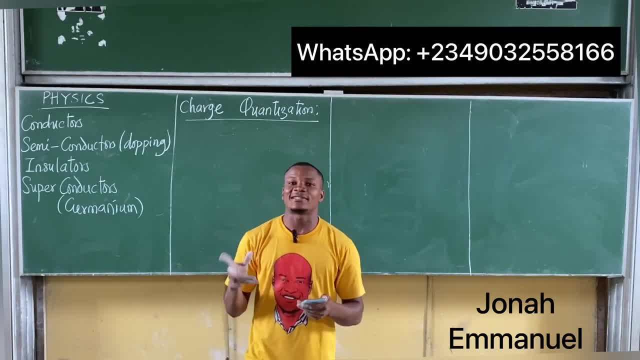 just a brief definition. i'll give you just a brief definition. i'll give you something and then proceed. please take something and then proceed. please take something and then proceed. please take that, please, that, please, that, please. charge. quantization means charge. charge. quantization means charge. charge quantization means charge. quantization means that. 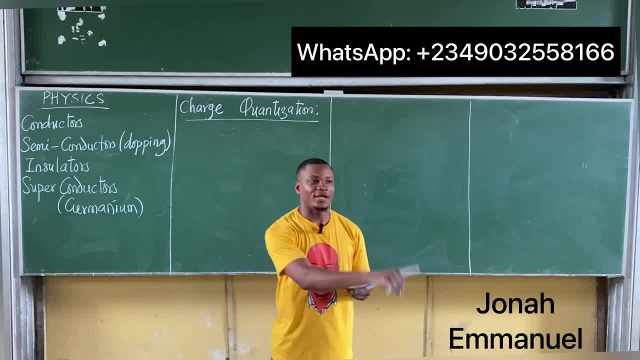 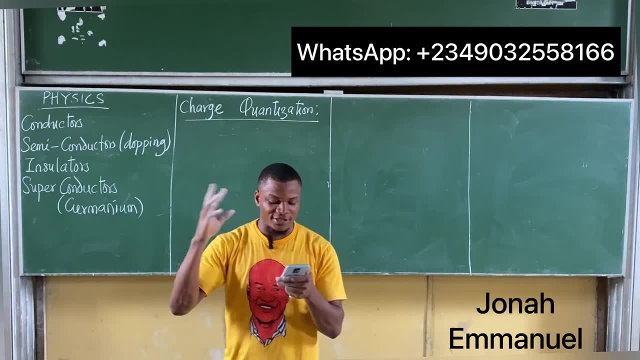 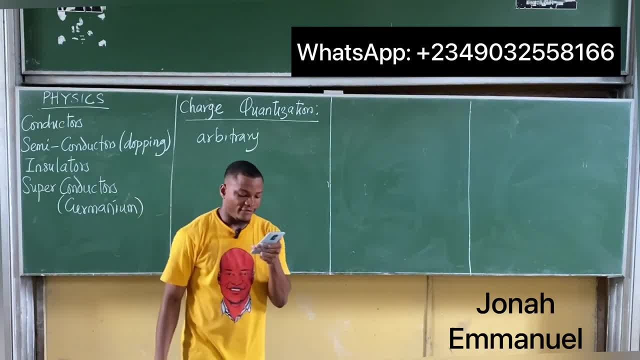 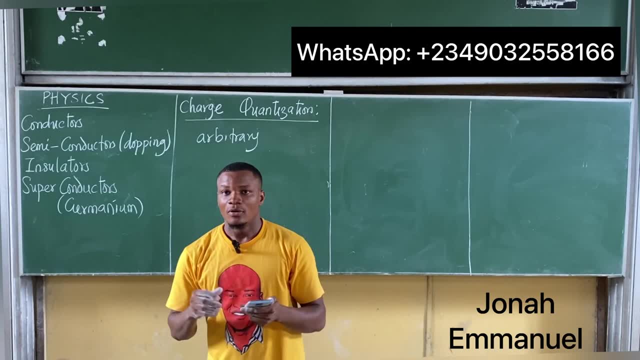 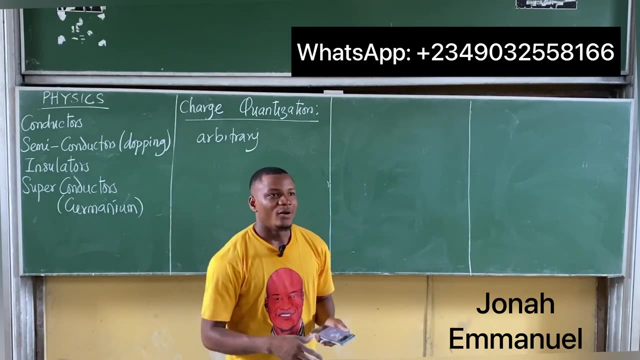 arbitrarily, arbitrarily, arbitrarily, arbitrarily, arbitrarily, arbitrarily, arbitrarily. values, values, values cannot take any arbitrary values, but only values that are, but only values that are, but only values that are integral multiples. but only values that are, but only values that are, but only values that are integral multiples. integral multiples. 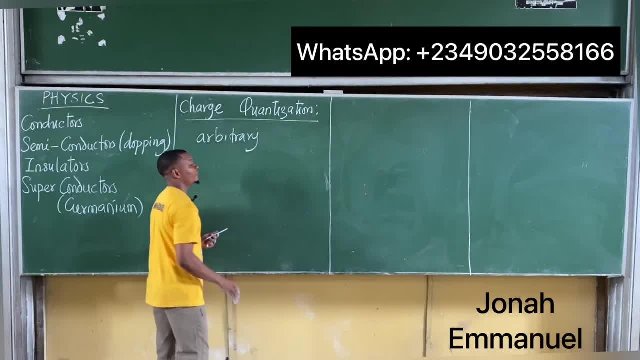 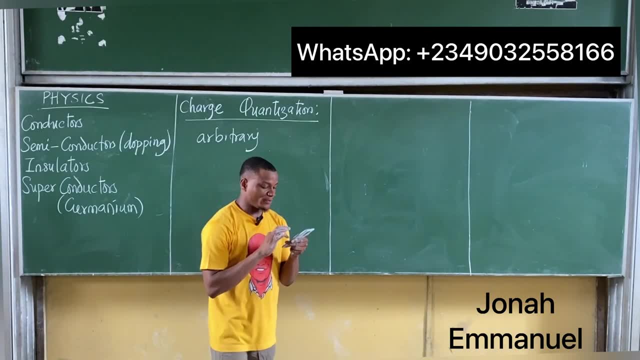 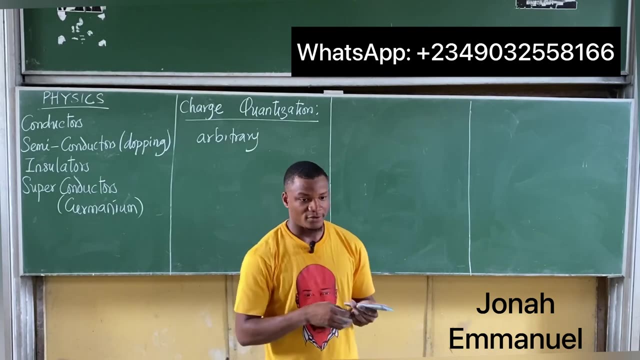 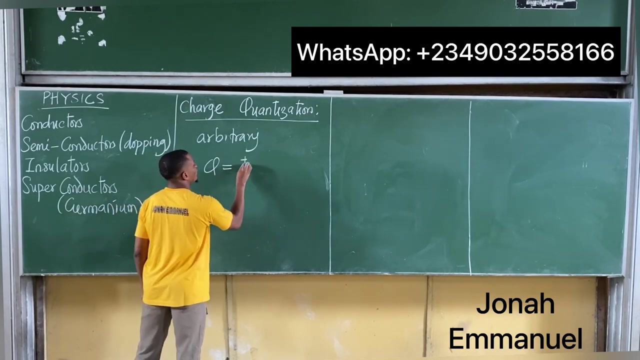 integral multiples that are integral multiples of that are integral multiples of that are integral multiples of the fundamental charge, the fundamental charge, the fundamental charge. integral multiples of the fundamental charge, the fundamental charge, the fundamental charge, full stop. it is given by the formula q equal to plus or. 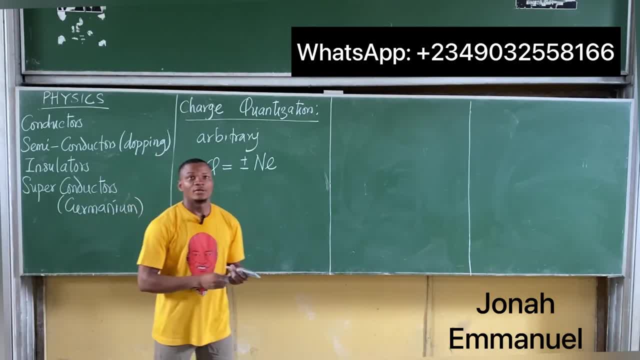 it is given by the formula q equal to plus or it is given by the formula q equal to plus or minus, minus, minus and e. it is given by the value q and e. it is given by the value q and e. it is given by the value q equal to plus or minus. and please note the 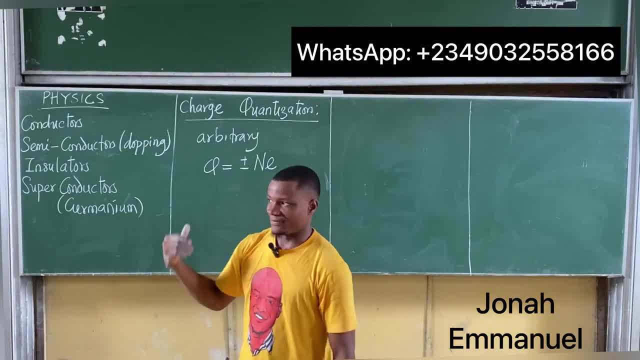 equal to plus or minus and please note the equal to plus or minus. and please note the stuff. please notice formula, please. probably stuff. please notice formula. please, probably stuff. please notice formula, please. probably really either your test or your exam. really either your test or your exam. really either your test or your exam. this is in science, is especially notice. 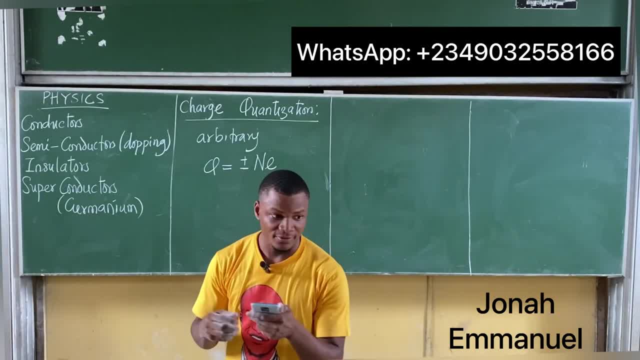 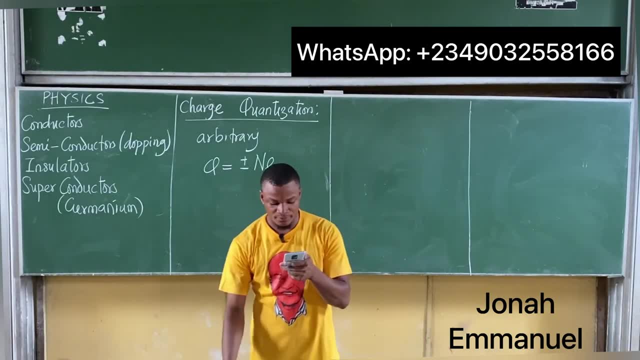 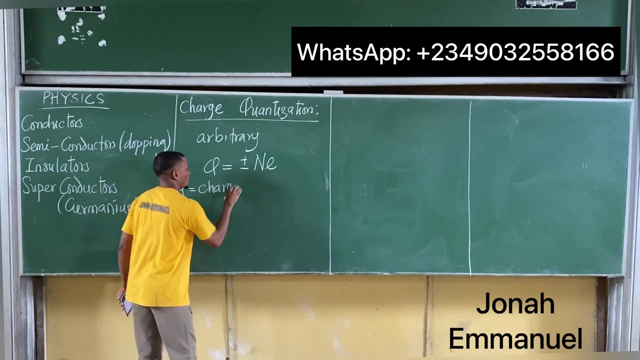 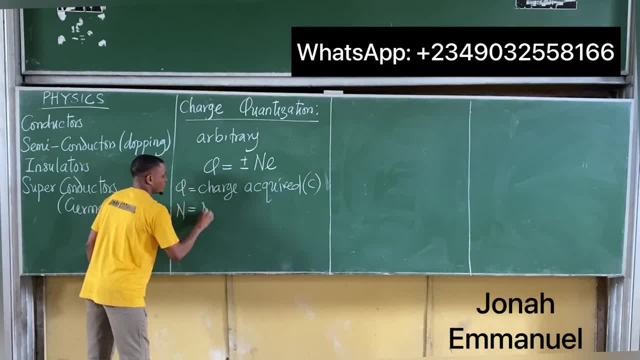 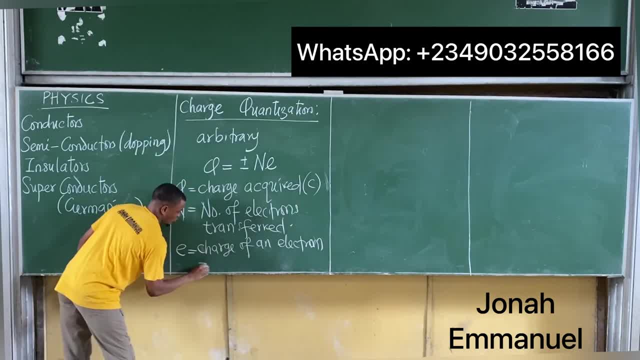 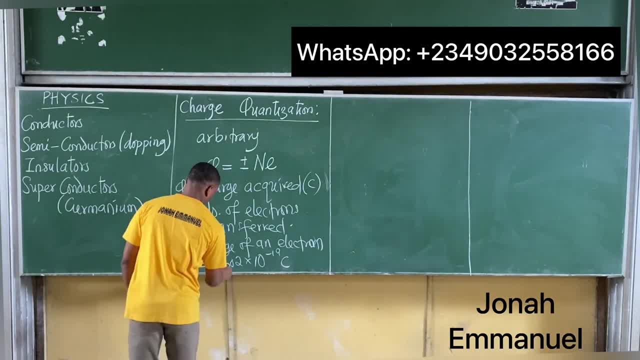 minus 19 column. minus 19 column, that's a charge of an electron. this one that's a charge of an electron. this one: that's a charge of an electron. this one here. some authors will say use negative here. some authors will say use negative here. some authors will say use negative here. so i will say: leave out the negative. 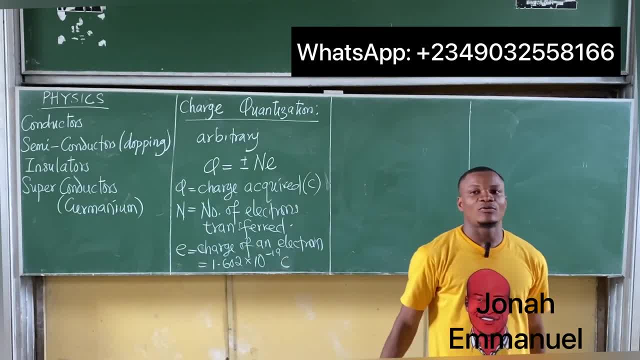 here. so i will say: leave out the negative here. so i will say: leave out the negative. when they say he's negative there, it's. when they say he's negative there, it's. when they say he's negative there, it's just because, just because, just because electrons are what they're negatively. 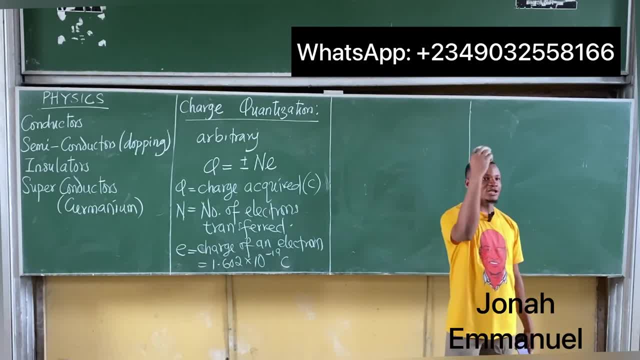 electrons are what they're negatively. electrons are what they're negatively charged. it depends on the one your your charged. it depends on the one your your charged. it depends on the one your your lecture. i use because observe in his lecture. i use because observe in his lecture. i use because observe in his serving. sometimes it isn't positive. 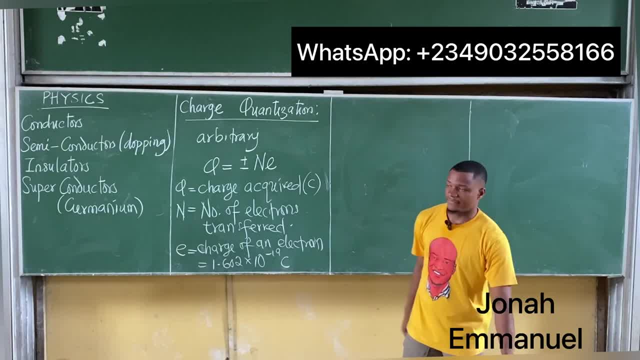 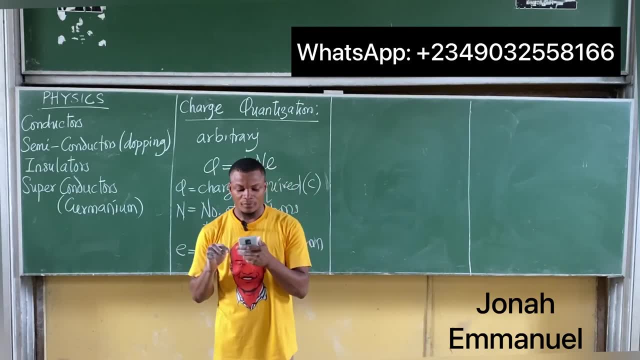 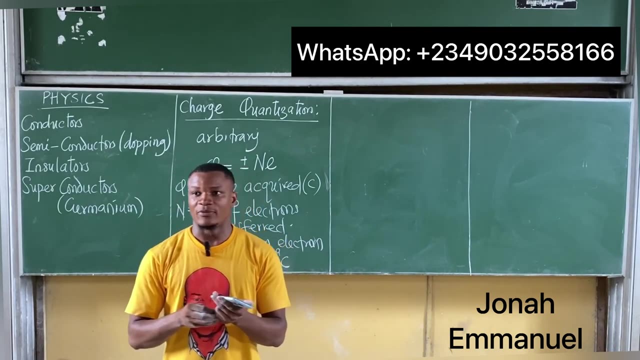 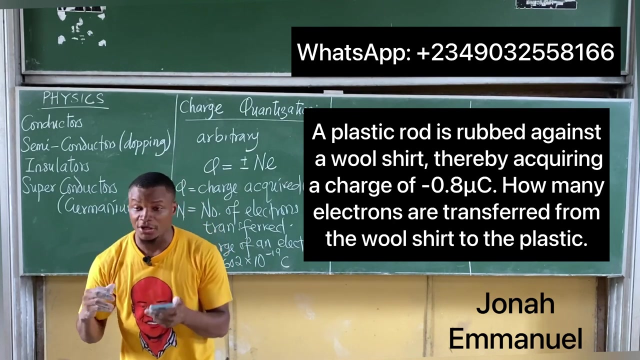 serving sometimes it isn't positive. serving sometimes it isn't positive. example example: please a plastic rod example. example: please a plastic rod. example. example: please a plastic rod. example: a plastic rod is robbed against a plastic rod. is robbed against a plastic rod. is robbed against a plastic rod: r-o-d. 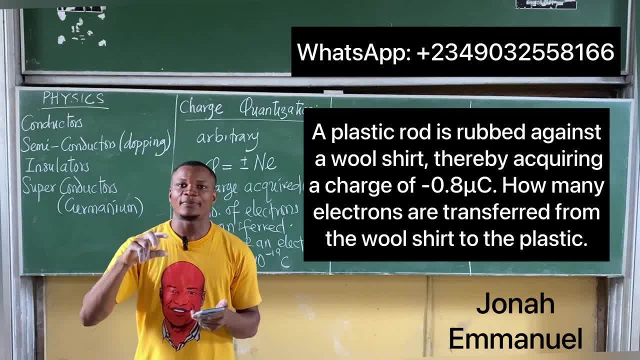 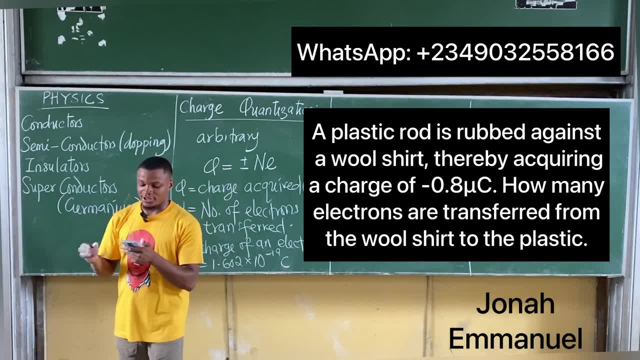 a plastic rod: r-o-d. a plastic rod r-o-d is robbed. r-u-b-b-e-d. a plastic rod is robbed. r-u-b-e-d. a plastic rod is robbed. r-u-b-e-d. a plastic rod is robbed, is robbed. is robbed. a plastic rod is robbed against a. 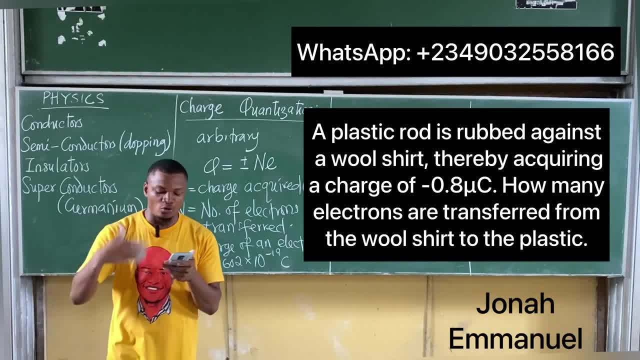 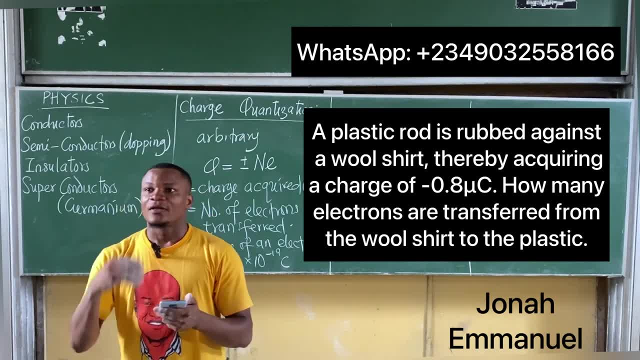 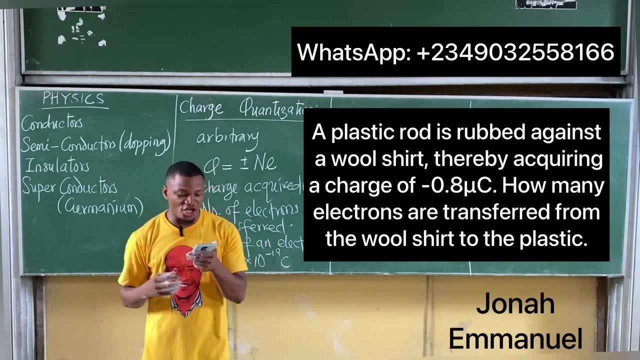 a plastic rod is robbed against a. a plastic rod is robbed against a wheelchair, wheelchair. wheelchair is robbed against a wheelchair is robbed against a wheelchair is robbed against a wheelchair comma. thereby acquiring, thereby acquiring, thereby acquiring a negative hold on, thereby acquiring a a negative hold on, thereby acquiring a. 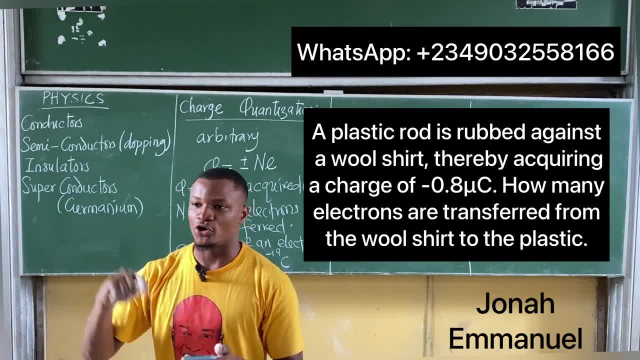 a negative hold on, thereby acquiring a charge of minus 0.8 microcolume. charge of minus 0.8 microcolume. charge of minus 0.8 microcolume. a plastic rod is rubbed against a. a plastic rod is rubbed against a. 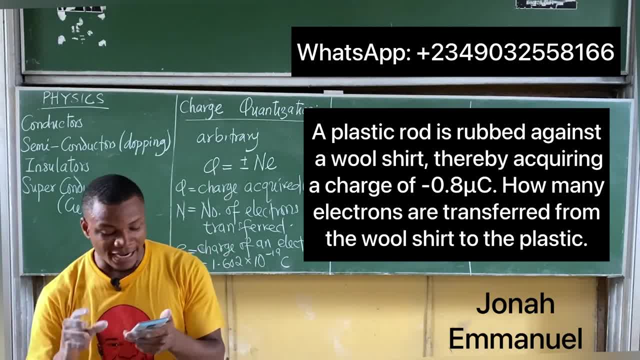 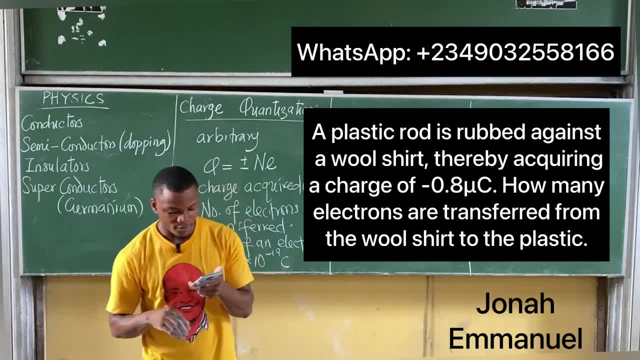 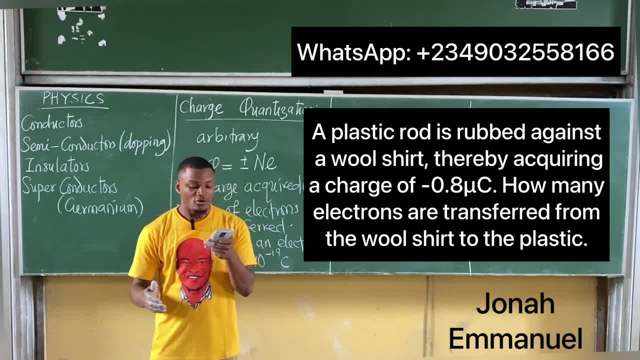 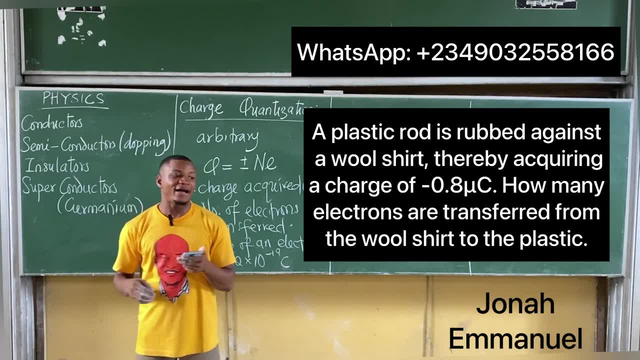 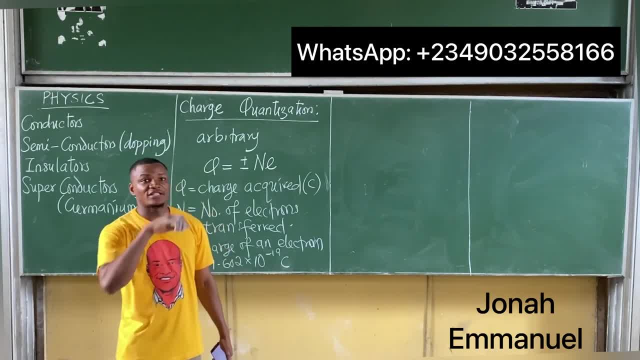 the wheelchair to the plastic, the wheelchair to the plastic. how many electrons are transferred from the? how many electrons are transferred from the? how many electrons are transferred from the wheelchair to the plastic? again I'm wheelchair to the plastic. again I'm wheelchair to the plastic. again I'm saying: a plastic rod is rubbed against a. 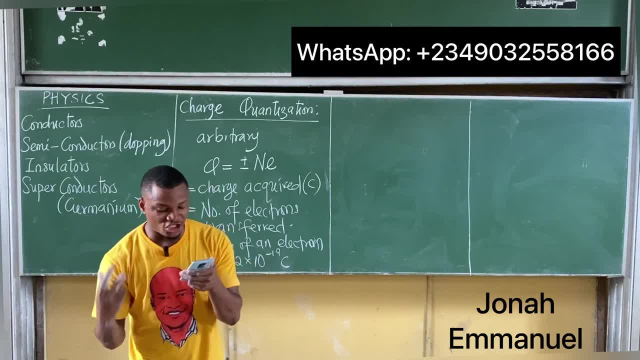 saying a plastic rod is rubbed against a. saying a plastic rod is rubbed against a wheelchair, thereby acquiring a charge of wheelchair. thereby acquiring a charge of wheelchair, thereby acquiring a charge of minus 0.8 microcolume to stop how many. minus 0.8 microcolume to stop how many. 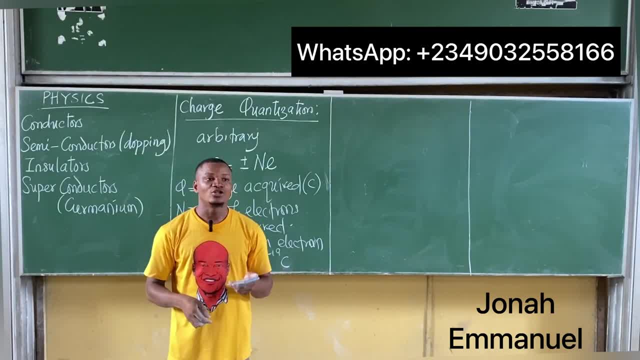 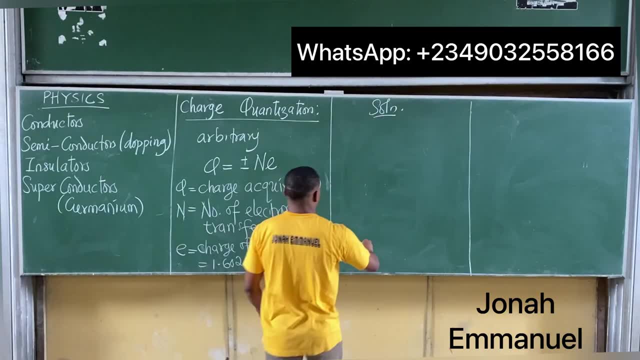 minus 0.8 microcolume to stop how many electrons are transferred from. the electrons are transferred from. the electrons are transferred from the wheelchair to the plastic. who stop so in wheelchair to the plastic? who stop so in wheelchair to the plastic? who stop so in this talk, please? first is first given. 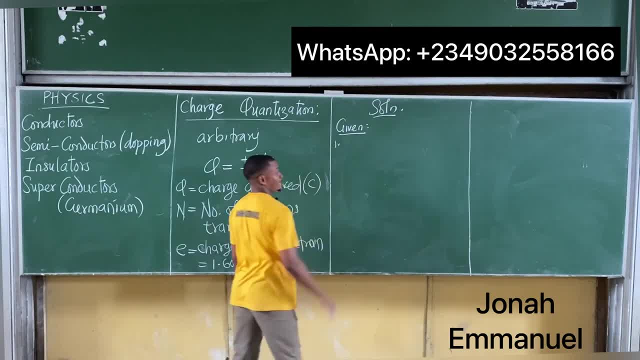 this talk. please first is first given this talk, please first is first given parameters. please check what you're parameters. please check what you're parameters. please check what you're giving there the charge that's Q. so giving there the charge that's Q. so giving there the charge that's Q, so said Q's charge acquired Q: how many? 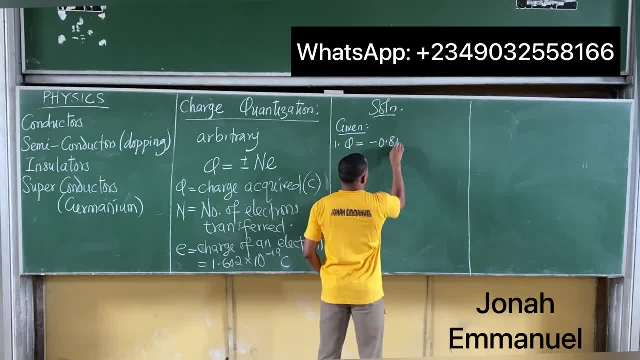 said Q's charge acquired Q. how many? said Q's charge acquired Q. how many? please? all right, please convert this. it, please, all right, please convert this. it, please, all right, please convert this. it becomes minus 0.8 micro becomes or. becomes minus 0.8 micro becomes or. 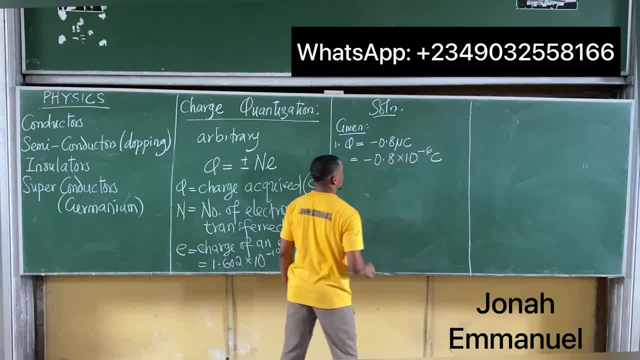 becomes minus 0.8. micro becomes: or there times 10 to power. there minus 6. there times 10 to power. there minus 6. there times 10 to power. there minus 6 volume. what else are you giving that volume? what else are you giving that? 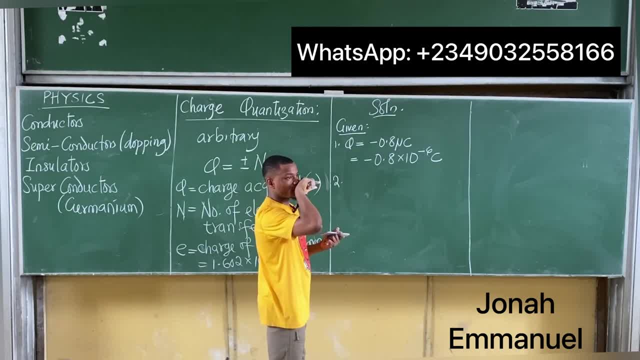 volume. what else are you giving that? okay with you asked to find what number. okay with you asked to find what number. okay with you asked to find what number of electrons. that's n equal to unknown of electrons. that's n equal to unknown of electrons. that's n equal to unknown. you can be given e you may not be given. 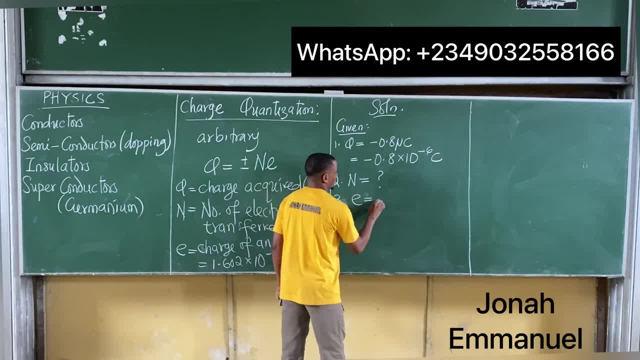 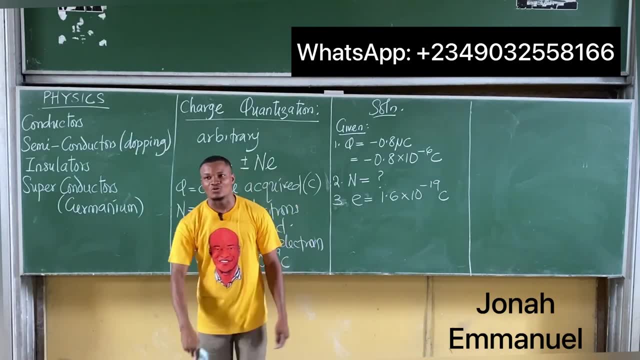 you can be given e you may not be given. you can be given e you may not be given. e is a constant, is equal to order. so I, e is a constant is equal to order. so I e is a constant is equal to order. so I will say 1.6, also 1.6 0, 2 is the same. 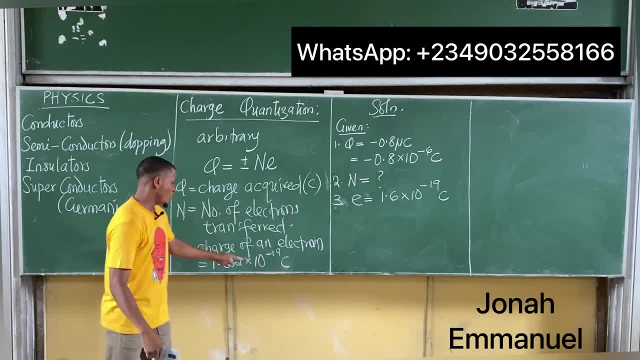 will say 1.6 also 1.6 0 2 is the same, will say 1.6 also 1.6 0 2 is the same thing. approximately right, one point six thing. approximately right, one point six thing, approximately right, one point six, one point six, zero two, the same thing. so 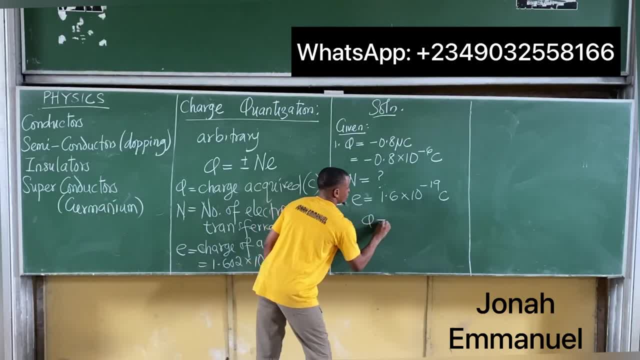 one point six zero two, the same thing. so one point six zero two, the same thing. so from here, obviously we're asked to find, from here, obviously we're asked to find. from here, obviously we're asked to find n. we do that. Q is equal to n, e. so from 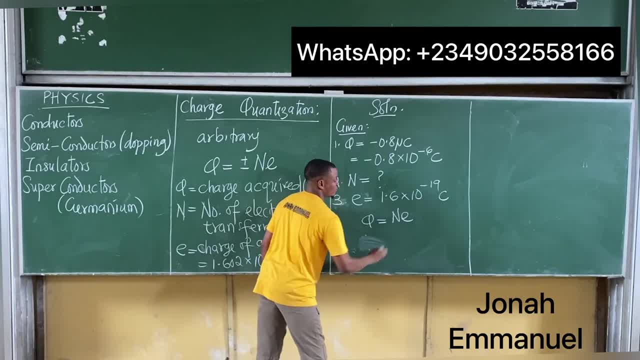 n we do that Q is equal to n e. so from n we do that Q is equal to n e. so from here n will be equal to. of course, my here n will be equal to. of course, my here n will be equal to. of course my task would be to get n divide here by e. 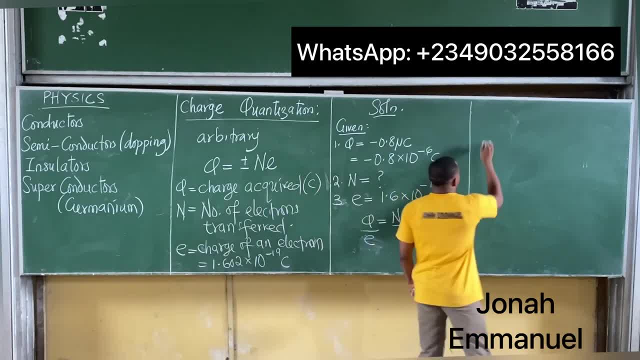 task would be to get n divide here by e. task would be to get n divide here by e. divide here by e. this cancels this. so it divide here by e. this cancels this. so it divide here by e. this cancels this. so it means that number of charges n is equal. 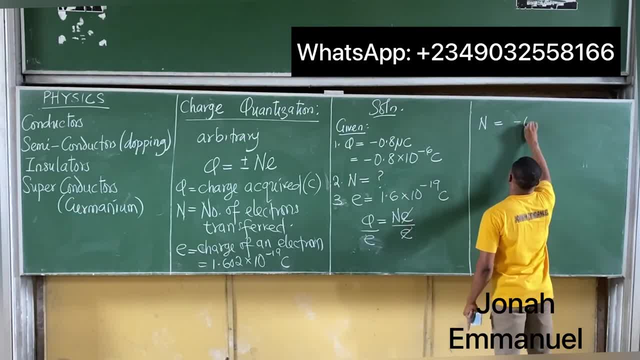 means that number of charges n is equal to Q. does this one here minus 0.8 times to Q? does this one here minus 0.8 times to Q? does this one here minus 0.8 times 10 to power? minus 19? all over e, e is 1.6. 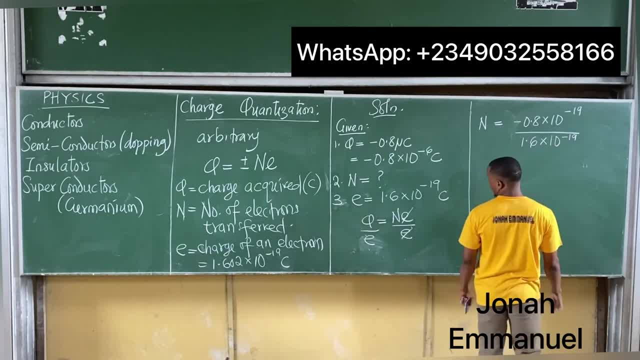 10 to power minus 19 all over e. e is 1.6. 10 to power minus 19 all over e. e is 1.6 times 10 to power minus 19, please minus times 10 to power minus 19, please minus. 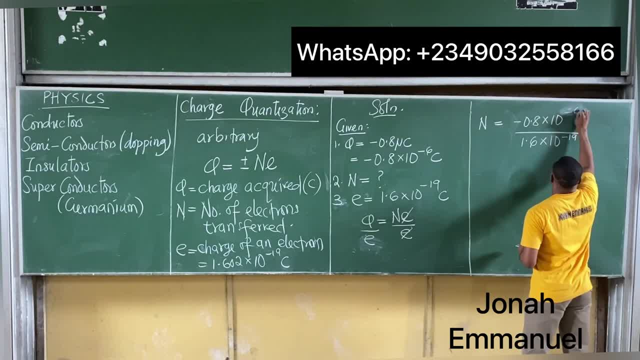 times 10 to power: minus 19, please, minus 6, please sorry, minus 6, and then minus 19. 6, please sorry, minus 6, and then minus 19. 6, please sorry, minus 6 and then minus 19. now look up it. look up, okay, fine, don't. 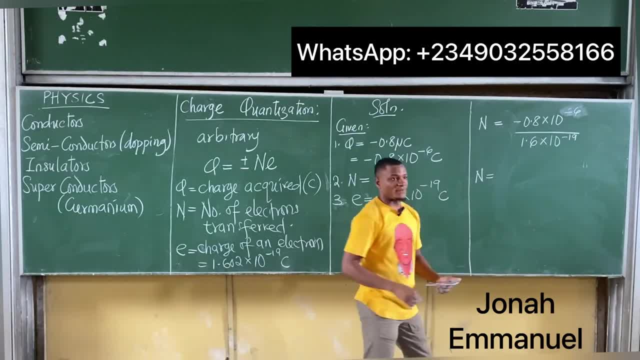 now look up it. look up, okay, fine. don't now look up it, look up, okay, fine. don't worry. give me values. what's n here, worry. give me values. what's n here, worry. give me values. what's n here, please punch correctly, please give me. please punch correctly, please give me. 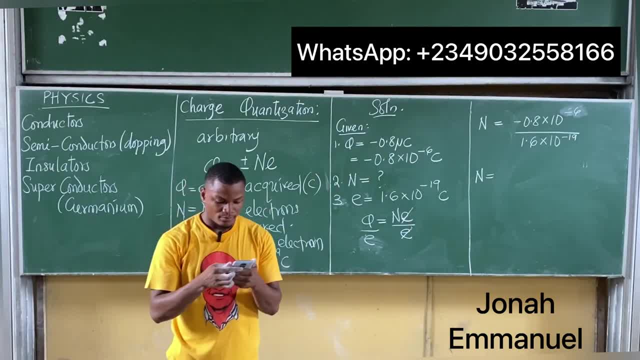 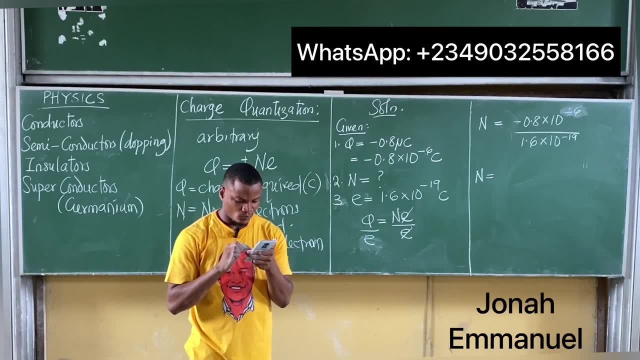 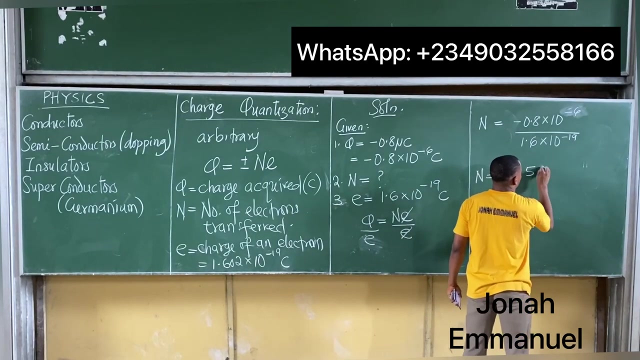 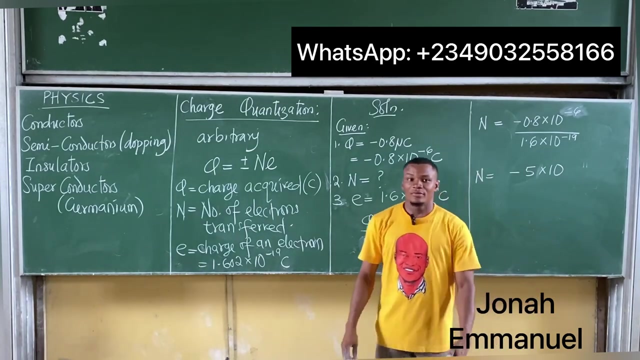 please punch correctly. please give me value. what's n, please, all right, all right, all right. Minus 5 times to power what there Plus or minus 12.. Now listen, Listen, please, Listen, Listen, Listen, Listen. Get this concept. Look up, please. 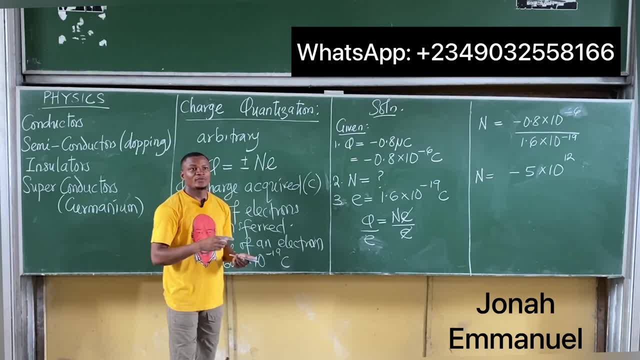 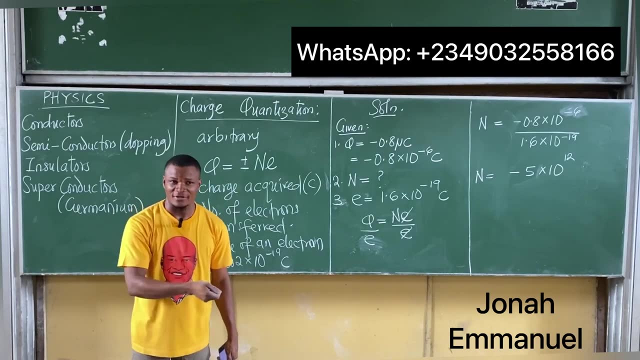 I want to tweak something. So look up, Get the concept, please See. In my formula for charge quantization I have a plus or minus. This plus or minus depends on your usage. Sometimes you use negative, Sometimes you use positive. How Look at this, please? 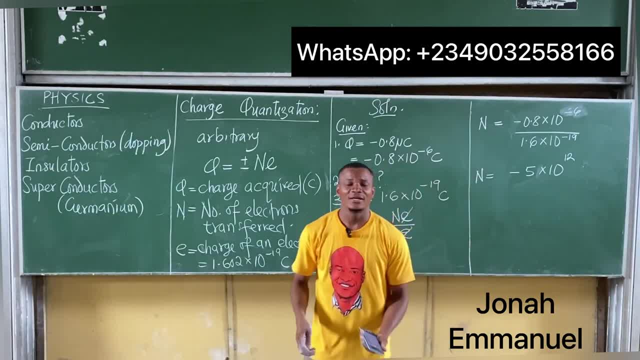 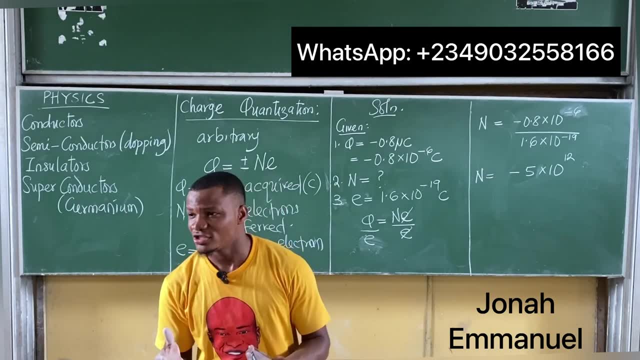 This stuff is asking you how many elections were transferred. Some things cannot just be negative in life. Some things cannot be negative. Example: Age Age cannot be negative. How old are you? I am minus 20 years old Makes no sense. 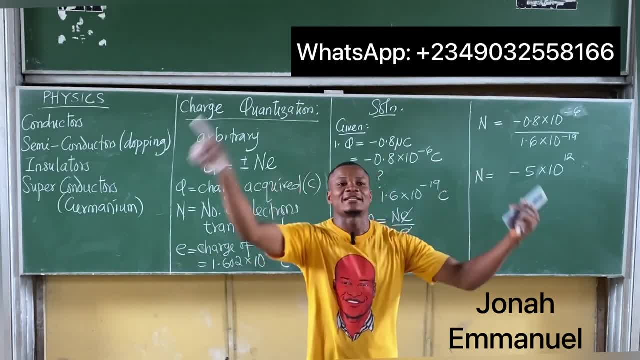 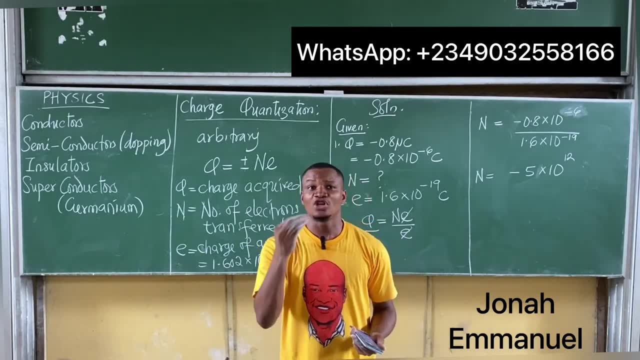 I walk into this class and I say how many boys are in this class, Or I just say what is the number of boys in this class, And they tell me minus 15 boys. It makes no sense. In other words, I am saying this: 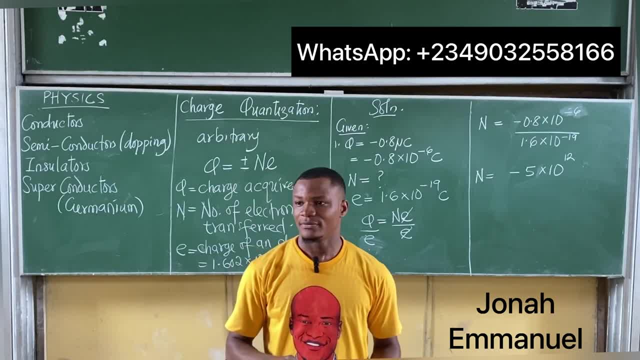 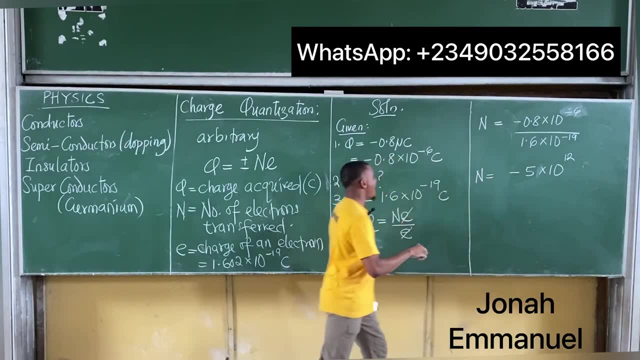 Number of something cannot be negative. In other words, in this case, now observe that the number is negative. This is not possible. So what do I do now? I will now play with this formula, This one here: Plus or minus. 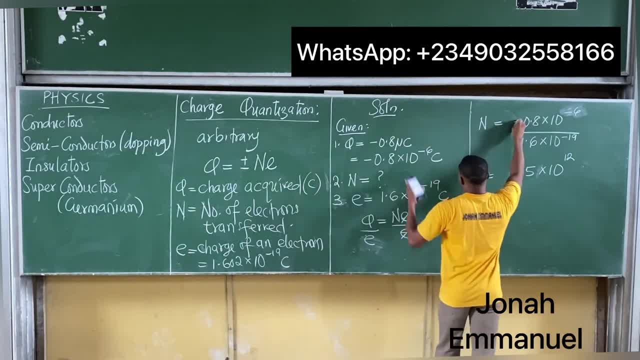 Means for me to make this one positive here. this one here which is negative, must be divided by what there and not that negative. It becomes negative. negative gives you positive. This becomes the answer. So, please, you play with the plus or minus at your own. 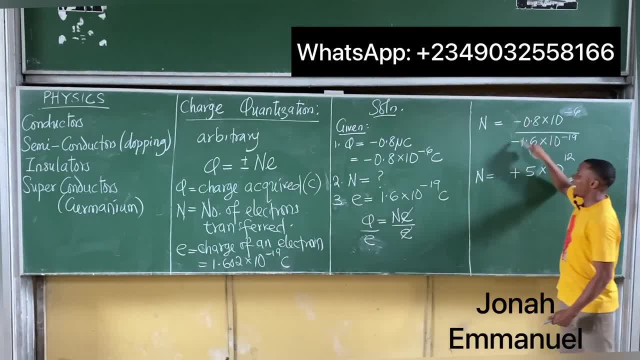 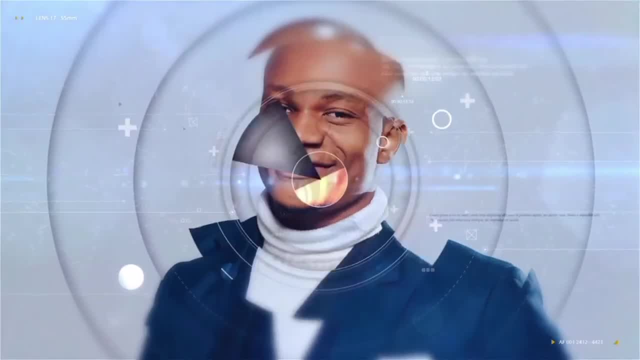 terms. In other words, if this was a positive number, I don't have to put negative again. That's the idea. So that's it, Thank you.